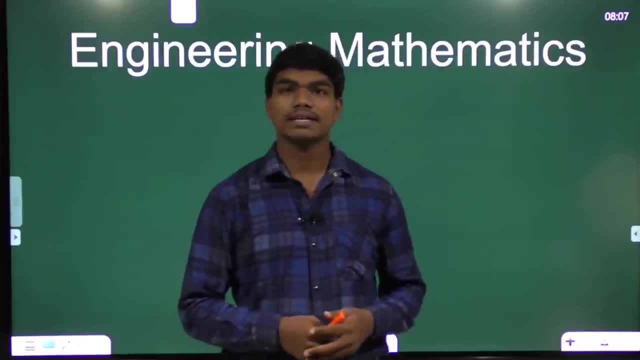 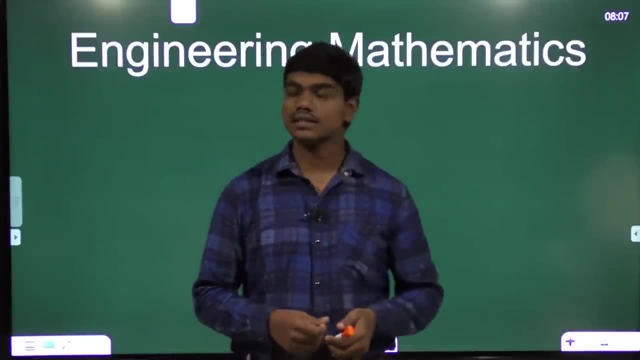 So I welcome you all to this first session on engineering mathematics. As some of you know, my name is Vinay Kumar and I am from IIT Madras. So, coming to the course, this course at the very outset, this engineering mathematics course. 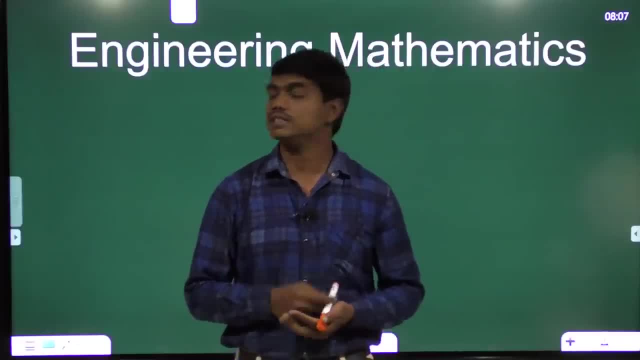 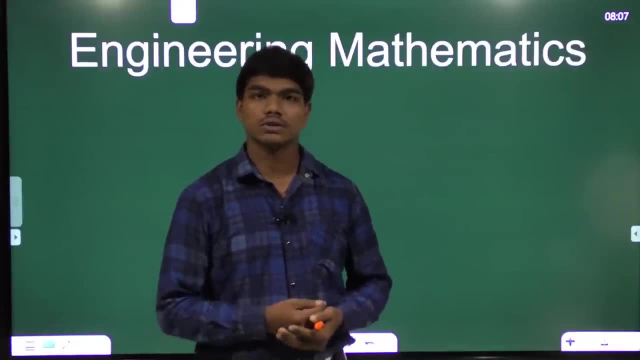 deals with the basic concepts, The basic concepts of mathematics that we use in engineering. Now, before going to the course contents, I would like to give some overview of this course to you. Like I would like to introduce this course to you. 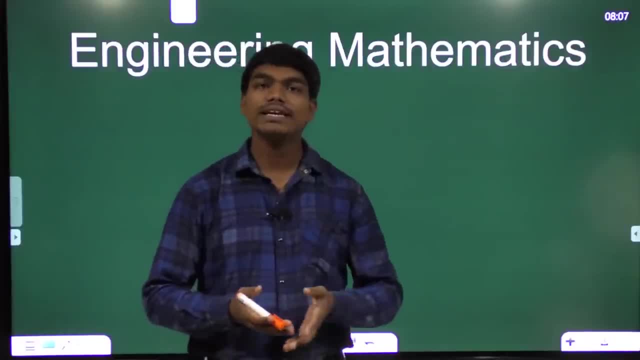 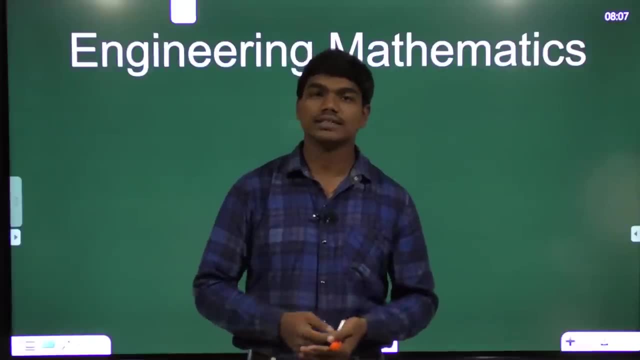 And, as you know, this mathematics is not a new course to you. You have been dealing it from your school, For example, every one of us, right from the shopkeeper dealing with the simple calculations to the engineers and scientists that deals with scientific calculations, every one of. 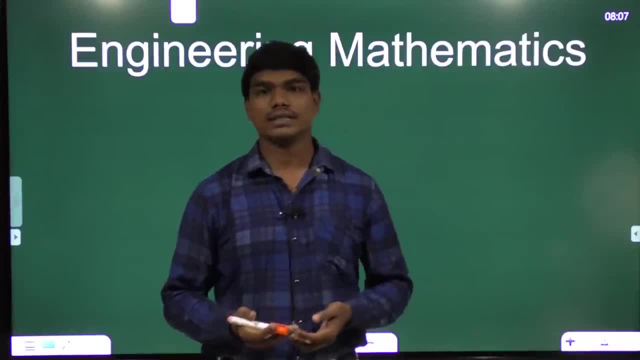 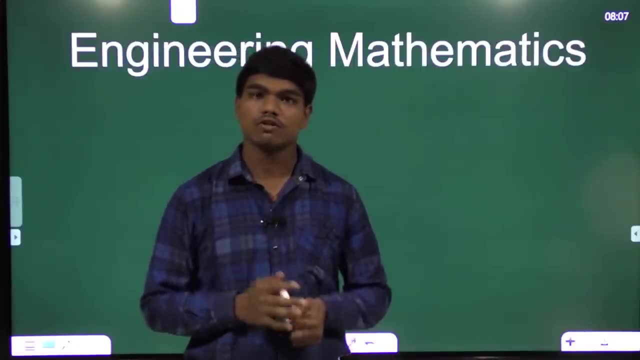 us is in need with mathematics at some point And we have been doing that since our schooling. So, coming to this engineering mathematics course, In this course we dedicate in learning to engineering concepts of mathematics. we learn a few fundamental themes, fundamental concepts of engineering mathematics that we apply in 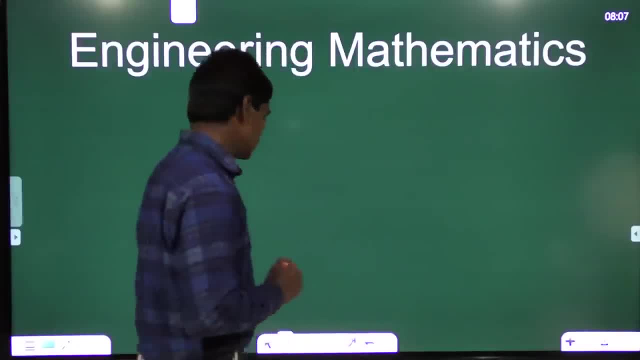 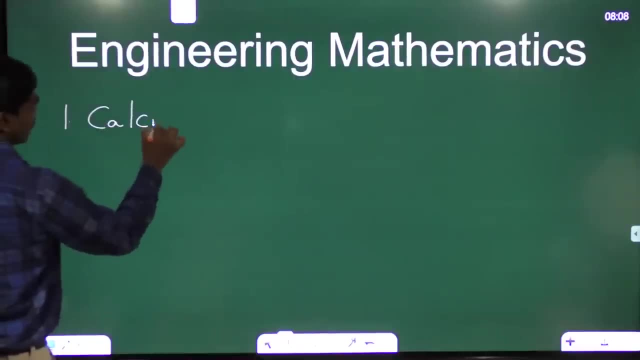 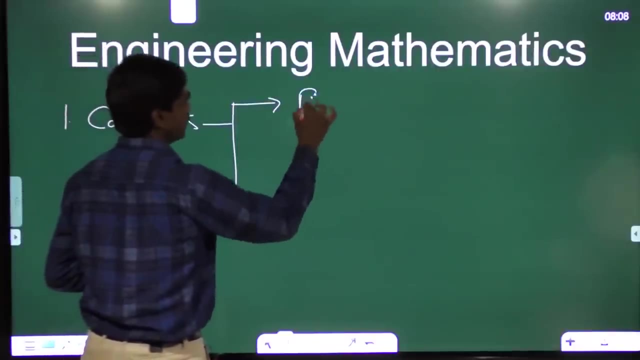 real time science. So, coming to the course, contents of this course, if you would like to see, we divide this course into certain modules. The first module is calculus. Now, in this calculus we again subdivide the topics as basic calculus, basic math and 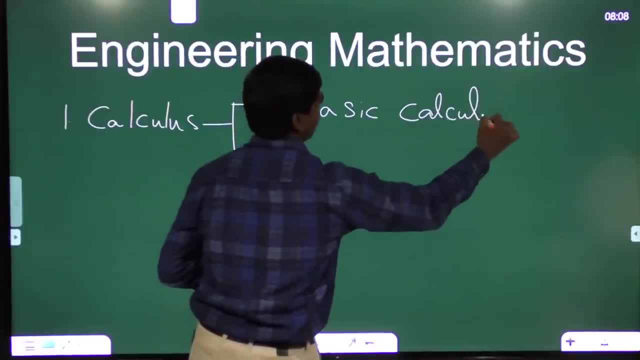 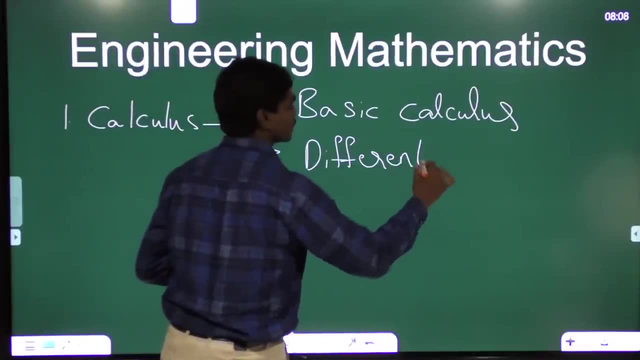 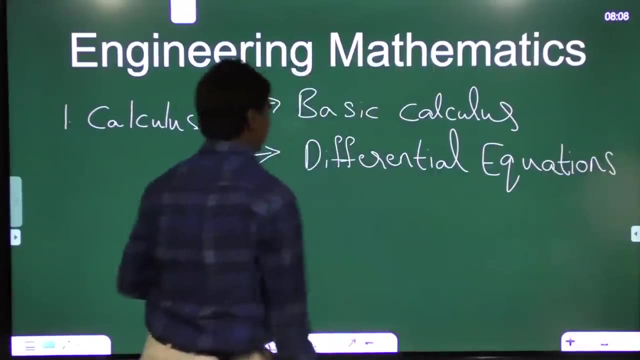 basic algebra And then we go for differential equations. Once if you come up with some calculus, we go for differential equations. And then we go a bit more and we deal with vectors and where we go for some vector calculus And then 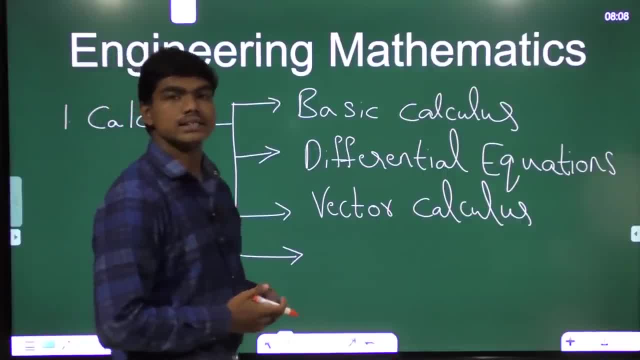 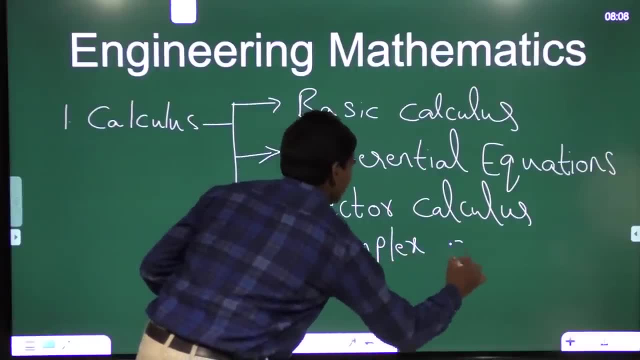 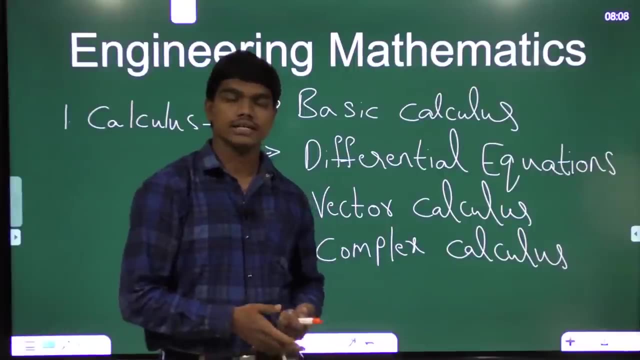 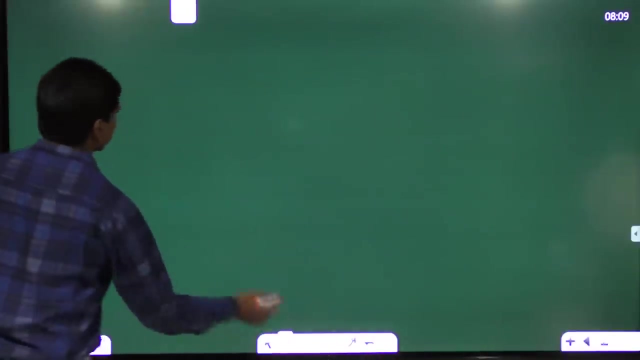 We deal with complex vector, complex variables and the integration and differentiation of complex numbers or complex functions. so which is complex calculus, and you know this calculus is the major portion of our course of study in this particular course. and now, continuing with the second module, in the second module we cover linear algebra, which basically involves matrices. 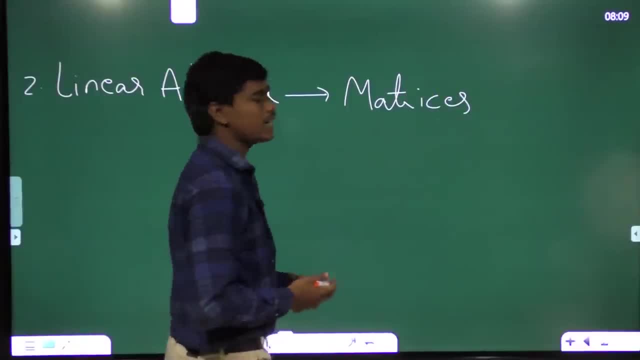 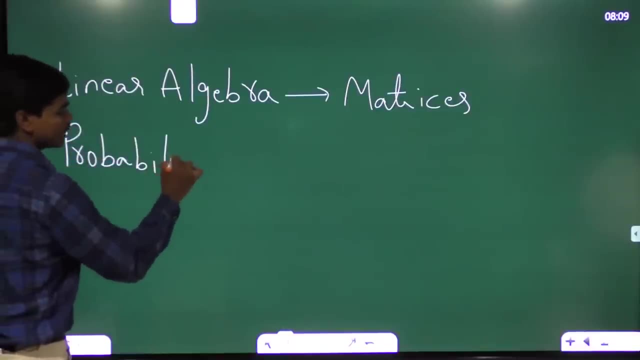 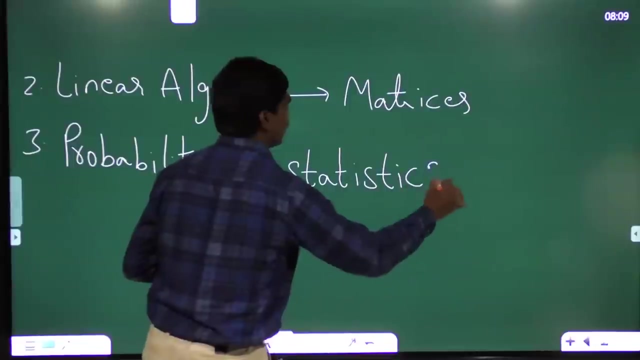 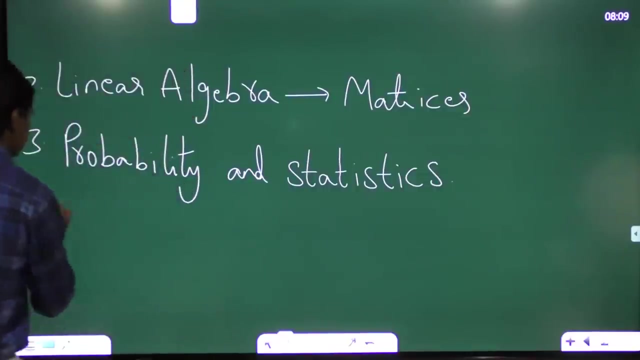 and several functions associated with matrices that we do in real time. next we go for probability and statistics, which some of you are asking in the comment box: probability and statistics: probability and statistics, where you will be knowing, with different terms of probability and different data analyzation techniques in analyzing statistics. and then we go for numerical methods: module. 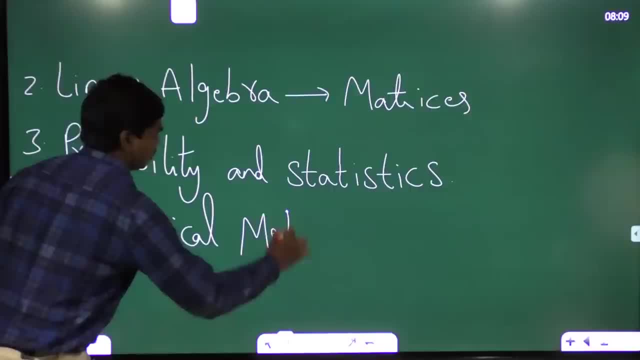 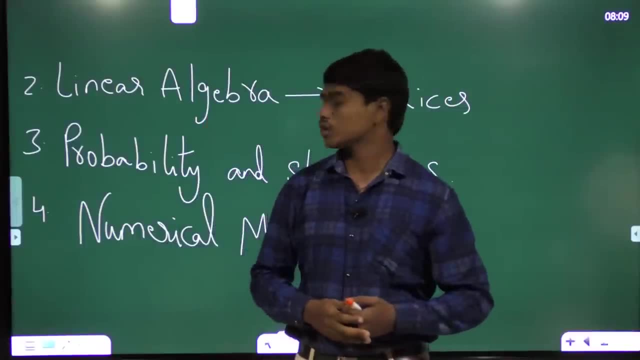 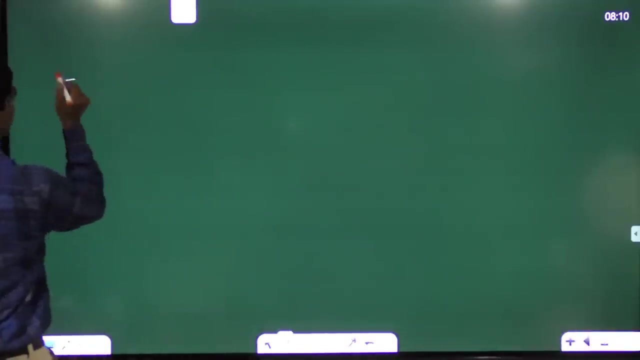 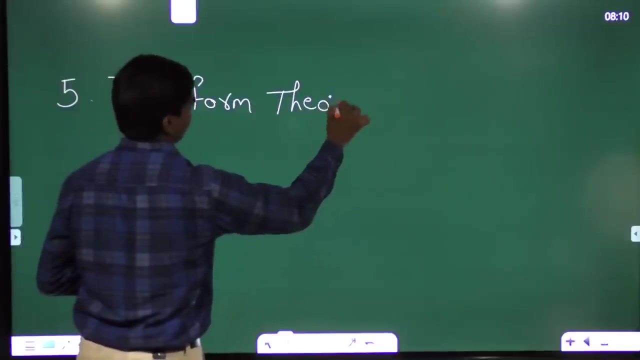 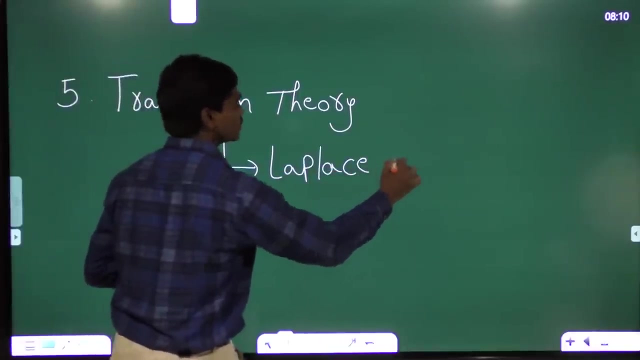 where in this module we see solving different. i mean we learn different techniques about solving of non-algebraic equations and all these things. and next, coming to the fifth module, we go for transform theory, where we'll be looking at certain laplace transforms which are really important when you're dealing control systems: laplace transforms. 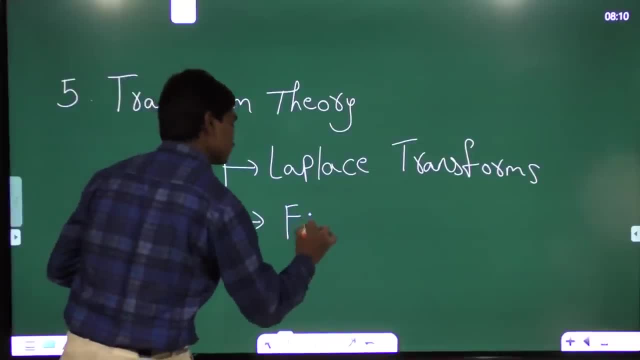 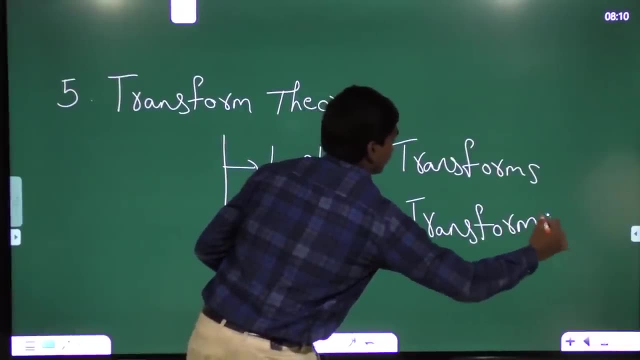 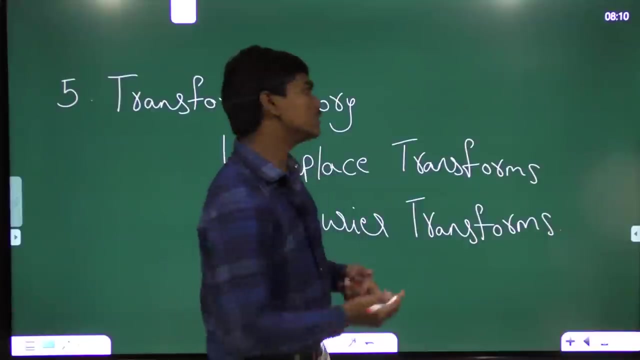 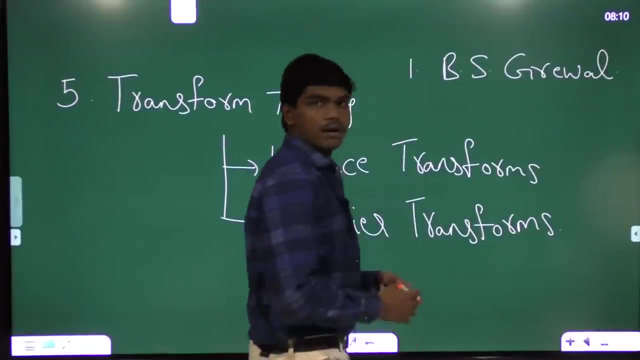 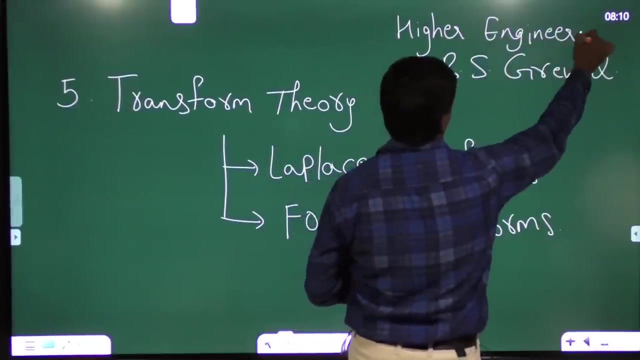 and now we'll go for four-year transforms as well, and, after the completion of this laplace, transforms you can doeslyn. so the ones you were interested in, do you find it worth theense? you as well? oh, go ahead. Gaurav desri group- Yeah. 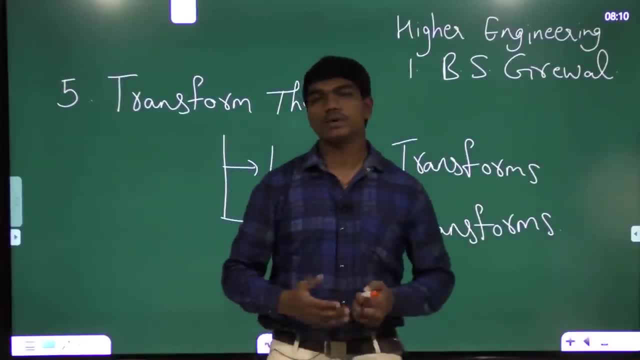 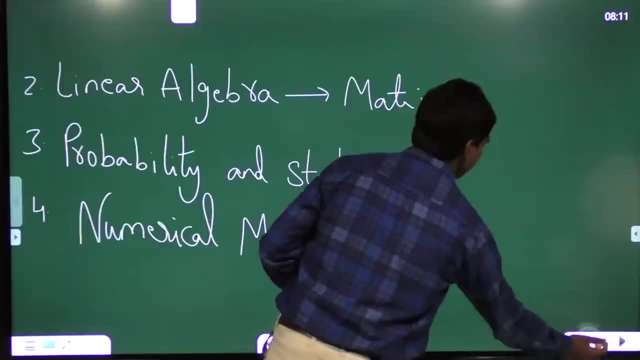 Now I'm going to leave this here for a second now, after attending these lectures, book reading problems. so, going back to our discussion, so these are different modules that we are going to cover, typically classified into six modules which we take on over the course of this course. 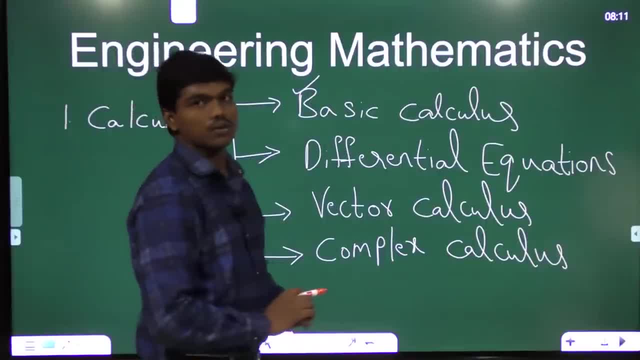 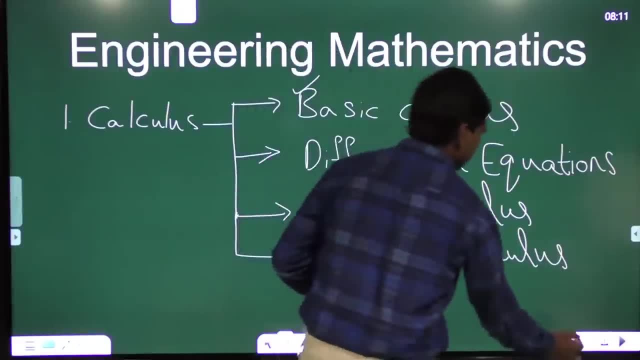 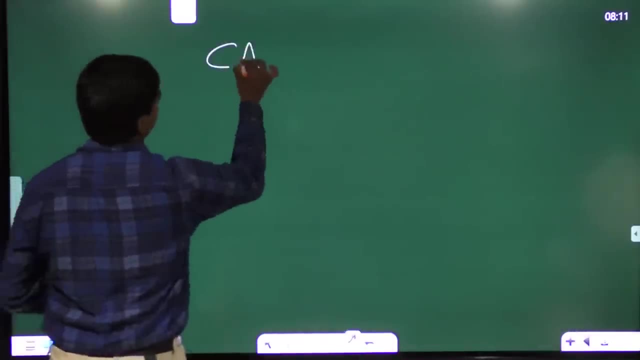 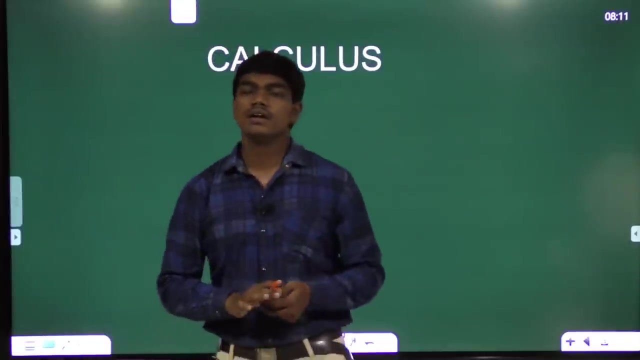 first we'll start with calculus and we'll start in that with basic calculus. now, why this basic calculus, or why calculus is really important for us? we'll start seeing that. so we'll start our first chapter today, which is calculus. so you can look at, look here. now we'll start with basic calculus and before starting, 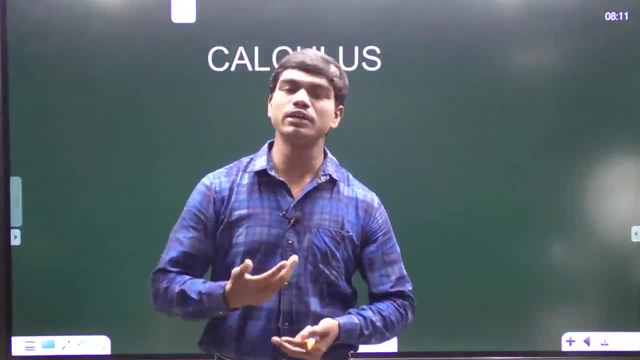 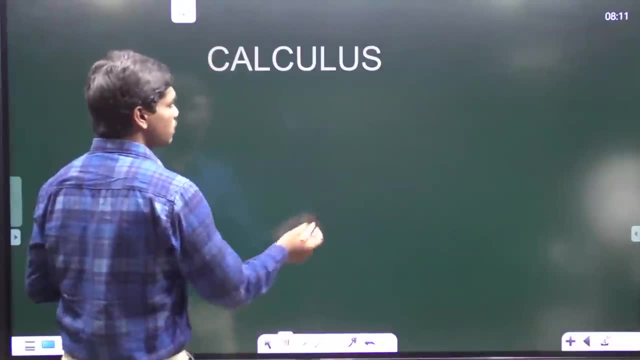 basic calculus. we'll look after the need for learning calculus, why we need to learn calculus. what happens if we don't learn calculus? if you might have gone to your 12th standard or diploma course in there you'll be seeing a lot of expressions, especially if you have a mechanical 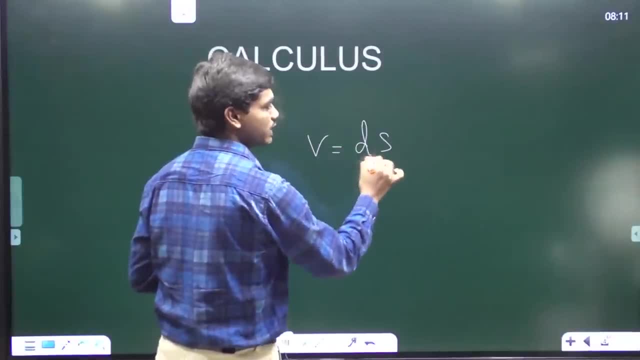 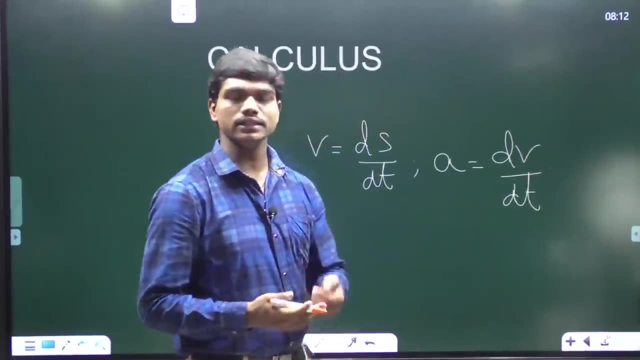 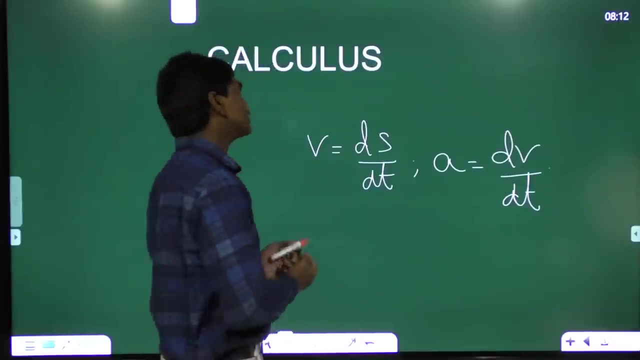 you'll be seeing the definitions like: velocity is the rate of change of displacement, the acceleration is again rate of change of velocity, all these things but means in your life you'll as an engineer, in your life you'll be dealing with some differentiation techniques, some integration techniques as well. okay, so for that we need to have knowledge of. 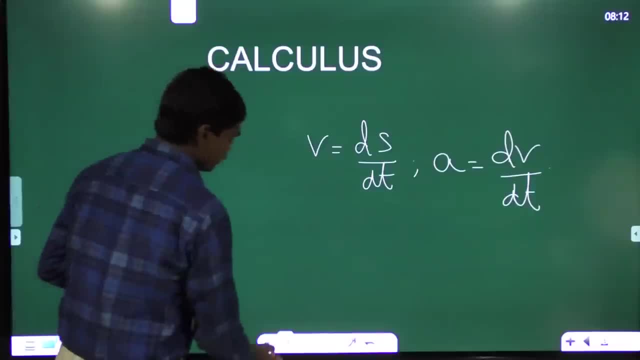 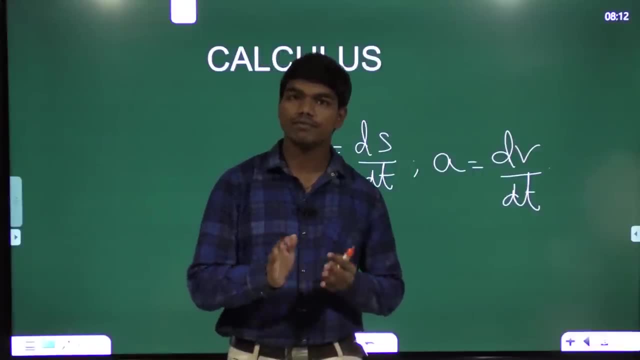 some basic calculus here. so right now, before starting calculus, i don't expect that you have any prior knowledge in mathematics. we'll start right away from the scratch. so if no one has, i mean if someone don't have any knowledge about this, you please don't feel we'll be covering that. 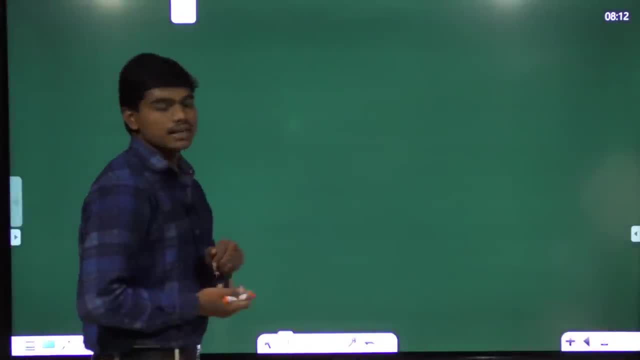 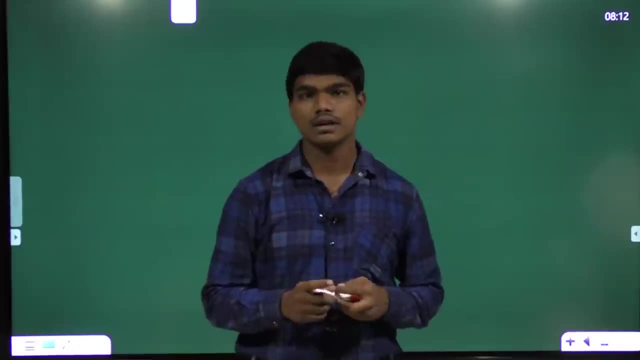 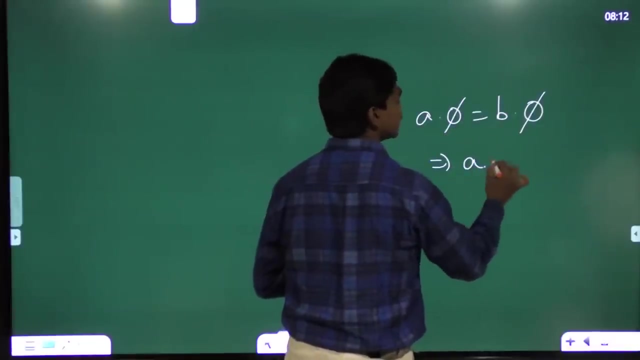 from basic itself. okay, so now let's talk about the question of calculus, starting from calculus. now, before starting calculus, let me ask you one question: can we cancel two zeros anywhere, like, for example, if i write a into zero is equal to b into zero, can i cancel these two zeros and can i write a is equal to b? 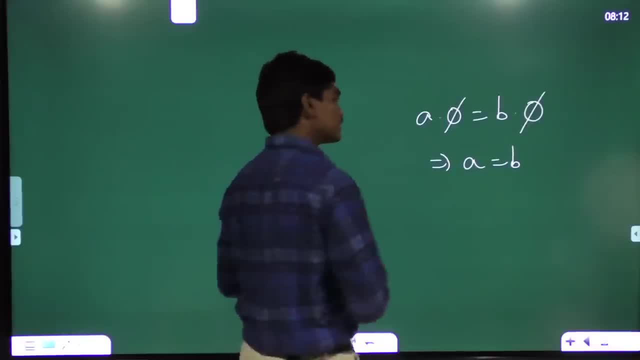 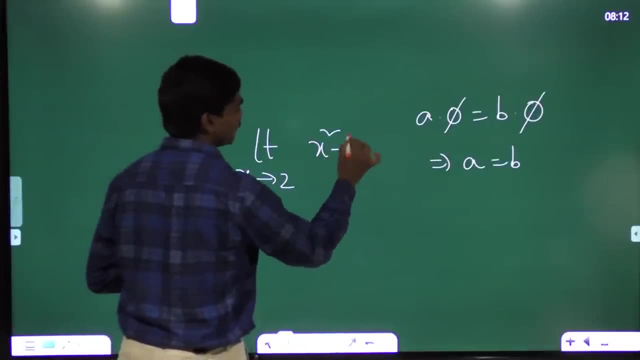 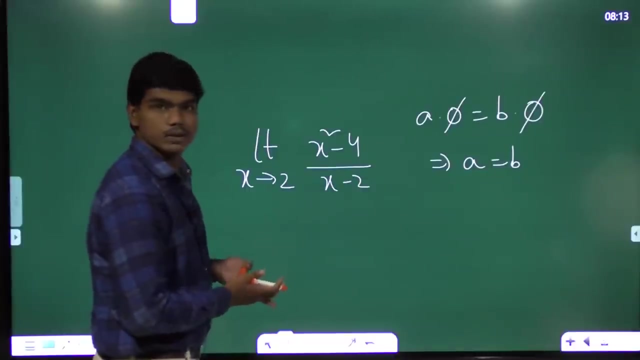 can we do that? i hope many of you know we can't do that correct now. why then? you might have gone through some limits like this in your schooling, for example, x square minus four by x minus two limit. basically, you might have dealt it in your first interval, I mean 10 plus 1, or in 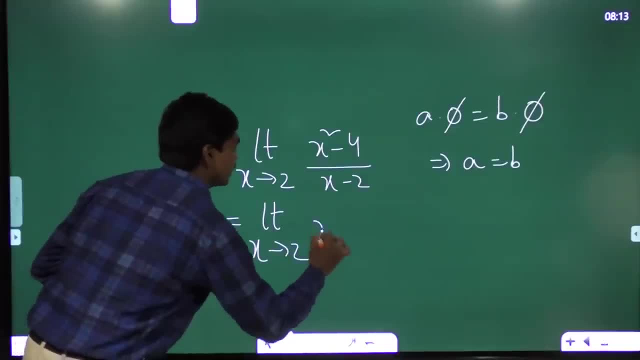 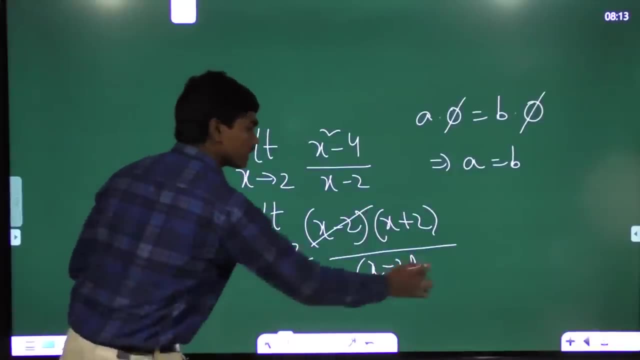 the 10th class itself. then you will simplify this in this way: You will factor this as x minus 2 into x plus 2 and divide it with x minus 2.. And if you remember, here you are supposed to cancel, here okay, Which means when you can't cancel two 0s, but still you. 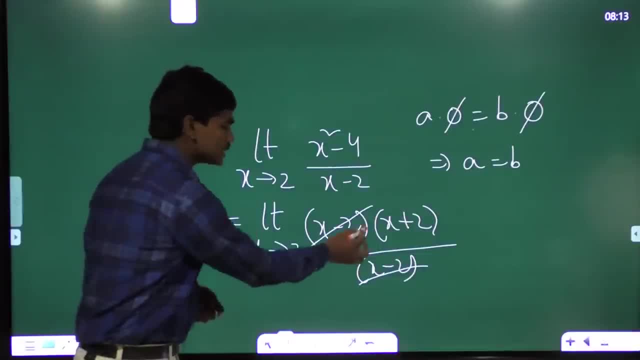 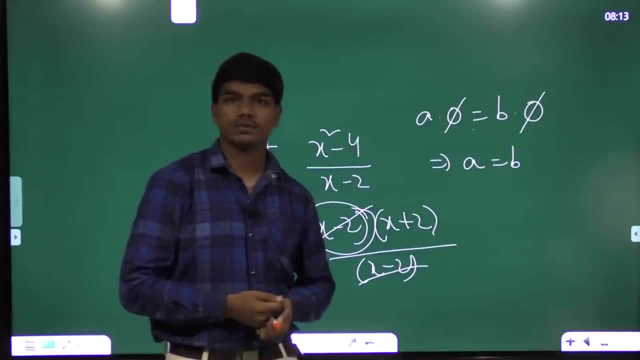 are cancelling this x minus 2,. one thing is very clear for you: this x minus 2 is not a 0 here. okay, So if x minus 2 is not a 0, then what is this x minus 2?? So this is the. 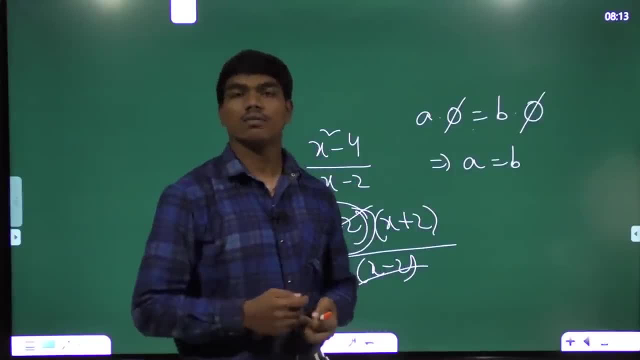 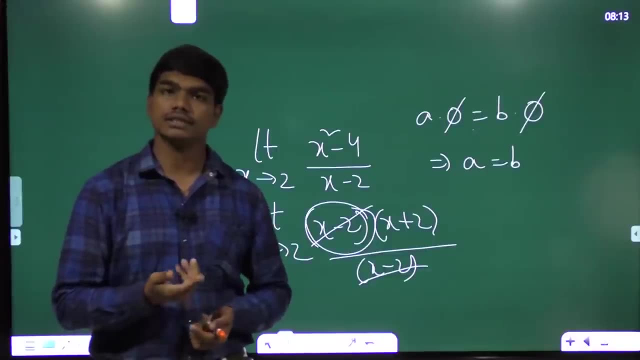 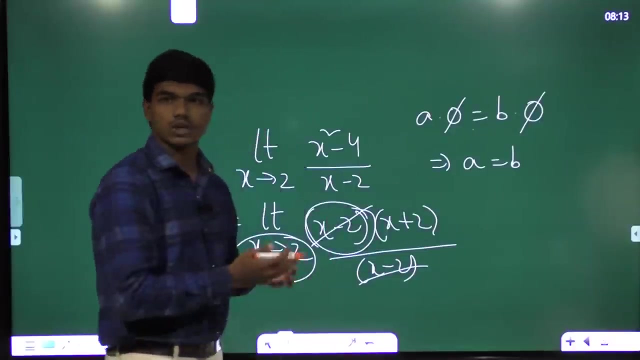 starting step for solving, I mean for starting calculus, And once we have clear idea on the concepts of calculus we will go for some advanced calculus, basically trying to solve some differential equations and all these things. So the difference between this tends to 2 and cancelling. these 0s will short out in a few minutes. So starting there, 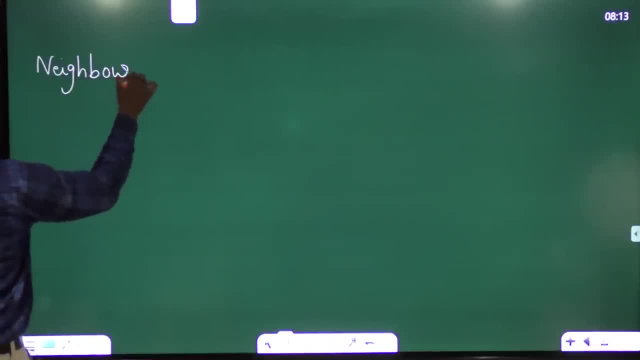 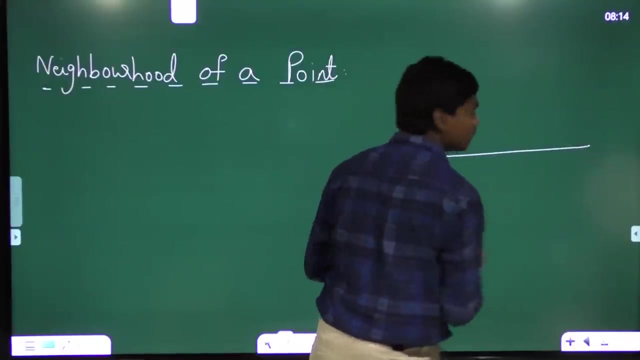 I would like to give you the definition of neighborhood of a point. Neighborhood of a point, Now, what is this neighborhood of a point really? Now, for example, let us suppose this is a main node in front of your home and, for example, this is somewhere here. 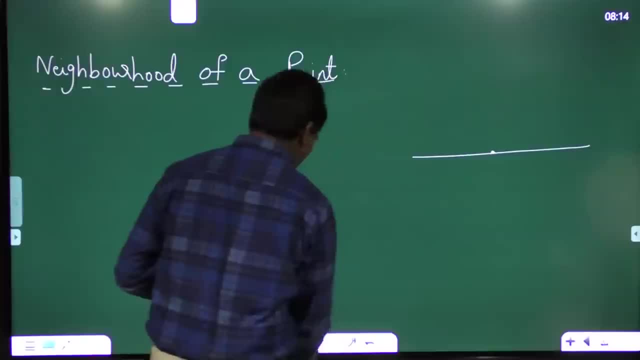 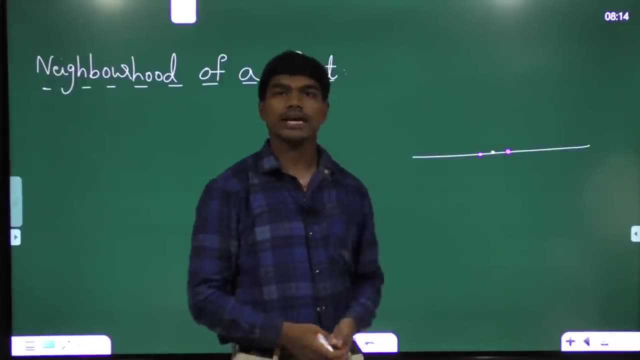 is your home. okay, Now, if this is your home, then tell me one thing: Who are these neighbors? These people call to you. Of course they are your neighbors, correct? Similarly, the persons who are here are also neighbors, But someone who is far away from your home, if 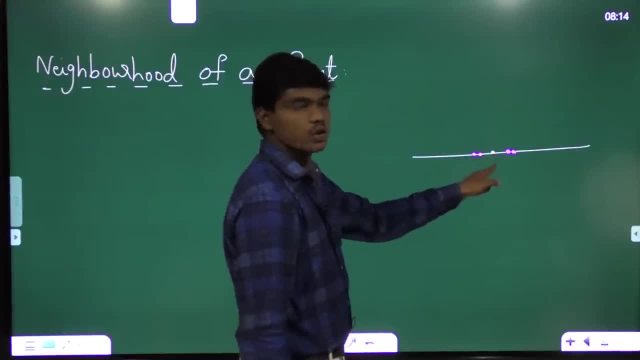 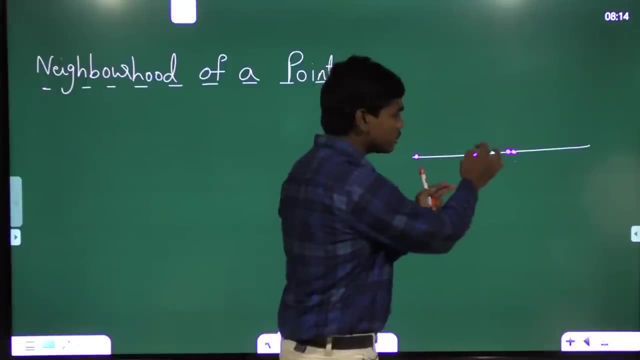 this is your home. this black dot which I am putting or this white dot which I am putting is your home. then someone who is far away is not your neighbor, which means you confine yourself to some space around your home so that you declare them as your neighbors. Similarly, 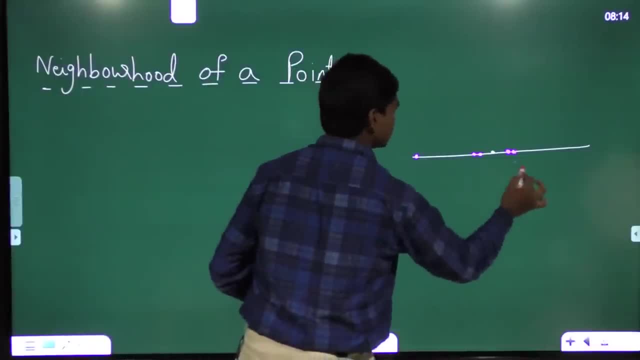 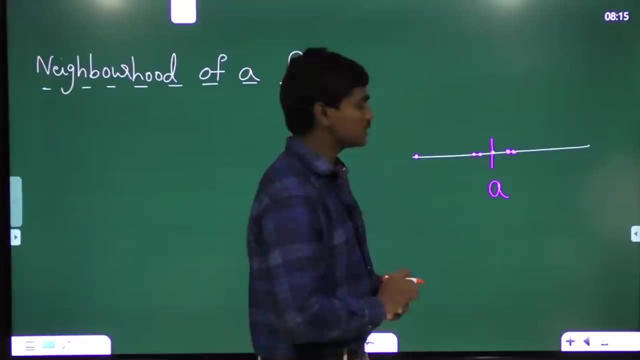 on a real plane. let me clear these points: design access. Okay, So let us get back. So, if this is the point A, on a real number axis, and you know definitely there are infinitely many real numbers between A to successive real 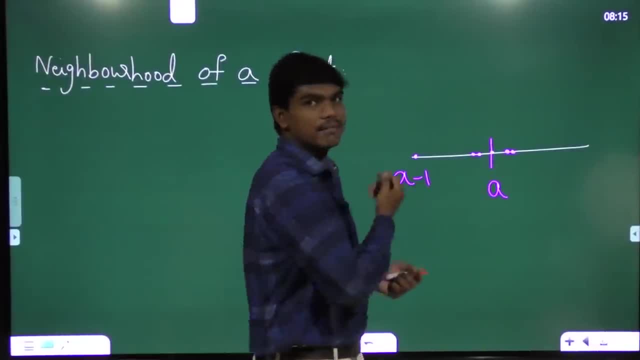 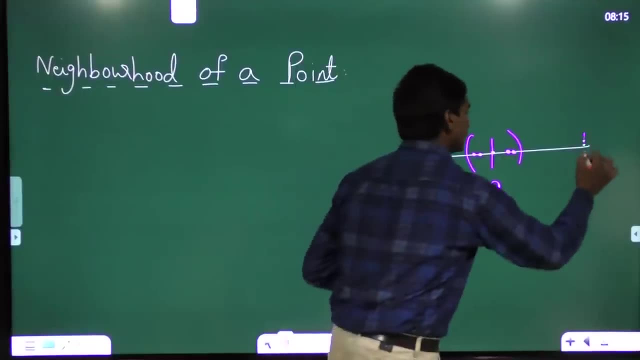 numbers. That means there are infinitely real numbers between A and A minus 1.. In this case there are some real numbers which are very close to this. A correct: A plus 1 is also so far from A and A minus 1 is also so far from A. But if you see, there are some real. 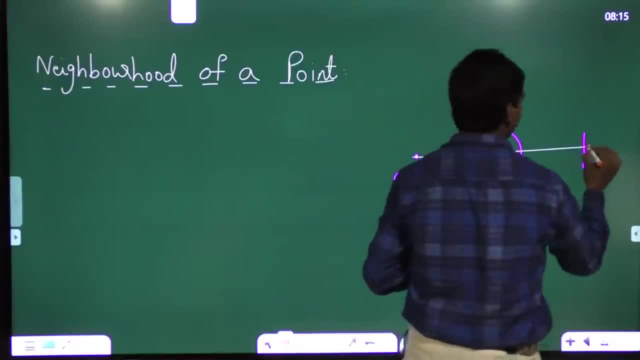 numbers which are very close to this A, very close to A Now, for example, if I consider this as my x-axis, if I consider this as my 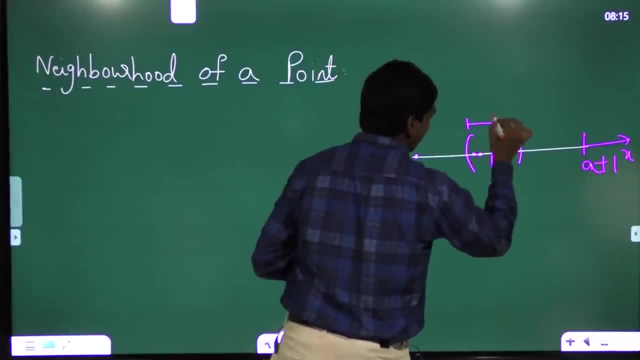 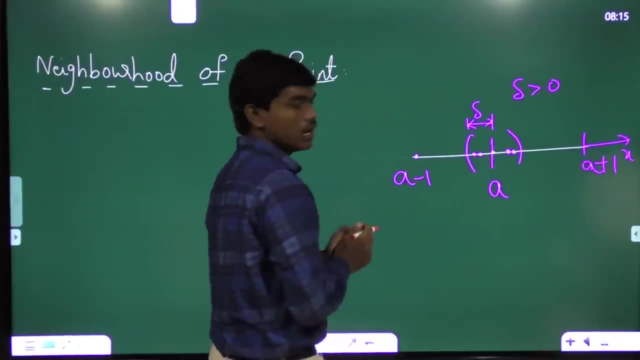 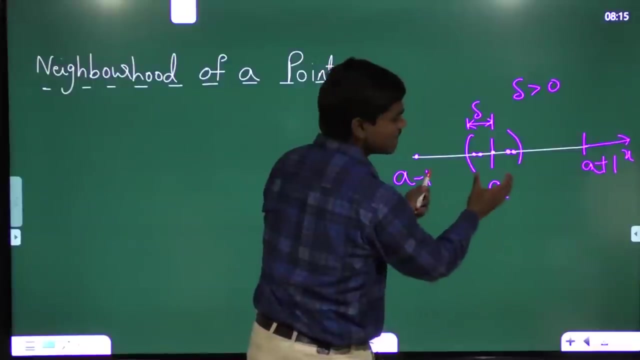 x-axis, then- and let me call this small difference here as delta, where delta is positive and of course delta is very small, Then if this is x-axis having origin at some other point- we don't care right now- then there are some values of x which are lying very close to. 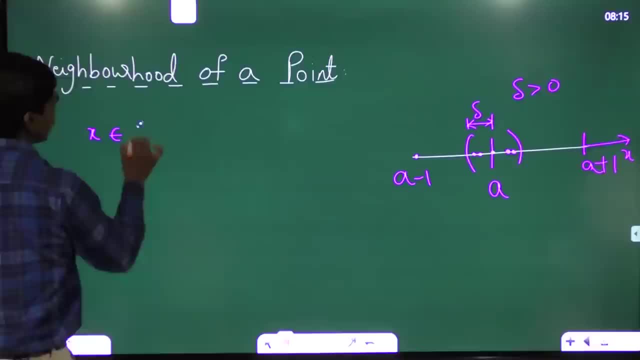 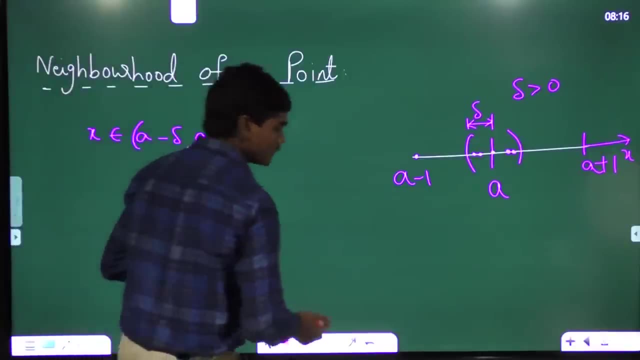 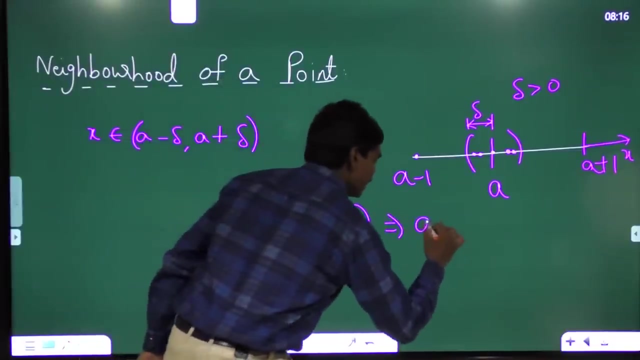 x. And can I write that x belongs to A minus delta comma A plus delta? for that It's on open interval. And if you don't have any knowledge on open intervals you can look here. For example, if I write x belongs to A comma B, then this implies A is less than x is less. 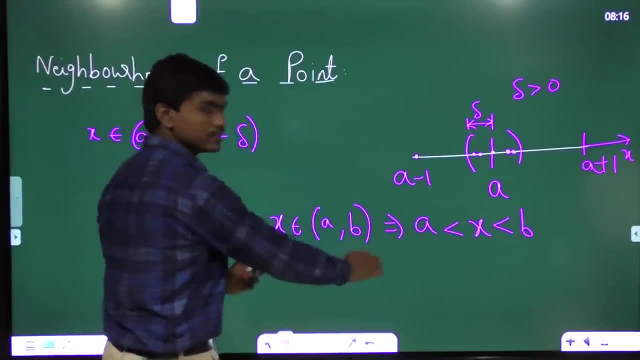 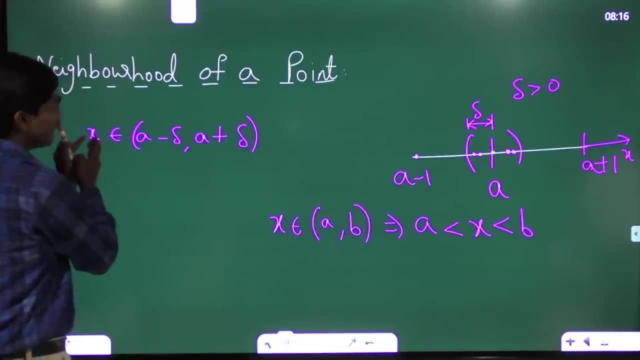 than B means x is basically in between A and B. If I have a closer base here, then you might have put equal to sign here. So, keeping this in mind, so this is the neighborhood of A, which means These values of x are very close to A, and so these are called neighbors of A, So which? 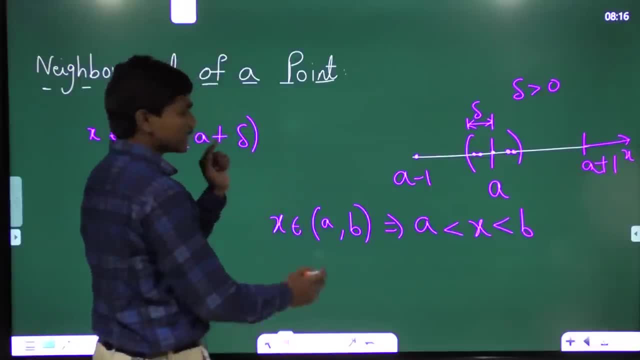 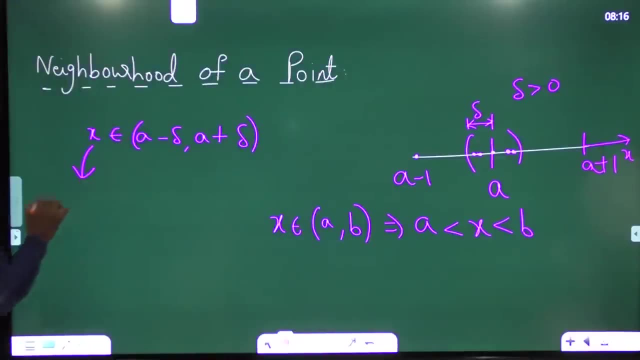 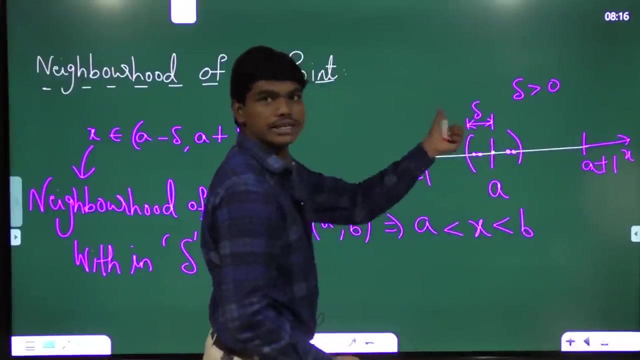 means your limit which you are talking, your x tends to A means x is lying in the neighborhood of A, but not at x is equal to A. So this interval is neighborhood of A within delta limits. If you change this delta, this interval incases or decases, depending upon your incasing or. 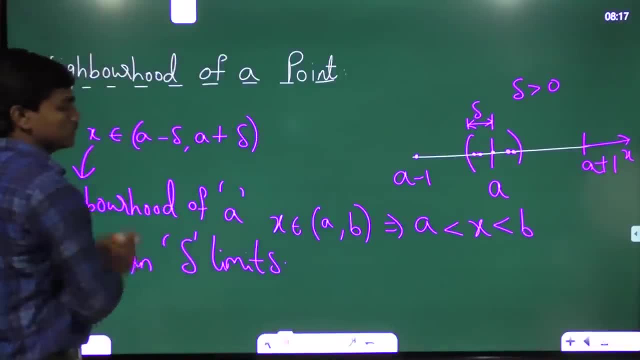 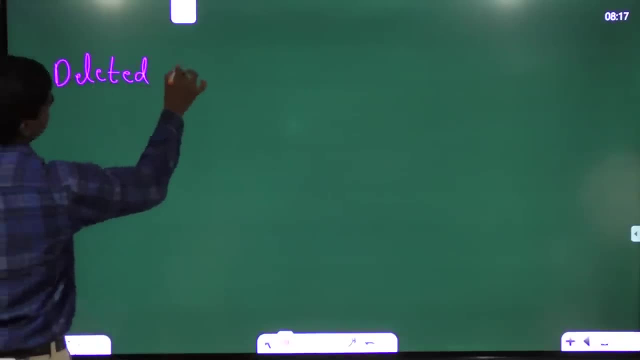 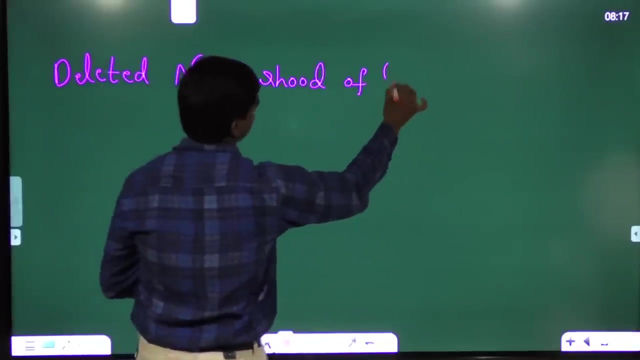 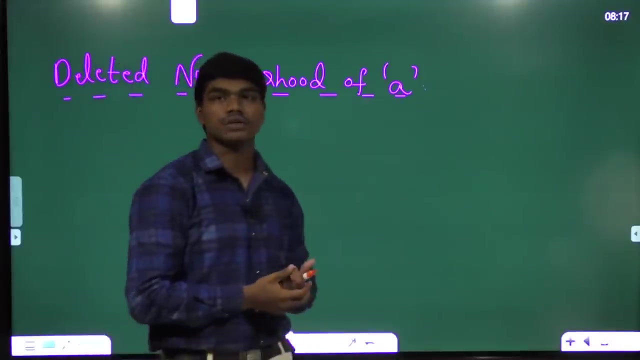 decasing this delta. So this is the case with neighborhood. Now we'll consider one more thing, which is called deleted neighborhood of A. Deleted neighborhood of A, As the name suggests. Deleted neighborhood of A. As the name suggests, There is the word deleted before neighborhood, which means we are deleting some part of the. 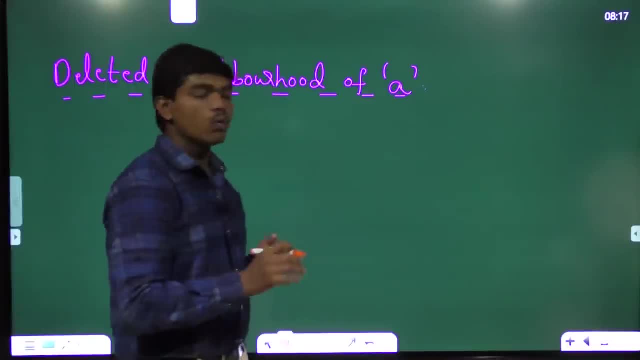 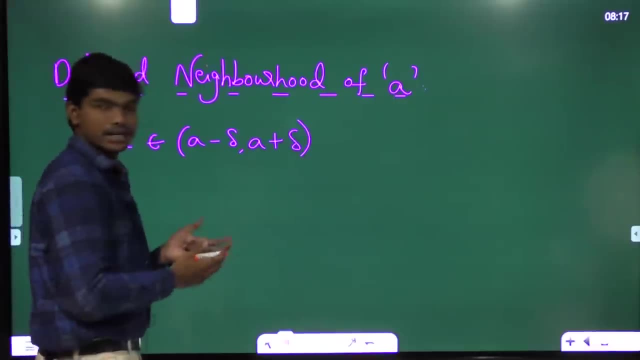 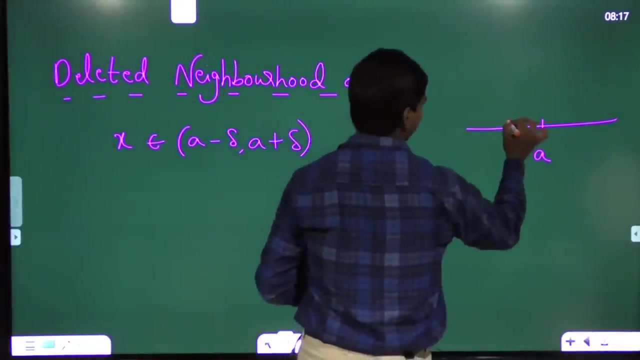 neighborhood or that interval. A minus delta to A plus delta. Now what we are really deleting. You know this. x belongs to A minus delta comma. A plus delta is the interval where the real numbers are very close to A. If this value is delta, then this is A minus delta. Similarly, 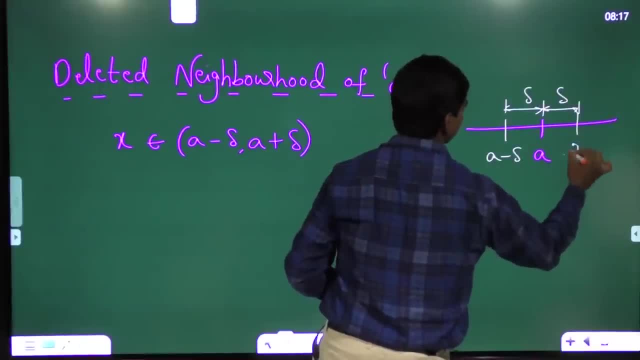 if this is also again delta, then this is A plus delta. So this is the interval where the real numbers are very close to A. If this value is delta, then this is A minus delta, Then this is A plus delta, which means this is the neighborhood. Now, from this values, 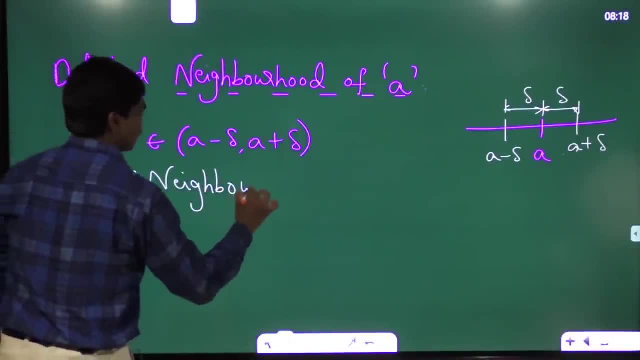 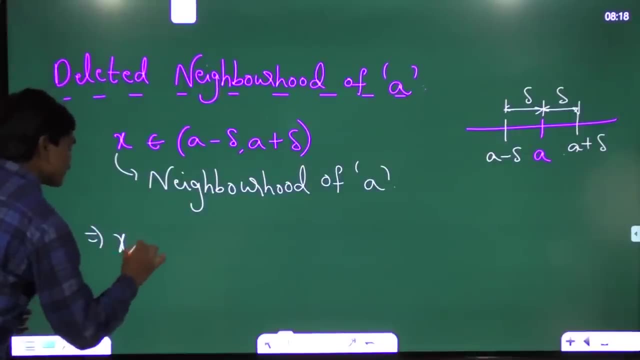 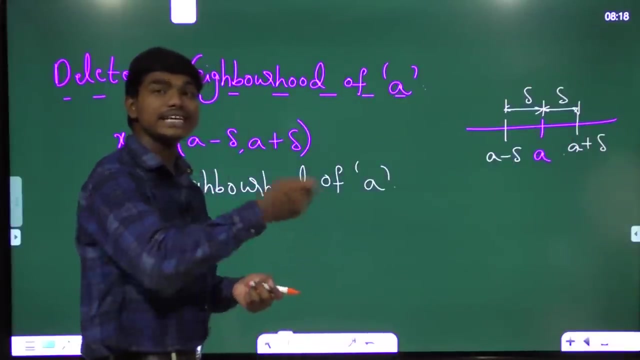 of x. as you know, this is the neighborhood of A. Now, from this values of x, if you subtract A means from this interval, if you remove this one point, then that's called deleted neighborhood, Because we are deleting that A from this interval. So x belongs to A minus. 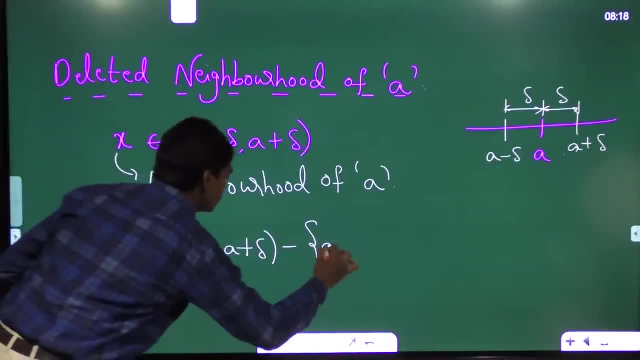 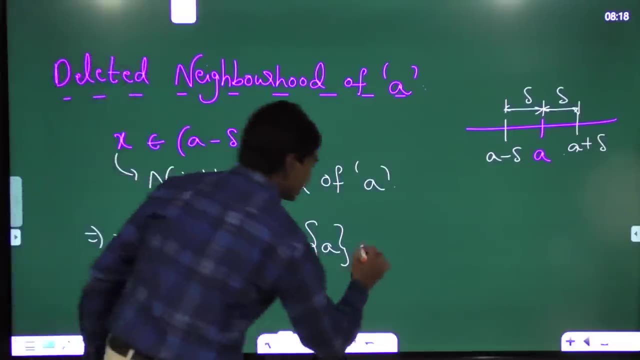 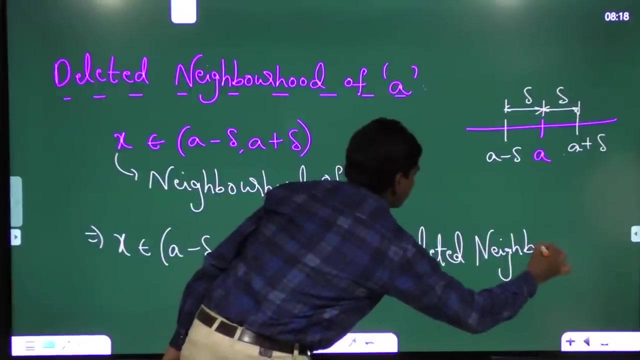 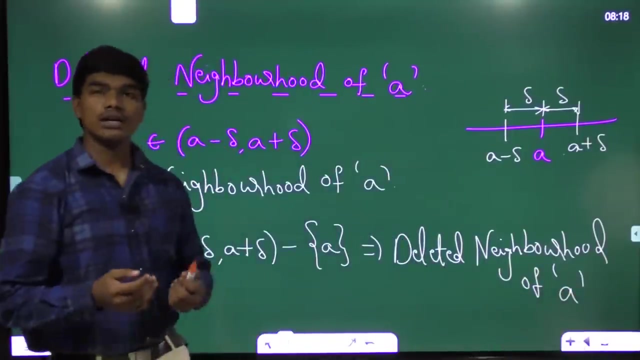 delta comma, A plus, delta minus. we need to remove this a from this interval. then this interval, which is actually this, without having a in it is called deleted neighborhood of deleted neighborhood of a and whatever the limits that we deal, we are dealing only in this interval. 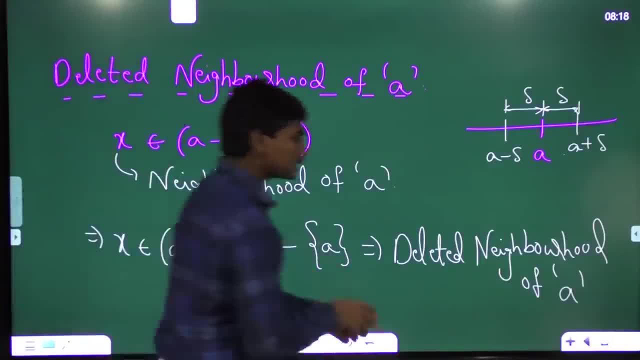 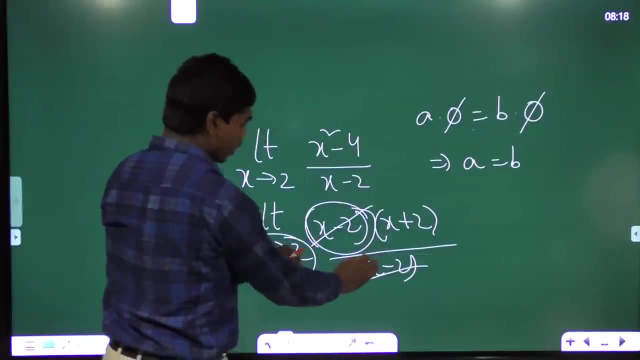 and, if you see, this interval doesn't have a in it and that's the reason when we are writing this limit, x tends to 2. we are canceling. we are able to cancel because this x is in the neighborhood of 2 and i mean, to be precise, in the deleted neighborhood of 2, which means x can't take. 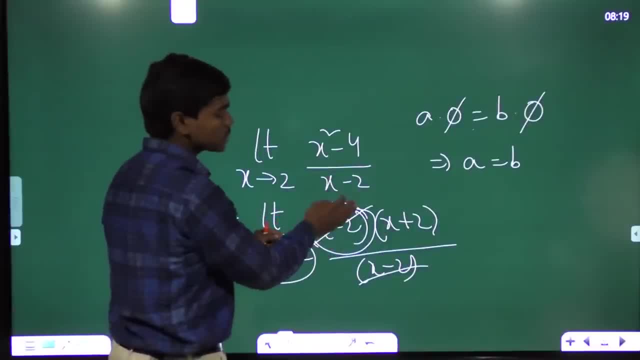 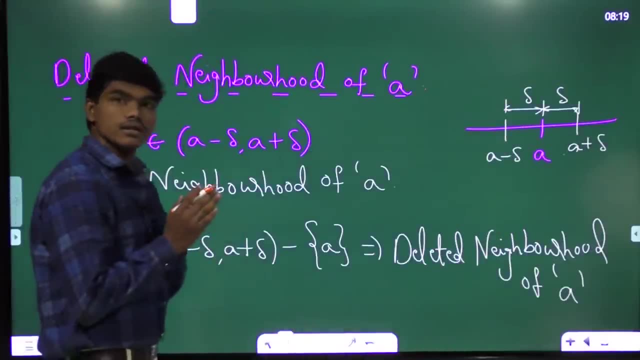 the value of 2. so when x can't take the value of 2, this x minus 2 can't be a 0 and you can cancel these two, undoubtedly correct. so this is the difference between x equal to a and x tends to a. when x is equal to a and x tends to a, then x is equal to a and x tends to a and x tends to a. 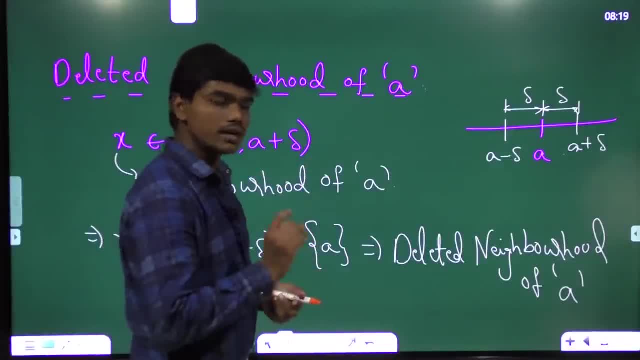 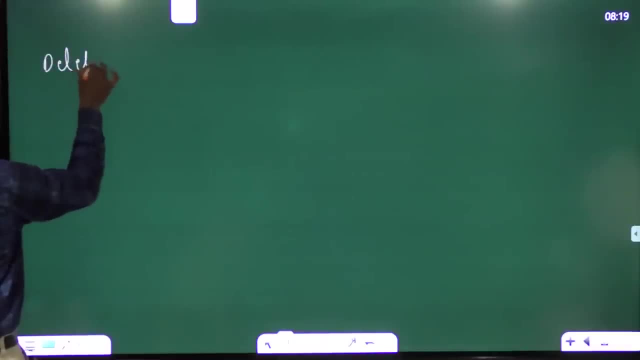 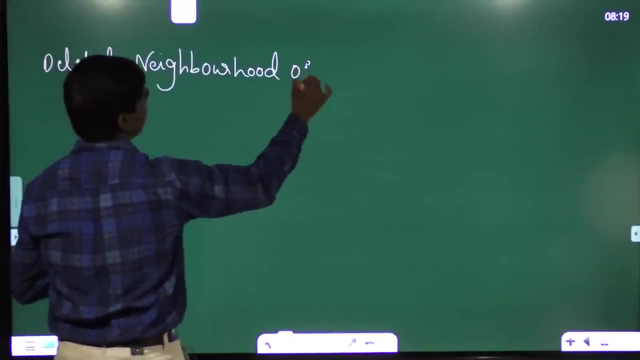 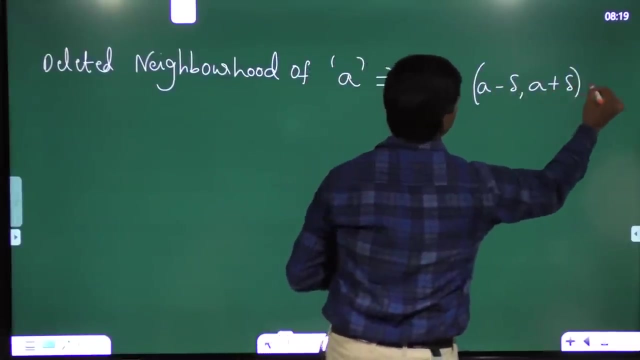 when x is equal to 2, you can't cancel the two fractions. when x is tending to 2, you can cancel that next. so right now you have seen deleted. neighborhood of a is deleted. neighborhood of a is a minus delta to a plus delta minus. we are subtracting this element. 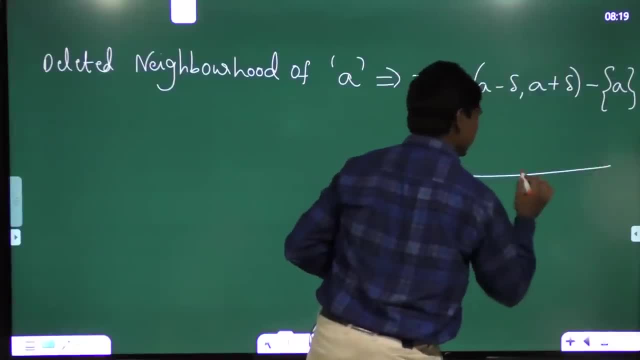 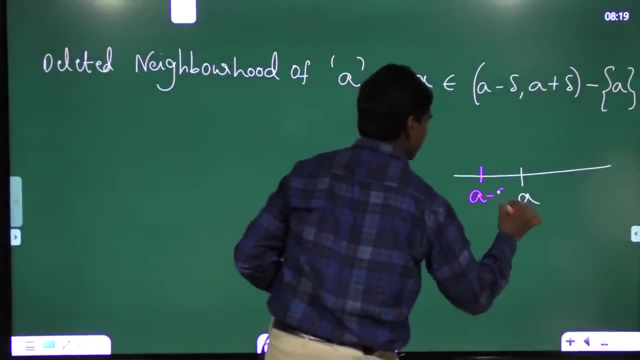 a, which means now, if you look at this element, you can see that this is a minus delta to a plus delta. if you consider this number line here, if this is a, and now if this is a minus delta and if this is a plus delta, of course these values are. 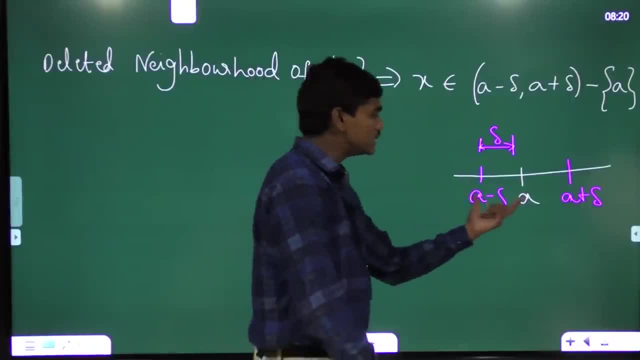 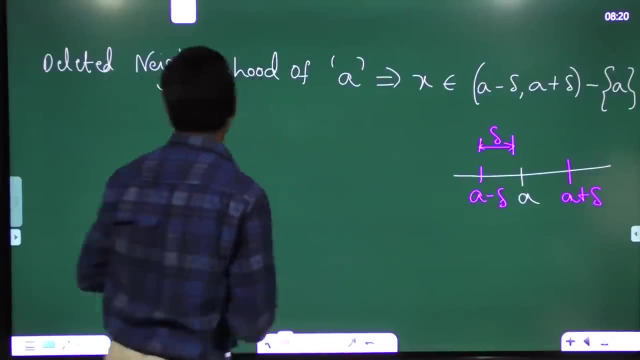 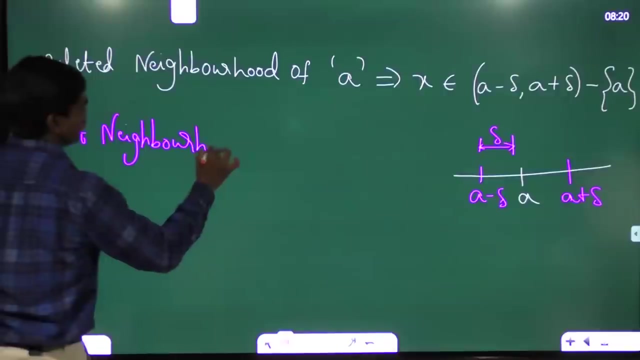 delta. now, one thing is very clear: this: a minus delta to a means, this interval, a minus delta to a is to the left hand side of this a. so for that reason it's called left neighborhood of a, left neighborhood of a, and it is denoted by denoted by a minus. be careful, my friends, this is. 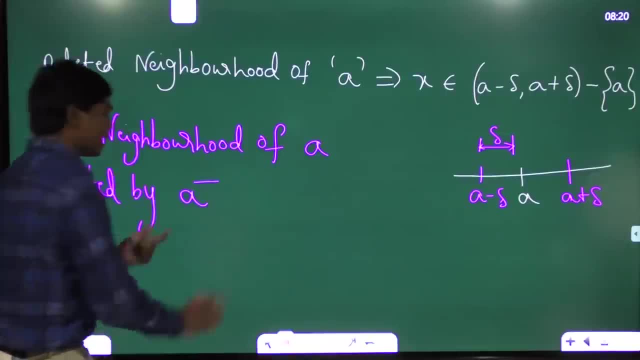 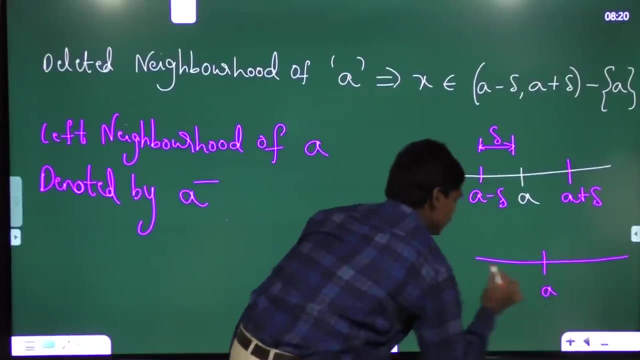 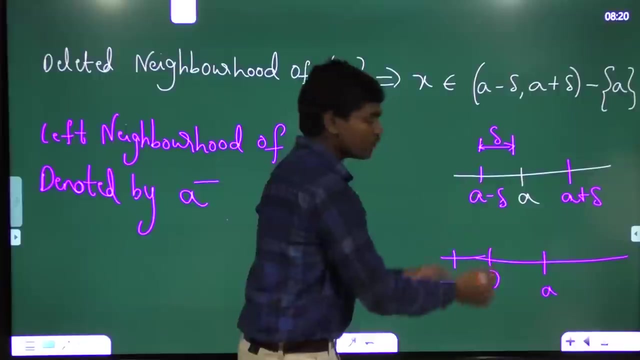 let me write it clearly: a minus, this is a minus, which is very different from minus a if you consider number line again, if this is a somewhere here, this is minus a and somewhere there is origin in between. but this a minus means this left neighborhood of a is to the left side of a minus delta to a. 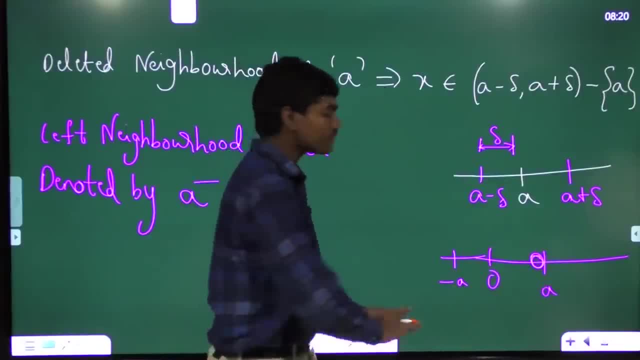 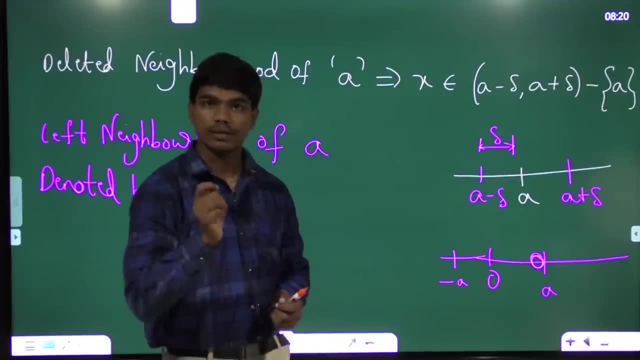 a is somewhere here, but not this. okay, so left neighborhood of a is here but not here, which means this minus a and a minus which is left neighborhood of a are quite different. okay, so please make a note of this because later in problems, whenever you need to deal with a minus, 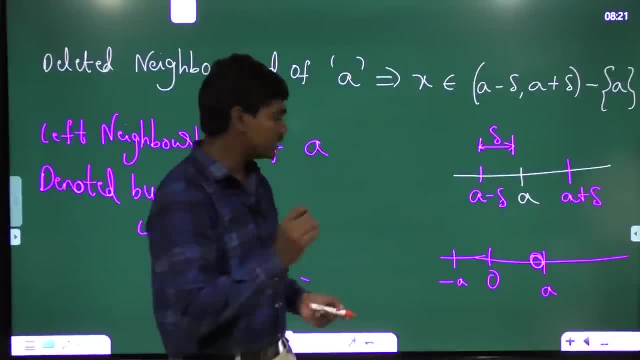 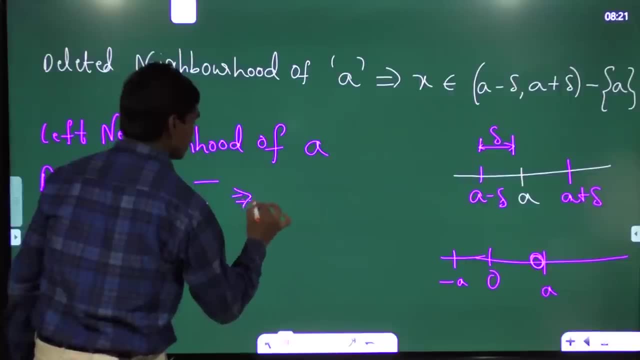 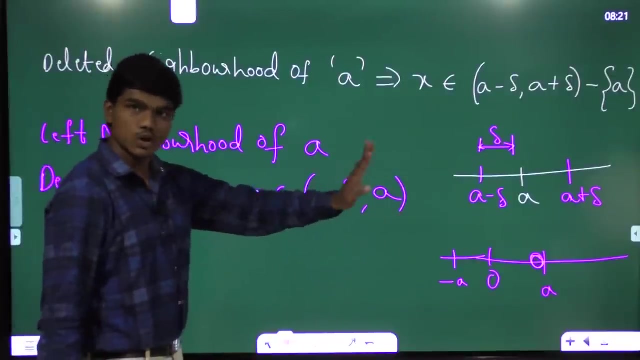 i see many students substituting minus a instead of a minus. okay, so please make a note of that. okay, so a minus is equal to or implies x belongs to a, minus, delta to a. now, if you see one thing, i put an open bracket here, which means i don't put my a inside this, and it includes the values. 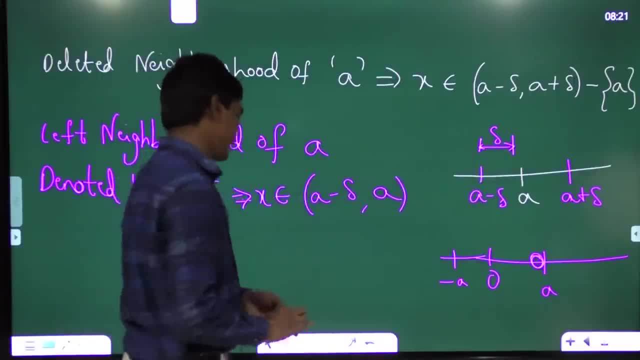 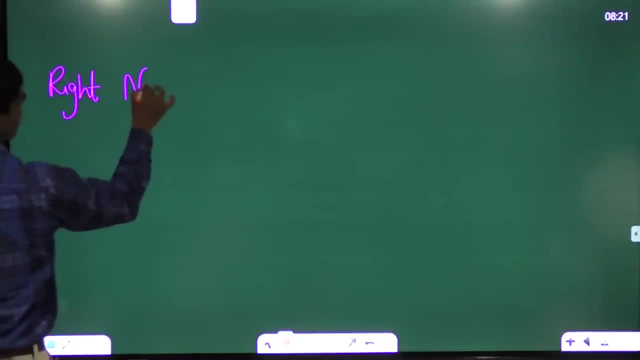 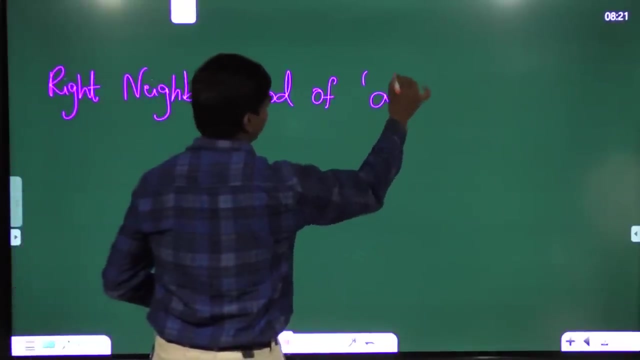 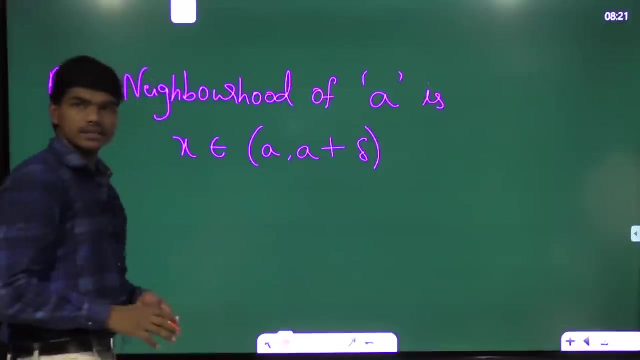 between a minus delta to a, which is left neighborhood of a. similarly, what would be the right neighborhood of a? could you guess right by your own what is the right neighborhood of a? okay, so right neighborhood of a is x belongs to a comma, a plus delta. okay, because a minus delta is on the. 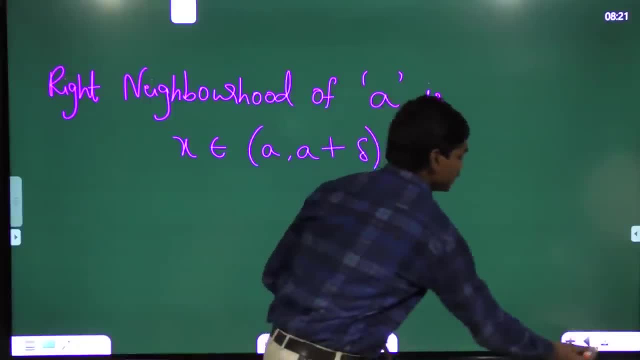 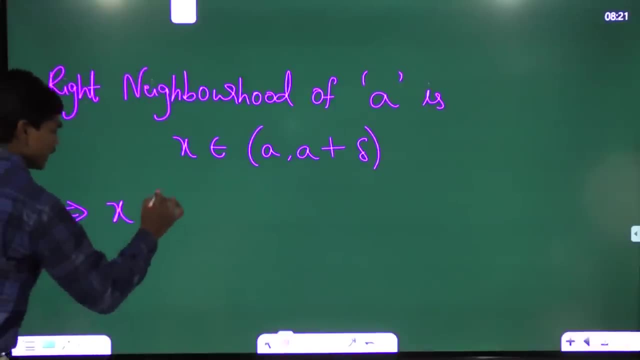 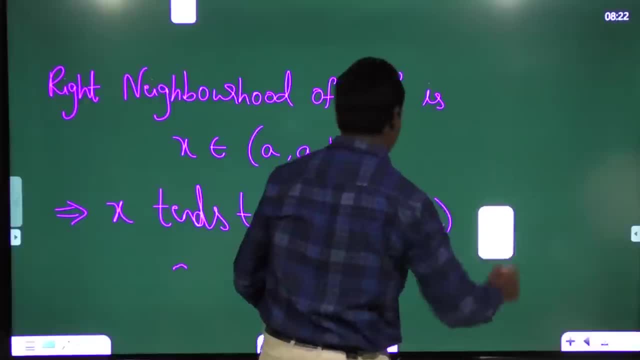 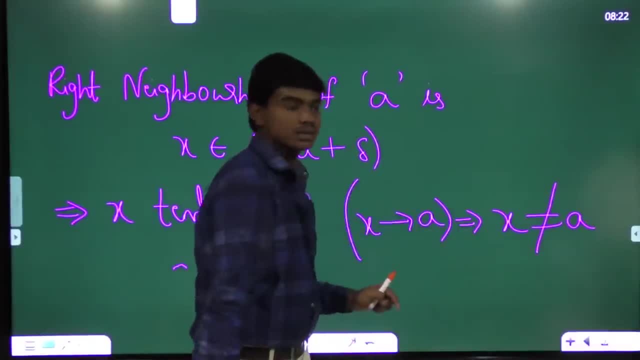 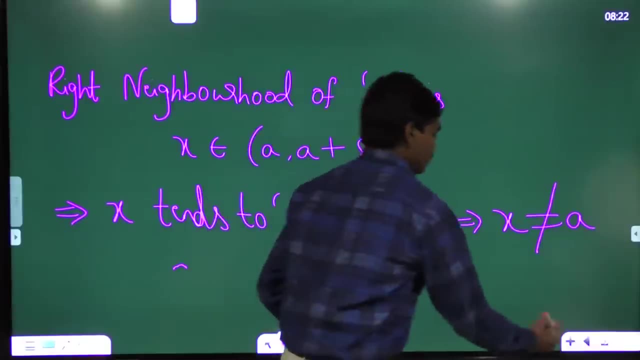 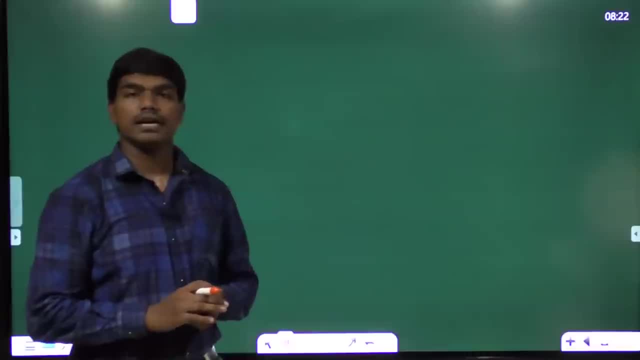 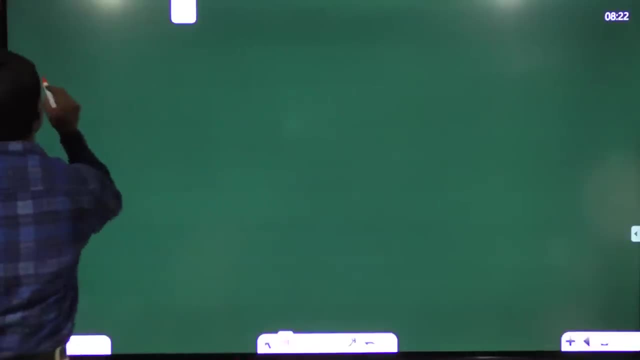 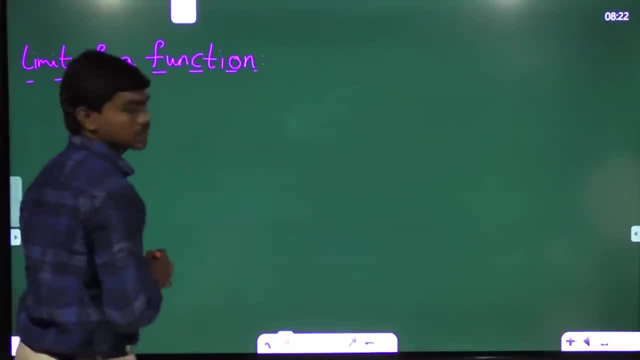 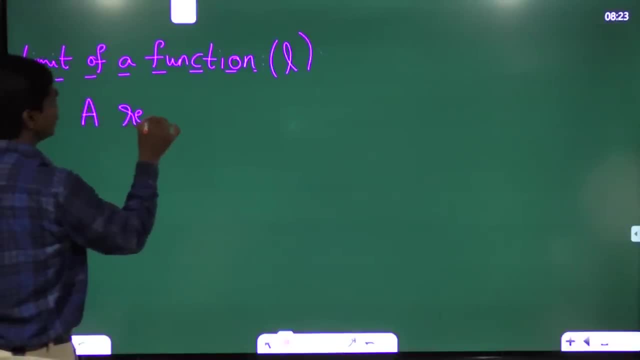 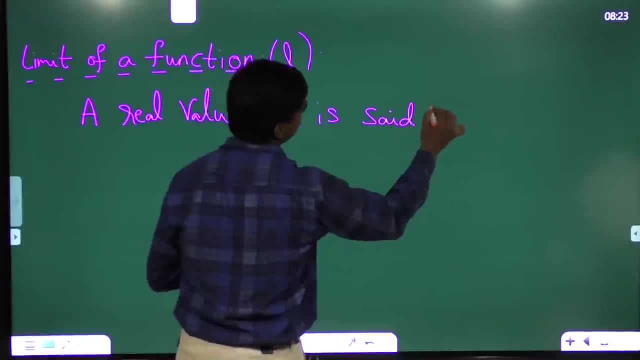 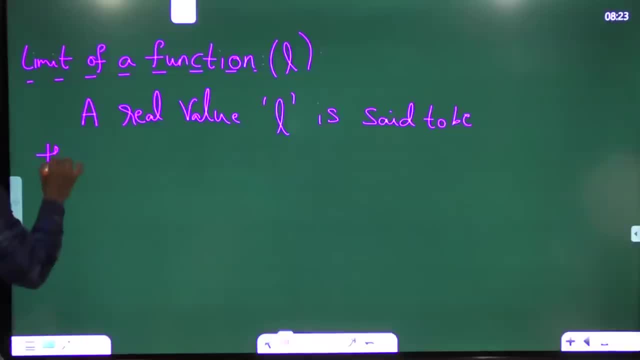 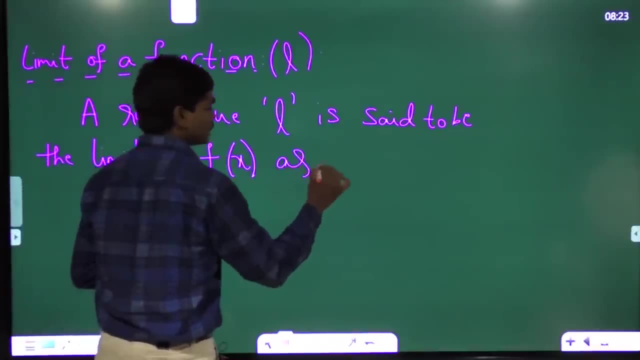 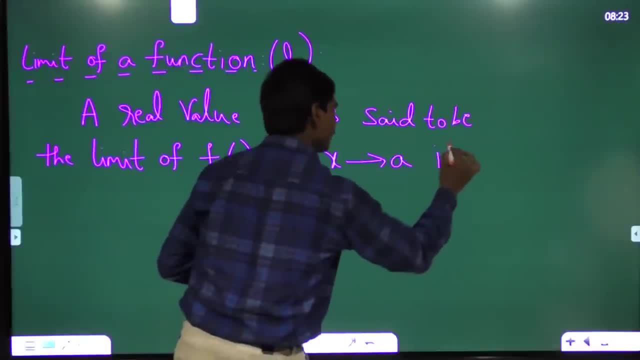 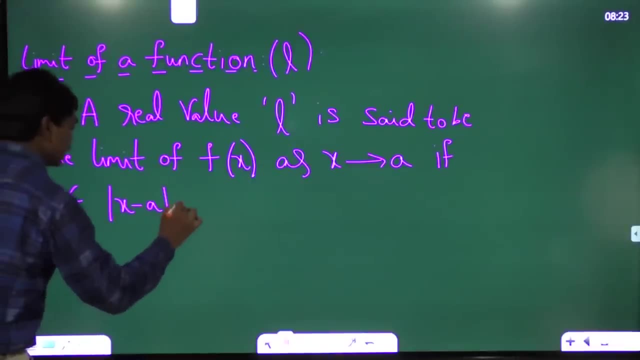 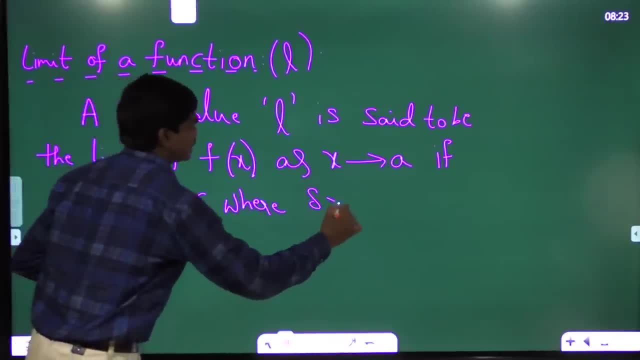 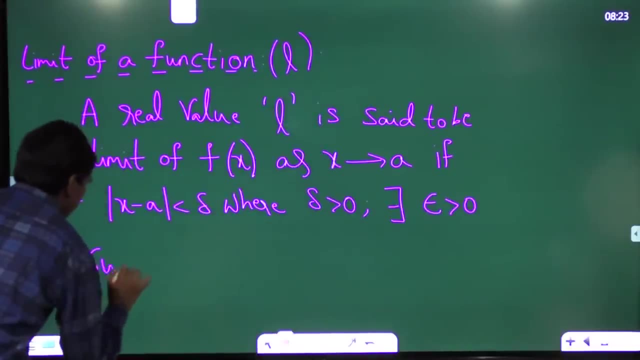 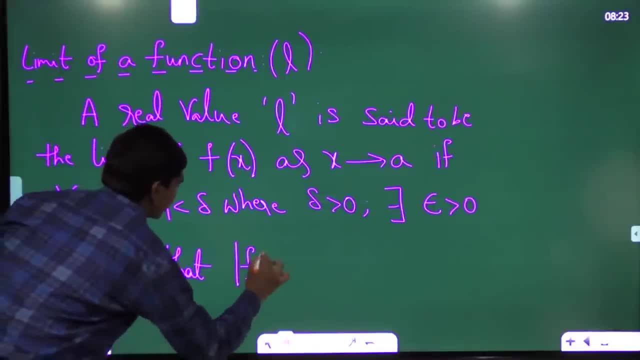 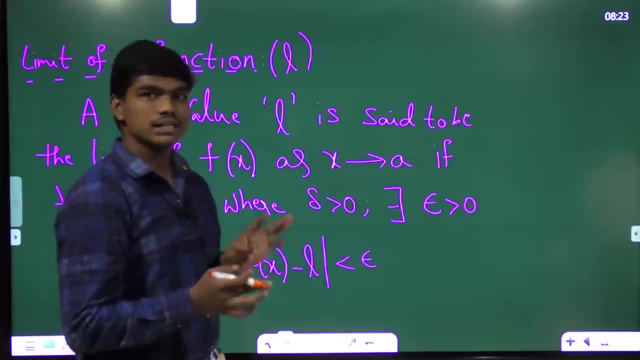 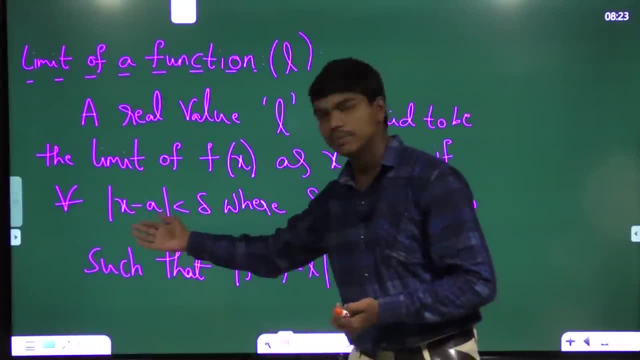 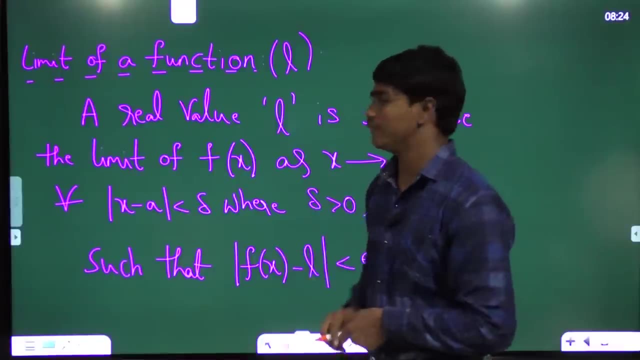 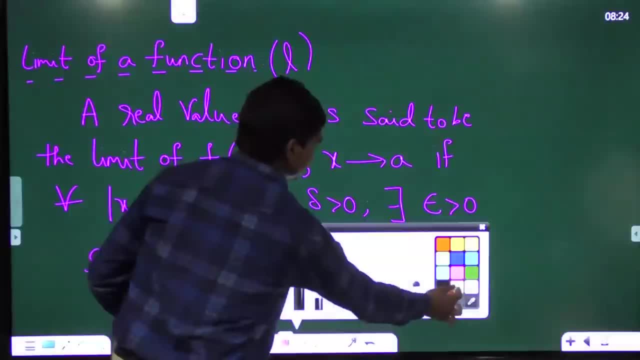 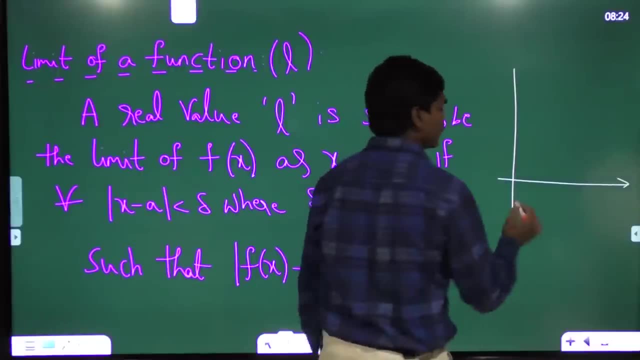 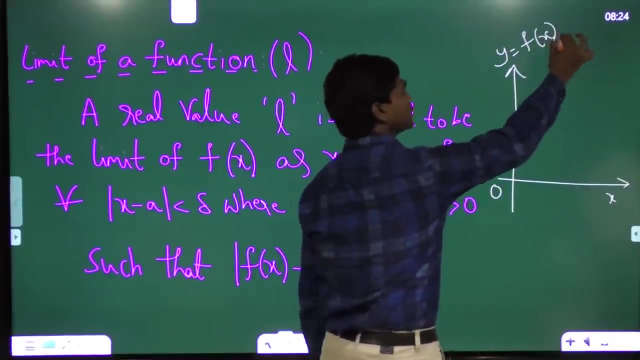 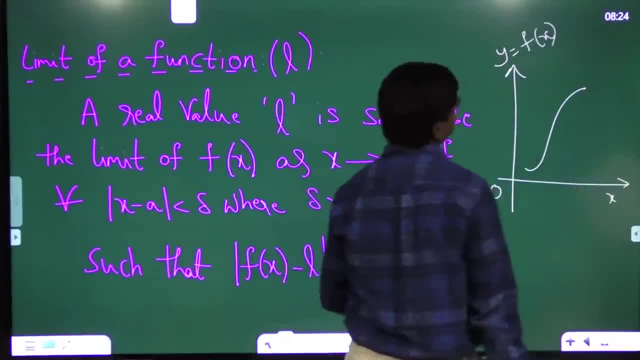 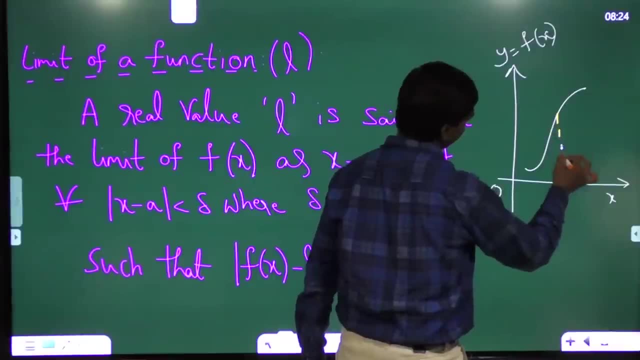 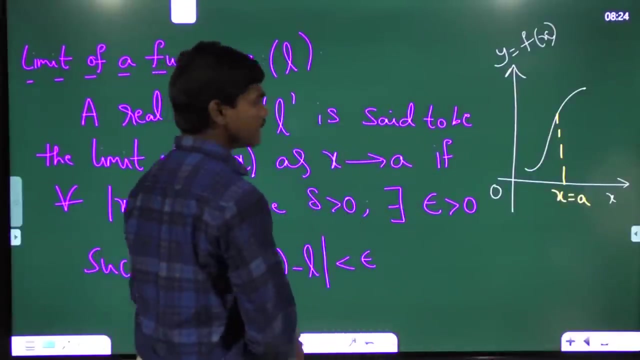 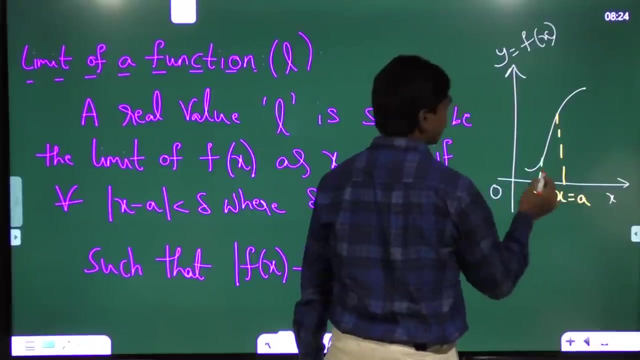 f of x. And let us suppose the function is something like this: And at this point let me write one thing: This is the value: x is equal to a, x is equal to a. Now, if I write x somewhere here, let us suppose this is x and let us suppose this value is. 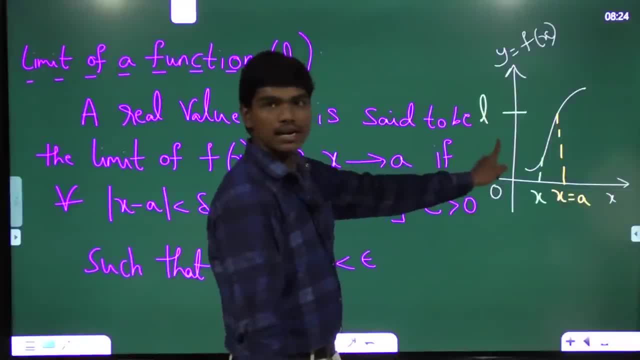 l Now understand one thing clearly: this l doesn't have any interlink with this f of x. This l is just a number on a y axis. that's it. This l- I am repeating this l doesn't have any interaction with this f of x. 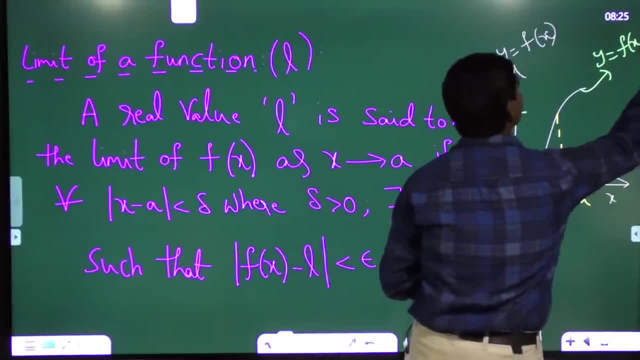 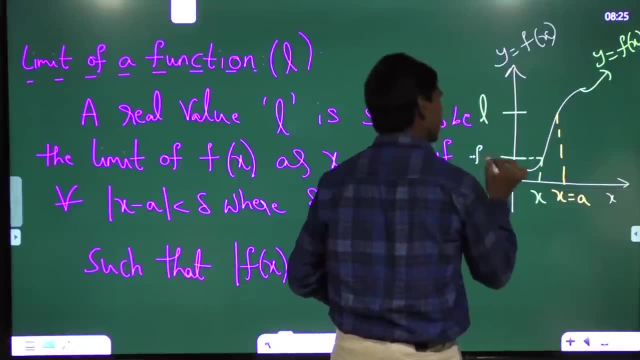 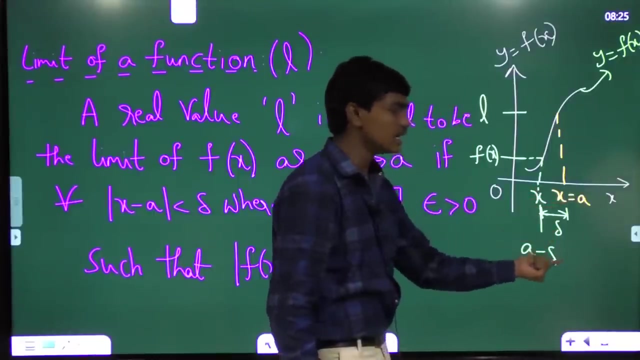 It is only a real number on y axis. Now, if this is x at this moment, this is f of x, and let us suppose this value is delta, Then it is known that this value is a minus delta. If this is delta, this value of x is a minus delta. 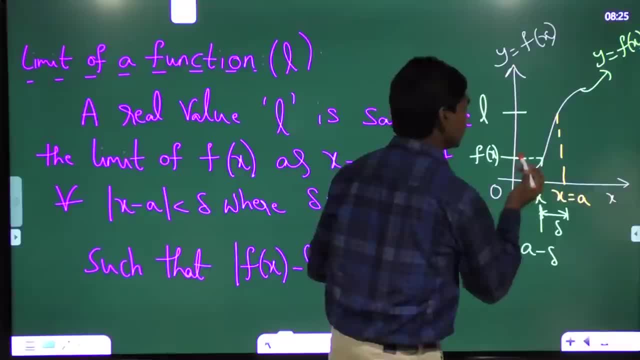 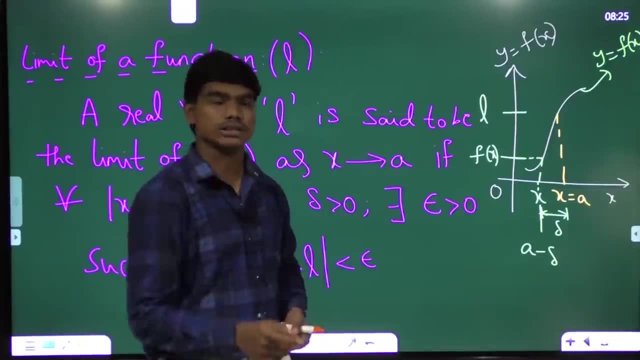 At a minus delta. the value of this f of x is somewhere here. So this is a minus delta. So this is a minus delta. Now x tends to a. What is the physical meaning of this? When x is tending to a, that means x is moving towards a. 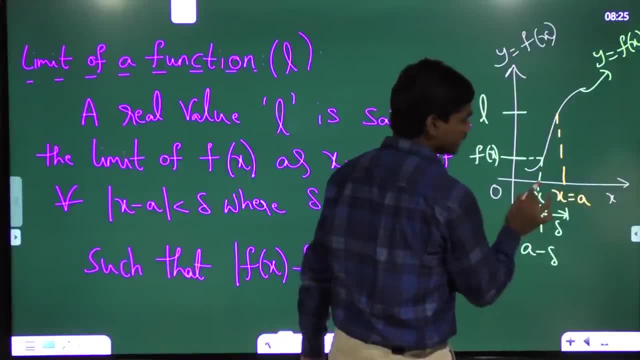 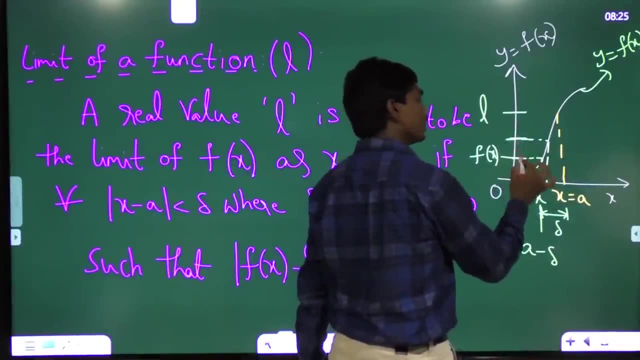 So if I move my x towards a, it means the x which is initially at this point. if I move a bit towards the right, then my f of x changes from this point to this point. Let me call this point a and let me call this point b. 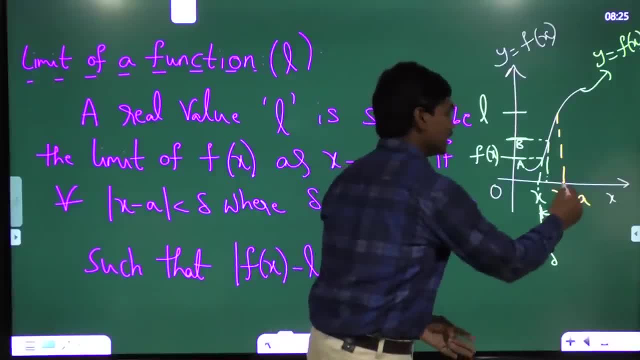 So when I am shifting my x towards the right or towards a, this f of x is slightly increasing. Or it can decrease as well, Or it can decrease as well with respect to the curve, but in this particular case it is increasing. 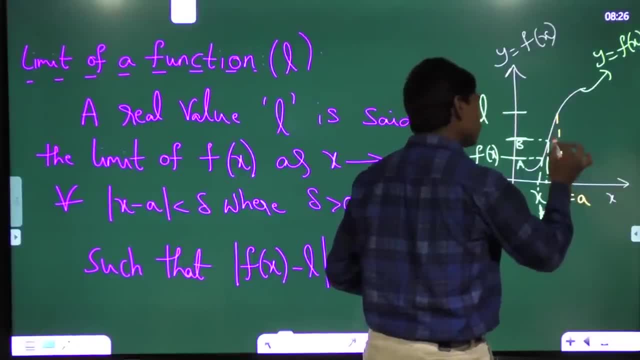 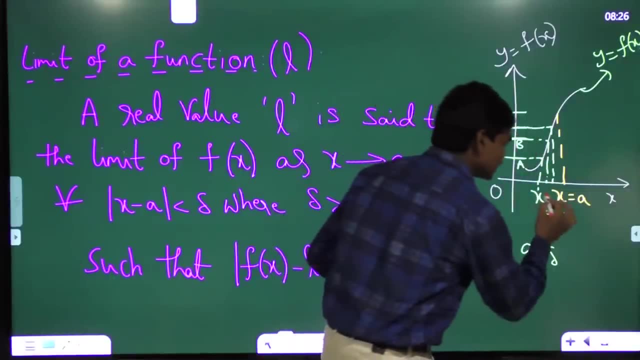 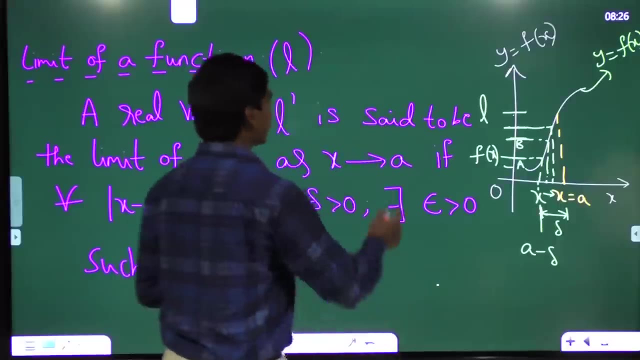 Which means now, if I further increase my x, if I further move towards a, this f of x is further increasing. Now one thing you can see very clear: when x is tending to a means, when x is moving towards a, this f of x is moving towards l. 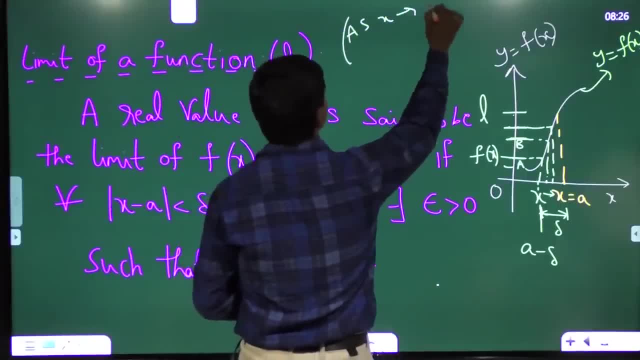 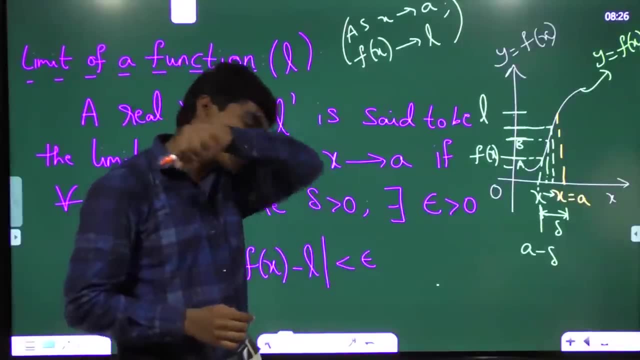 So we can write that, as x tends to a, f of x tends to l? Correct, Yes, Correct. Now you may get a question, Sir. you told x tends to a, but you didn't say from which direction, because x can be. 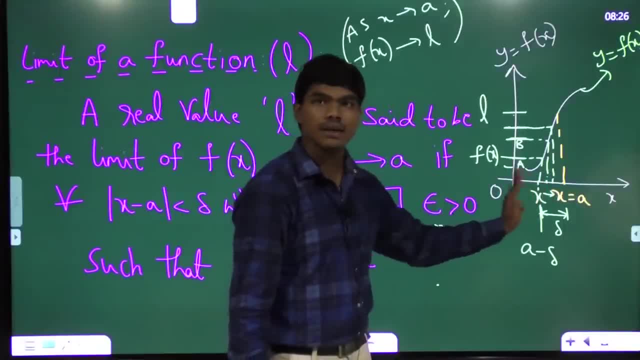 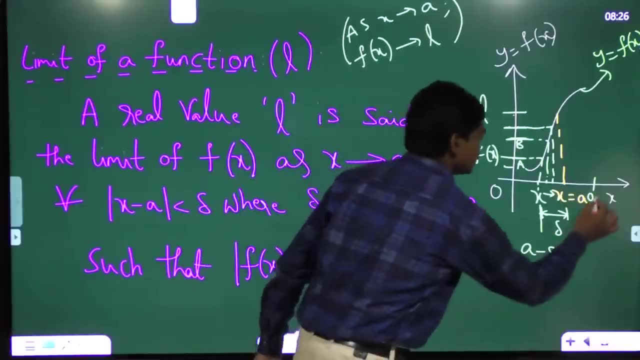 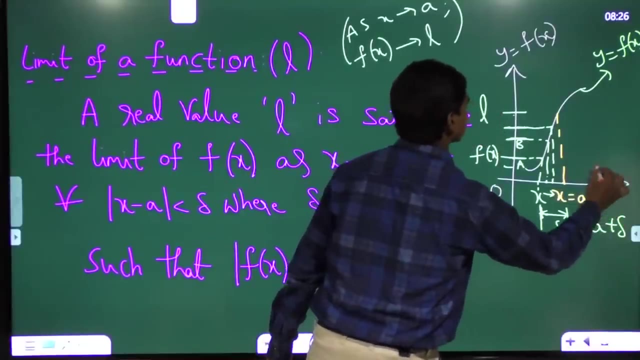 in the left neighbourhood and it can tend to a towards left hand side. or x can be in the right neighbourhood of a, where this is basically: let me, is this zero here, where this value is a plus delta and my x can be here. 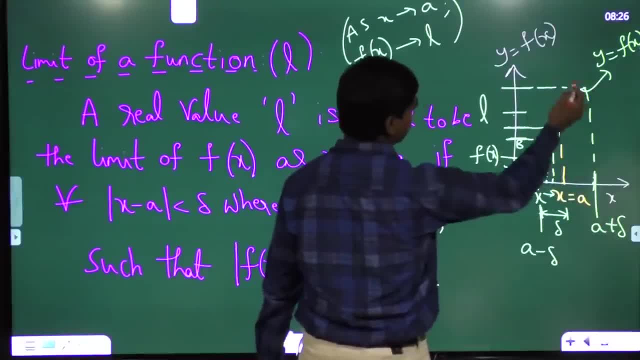 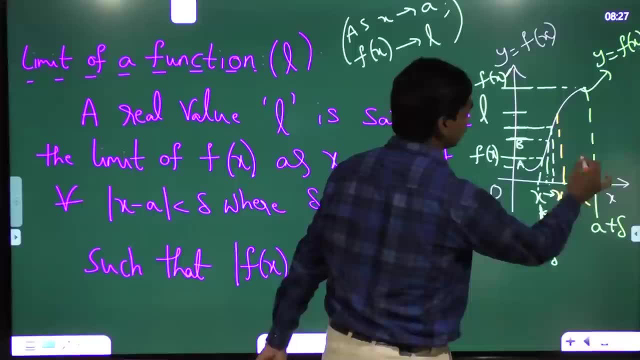 You can get that question. If this is your x, then this is your f of x. And again, if you are tending towards a means, if you are moving your x towards a, for example, if you move in this way, again your f of x is coming down towards l, as you tend to. 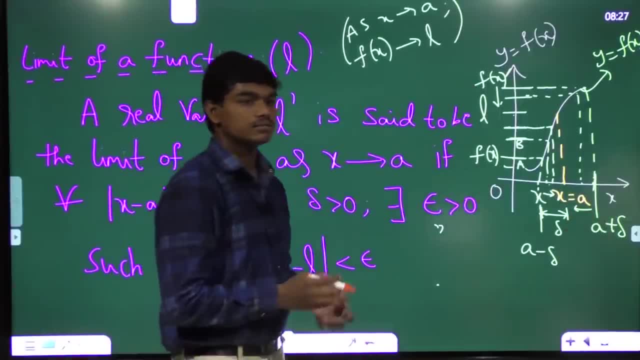 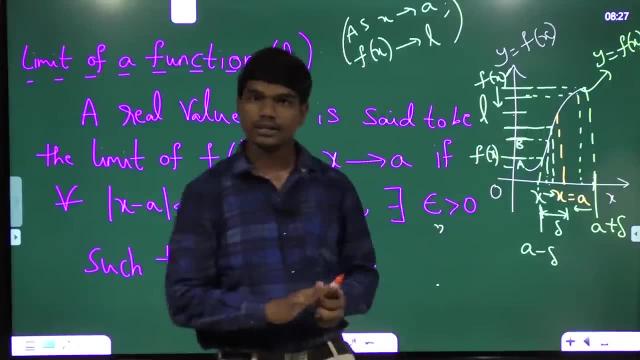 x tends to a Means. one thing is very clear. One thing is very clear. So, as x is tending to a f of x is tending to l, Did you understand these two things? It doesn't matter from which direction you are tending towards a. 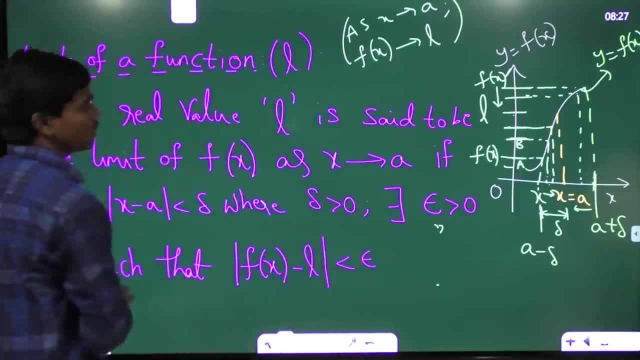 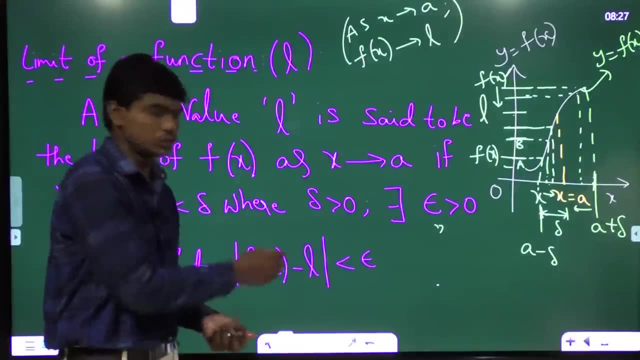 Correct, So please take it till here. You take the definition of limit and try to take this graph here, so which you can get few things, And we will discuss more about this limit once you take this definition. Please take it. I will give you a minute for you. 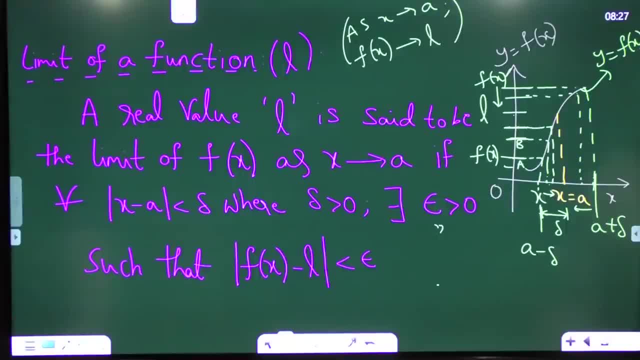 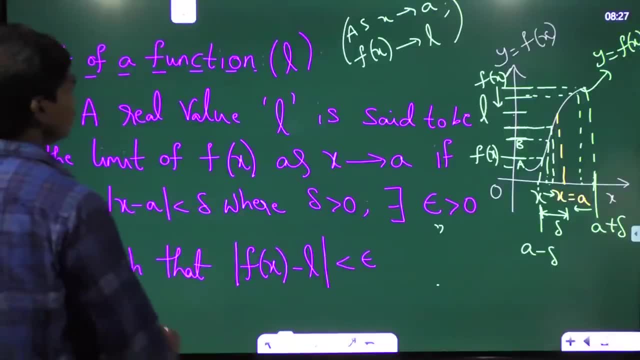 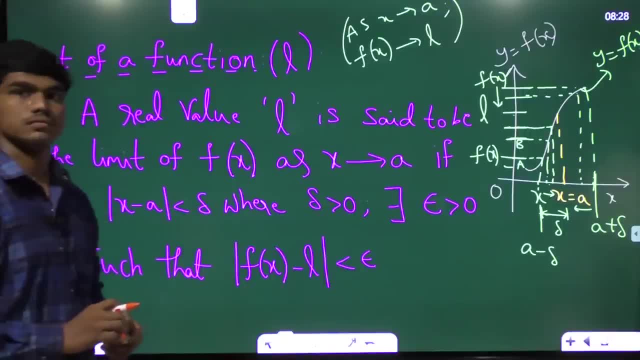 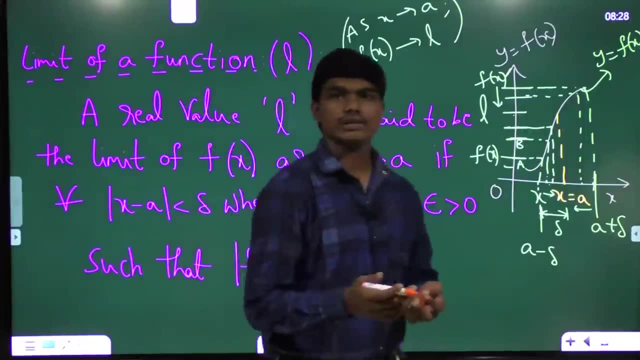 Sorry, Sorry, Sorry, Sorry, Sorry, Sorry, Sorry. So now I would like to proceed. If you are lagging a bit, you can pause the video at that moment and you would write the definition. Now I would like to reexpress this technique and reach the next step. 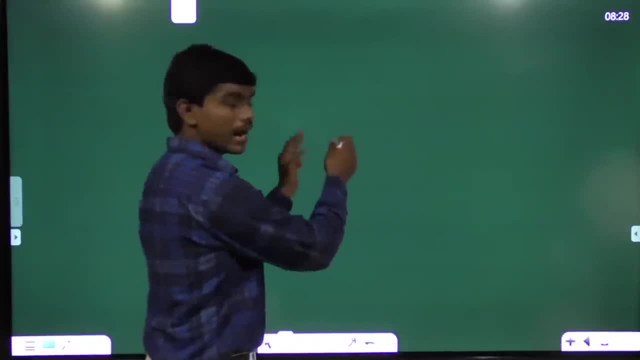 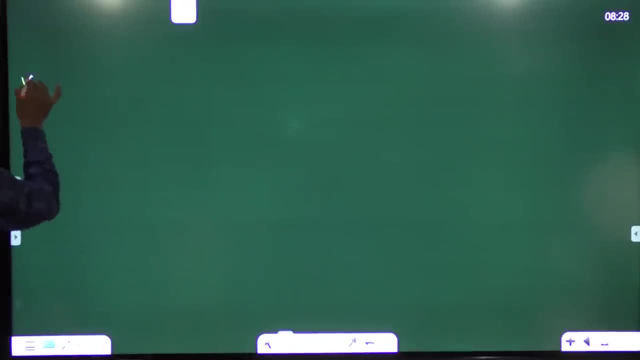 I would like to re-explain this diagram once again, because we have- we need to put few more things in that diagram, So let me draw the diagrams clearly. Before drawing, let me write two things here that I mentioned. For all x minus a less than delta, where delta is positive. 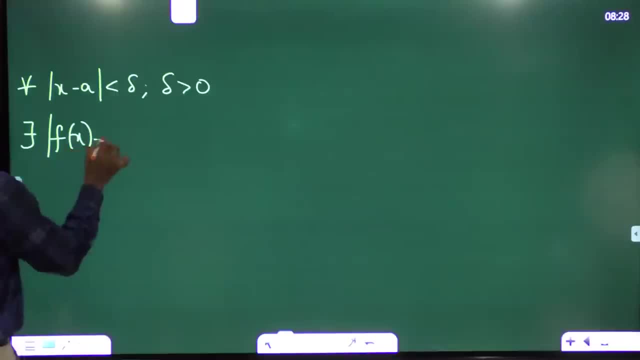 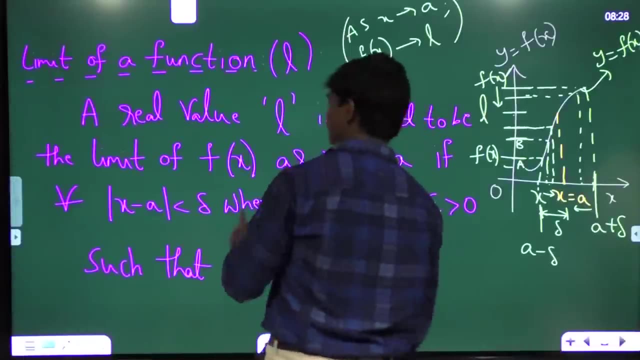 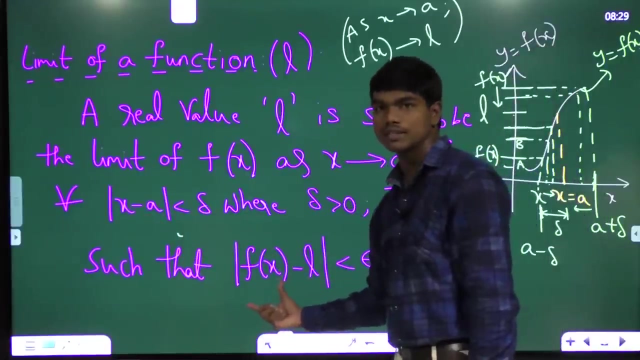 there exist, f of x minus l under modulus is less than epsilon, where epsilon is greater than zero. These are the two key points that I mentioned here. If you see, for all x minus a less than delta, there exist epsilon, such that this mod of f of x minus l is less than epsilon. So now, 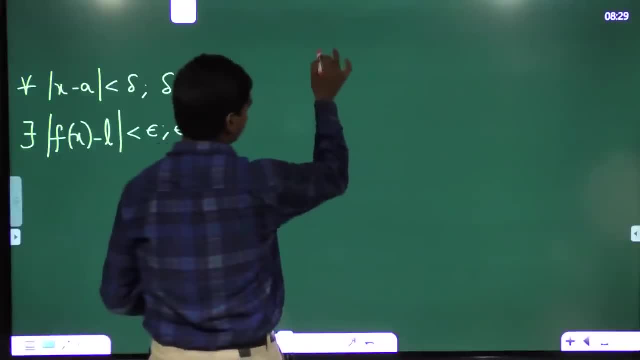 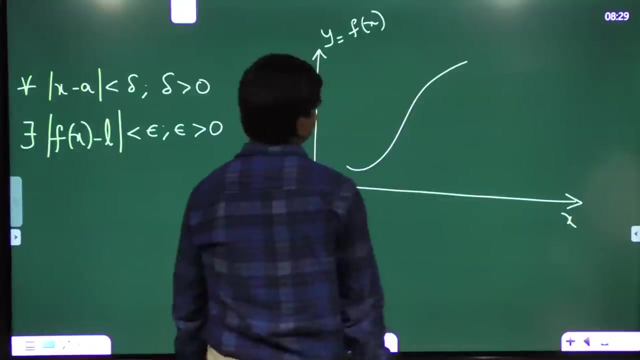 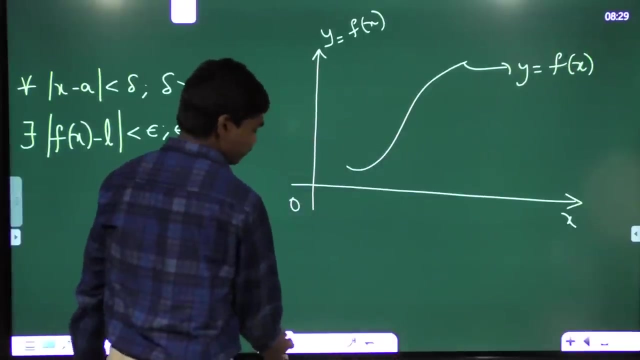 let me draw the diagram which I have drawn for you again: Zero x, y, where y is some function of f of x. Now suppose this is the curve: y is equal to f of x. Okay, Now let me mention those points again which I mentioned in earlier diagram. If this is the 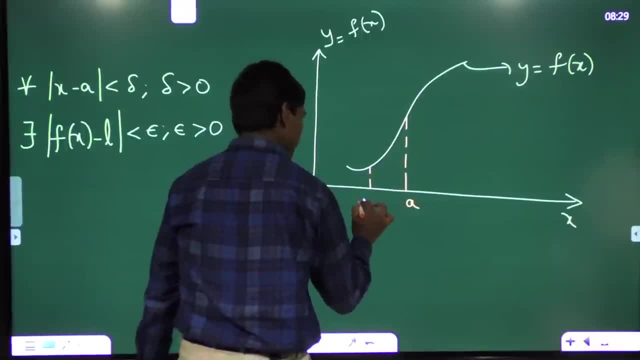 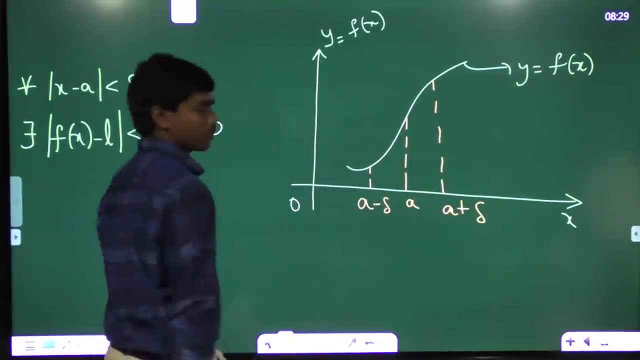 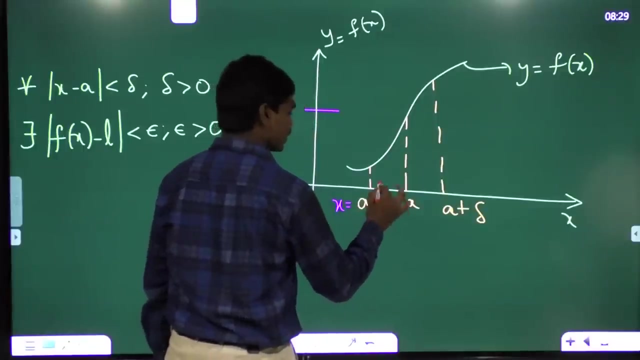 point a and if this is the point a minus delta, and if this is the point a plus delta. Okay, Now I also mentioned this value is l. This l is just a number on y axis. Now thing is, if your x is initially here and if you start moving towards this a means, if you move this x towards a, you 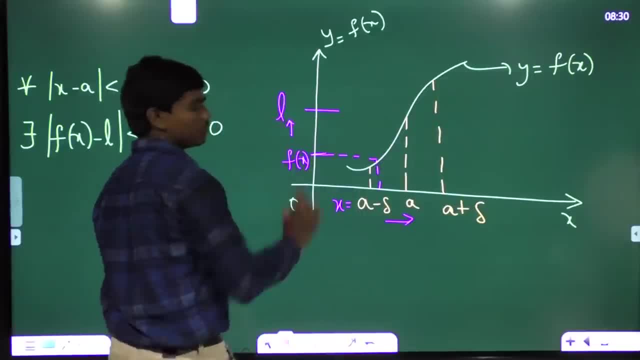 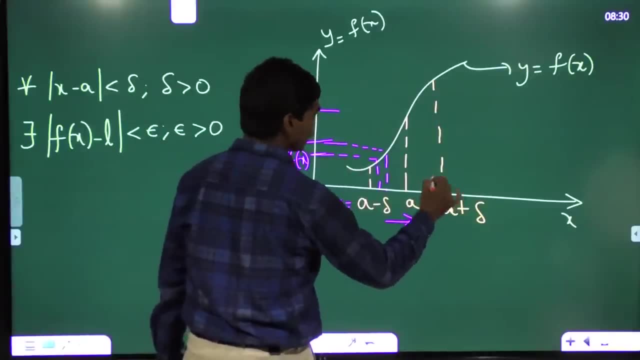 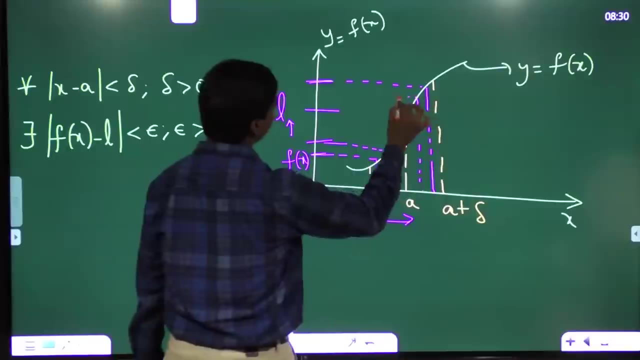 have seen this f of x is moving towards l- Okay. Similarly, it goes on Similarly on the right hand side. if you consider this initially, your f of x is somewhere here. Now, if you start moving towards a, this f of x is coming towards l- Okay. 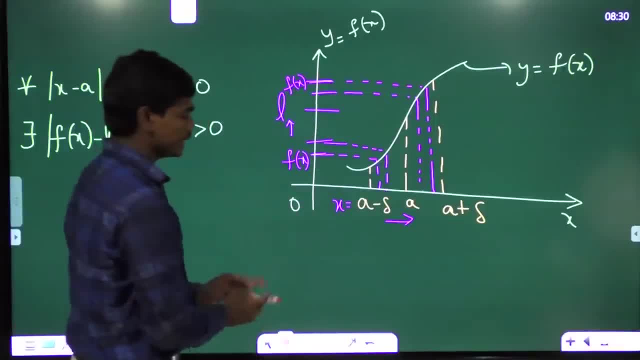 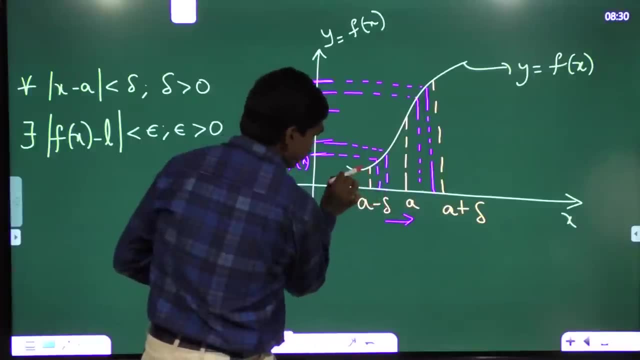 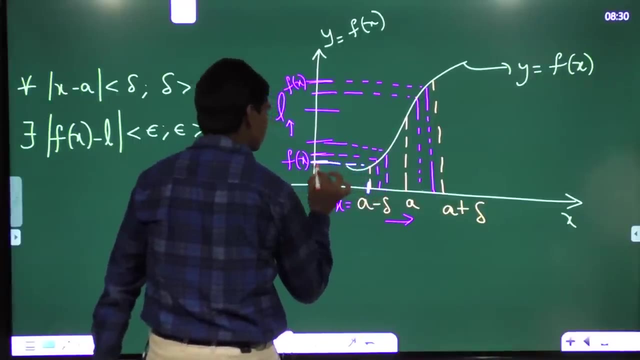 Now let me write: this is the previous diagram. that's what you have seen. Now let me add few things here which could make some use to you. Now see this point here which we are talking here is a minus delta, and let us assume the functional value here means this white line is f of x or you. 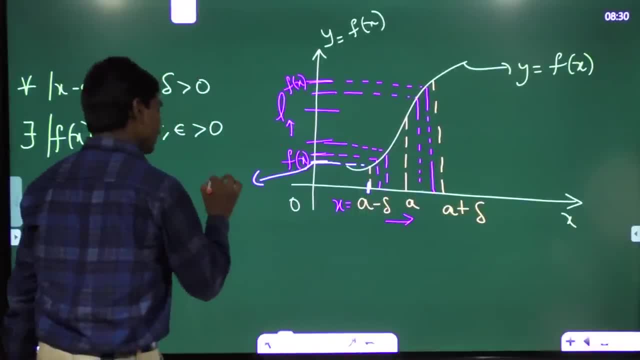 can write this as for the time being: l minus epsilon. Okay, where epsilon is something which is greater than zero, and of course you know l is nothing. but where epsilon is something which is greater than zero, and of course you know l is nothing. but where epsilon is something which is. divided by a 뭔가 nt. that means y right, where epsilon is something which is greater than zero, and of course you know l is nothing, but where epsilon is nothing, but where epsilon is non exponent, and And of course you have to do like then to get out This next general diferencies of what you. 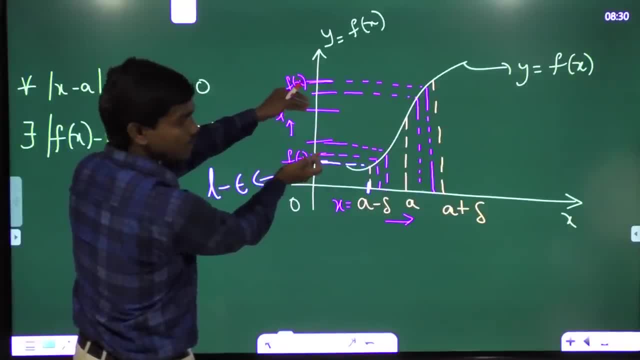 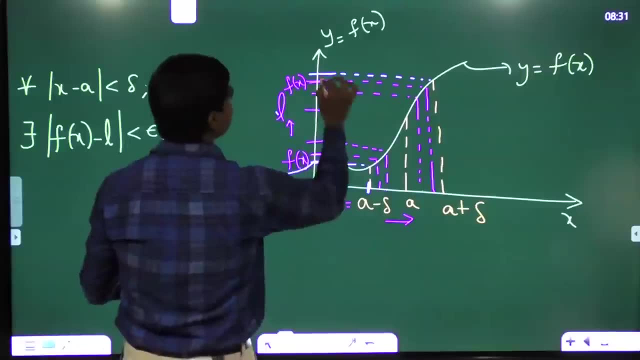 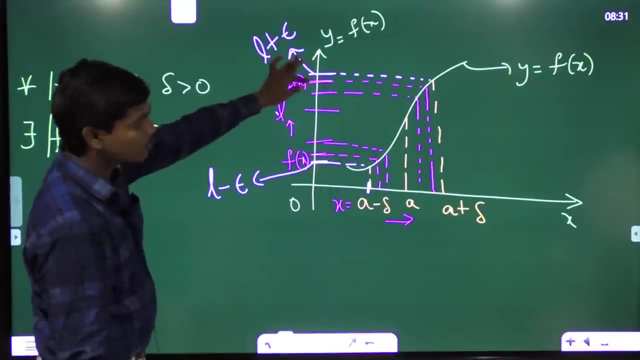 only since the top of this. this value is definitely less than L and that small difference. I am considering it as L minus epsilon. Similarly, here, at this point, if you see, let me consider this value as L plus epsilon, okay, because you know this point is slightly above L. so 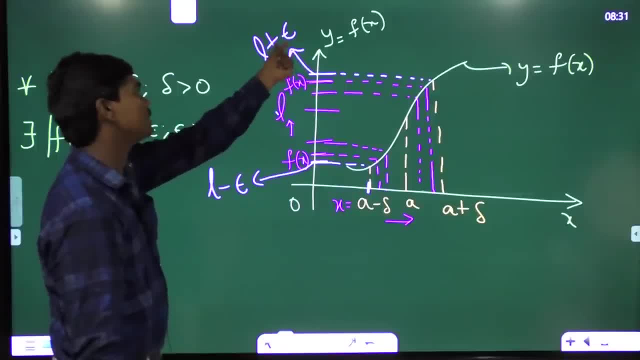 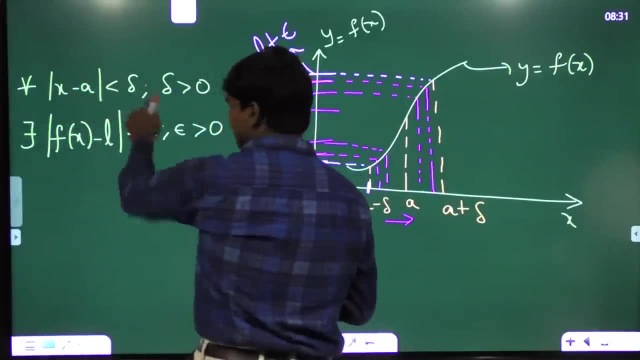 there is some difference between this L and this point, so that difference is compensated by this epsilon. Now one thing you need to observe here. observe here: for all mod of x minus, a less than delta means this interval, basically a minus delta to a plus delta. 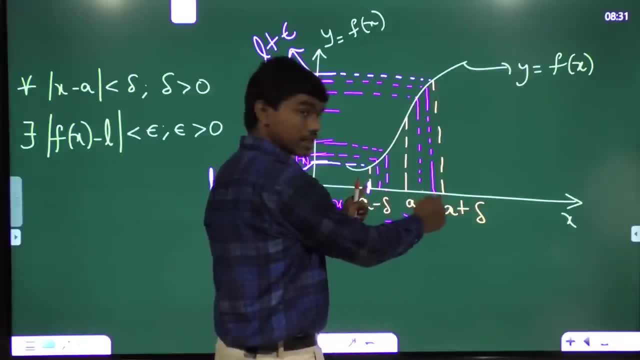 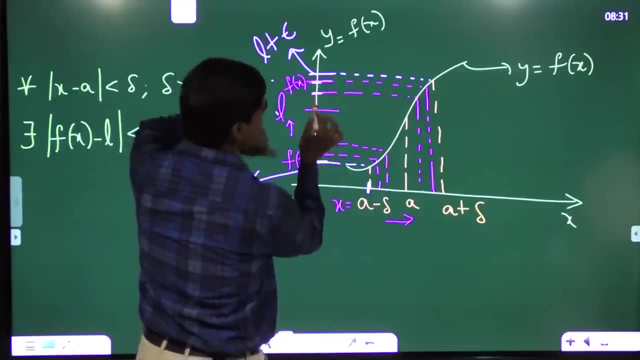 which we have seen. the neighborhood of a for all x belongs to this interval. there exists some difference between f of x and L At this moment. if you see, this is f of x. at this moment, this is f of x, but at every moment there is some difference between. 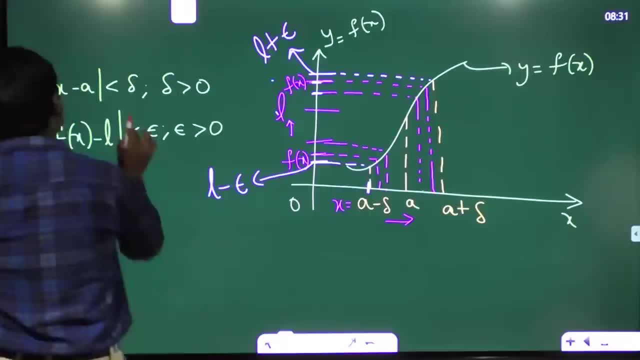 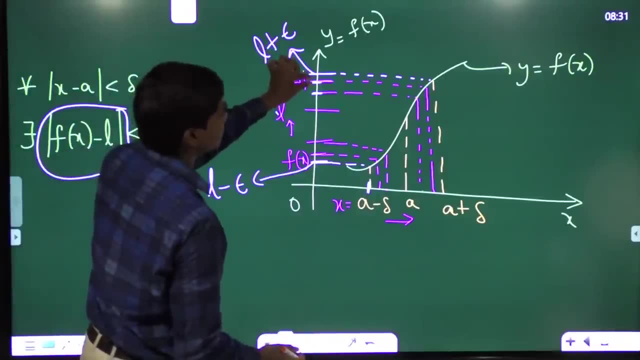 this L and this f of x, which means mathematically we can write this term as we have written for x, where f of x minus L means that there is always some difference between this f of x, So f of x and L, at every instant as you keep on moving to a, and mathematically we 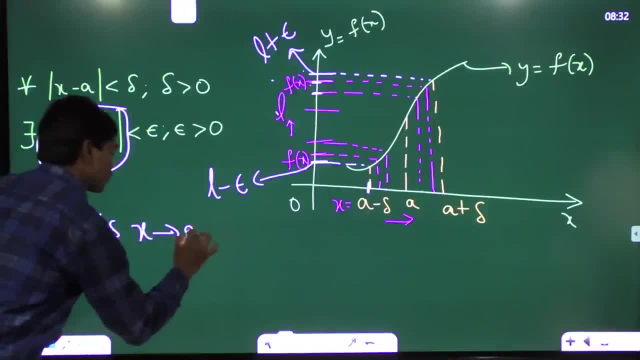 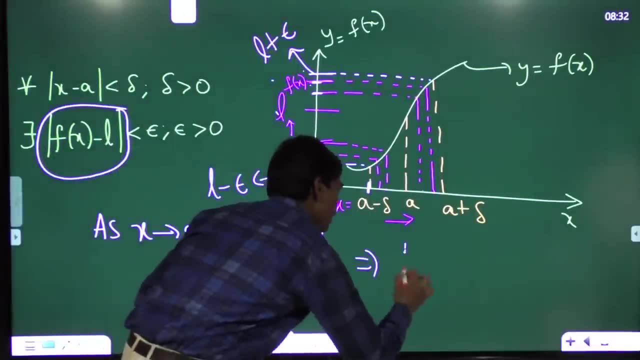 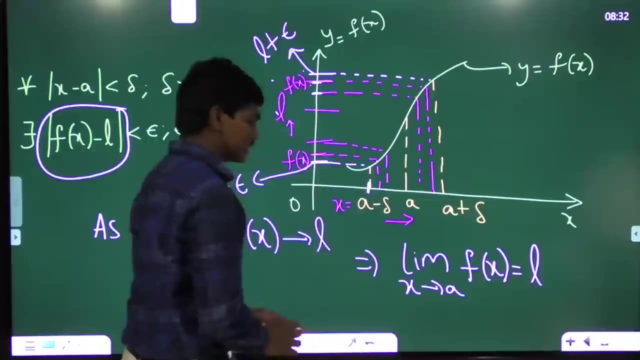 write this as: as x tends to a f of x tends to L, and this is mathematically denoted by the symbol limit x tends to a f of x is equal to L, which means whenever your x is moving towards a, which you can see in the diagram here, your f of x is moving towards. 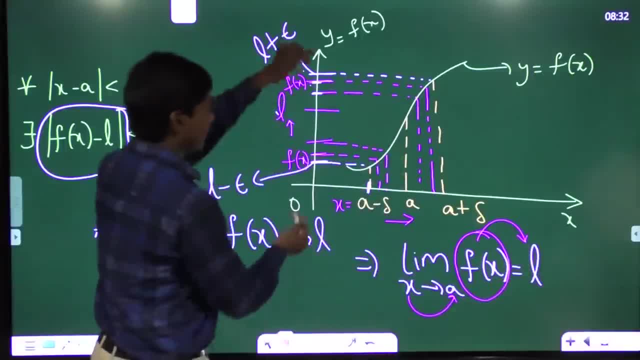 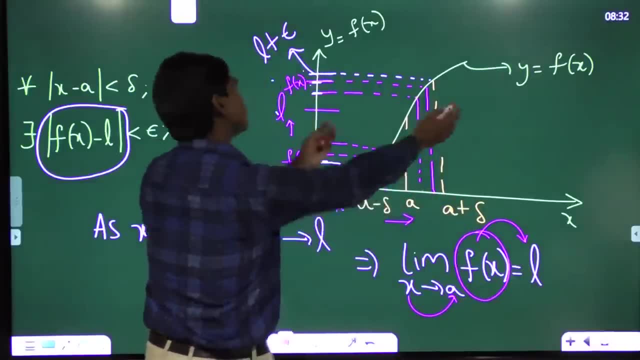 L. like this: whenever you are moving in the left neighborhood, this value f of x is moving to L from bottom to top. similarly, when you are in the right neighborhood, this value f of x is moving to L from bottom to top. 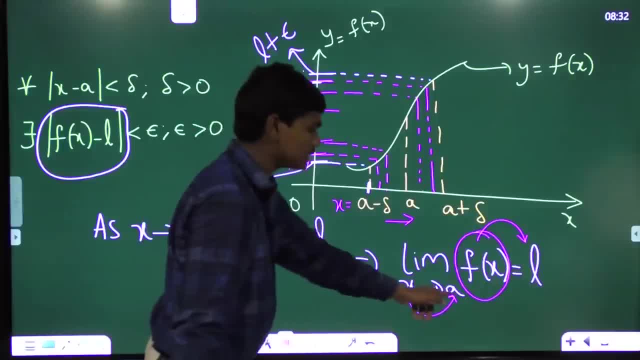 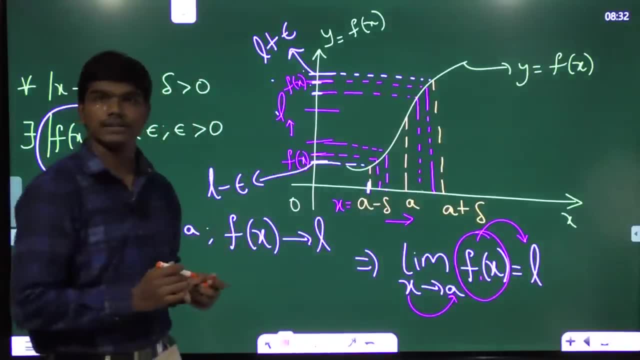 So this the mathematical form of this is: whenever this x is tending to a like, in this case this f of x will tend to L, which you have seen here. okay, so I hope now everything is clear under the concept of limit. so please take this diagram and write all these things. 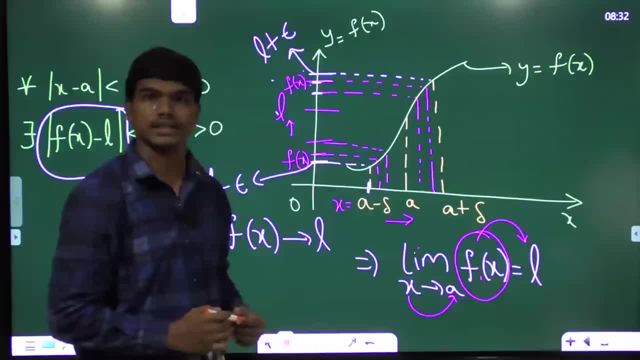 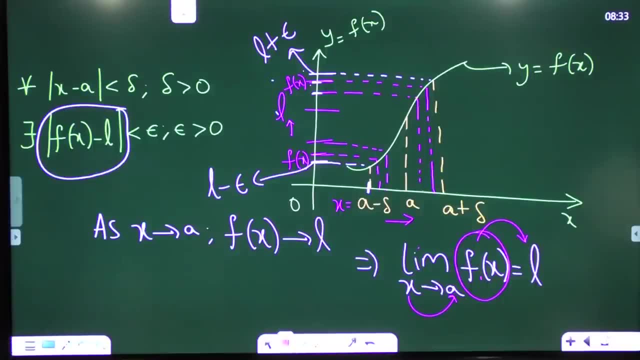 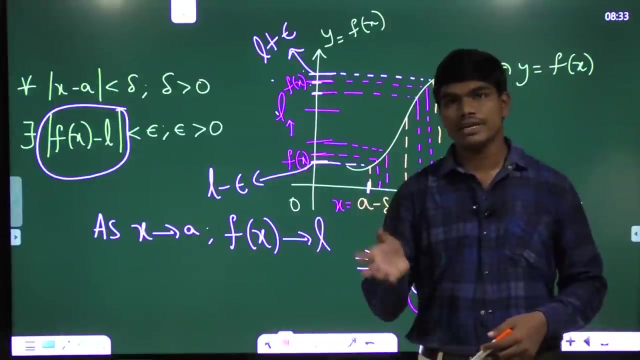 and please make a note, This mathematical notation of limit x tends to a f of x. okay, take a minute and please take this. I will give you time Coming to the course plan. after every lecture, we will be providing you with a PDF of the 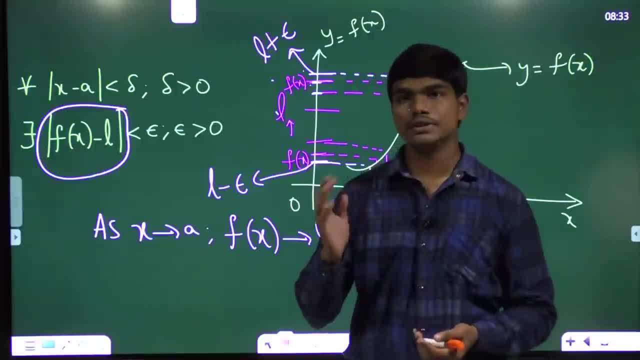 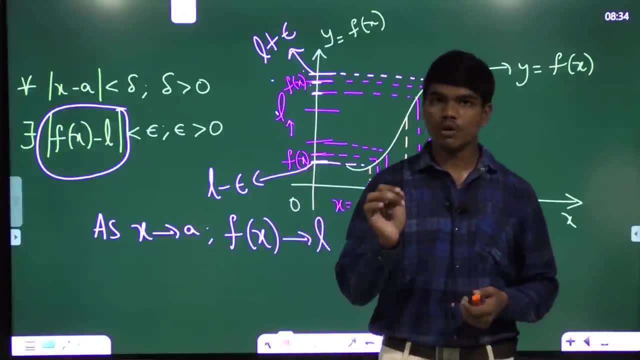 same what we have written, And also after completion of every individual module, we will look at some questions based on the topics that we covered, where I will be solving along with you, but I would recommend you to pause the video when I give you a question and try it by your own and later look for. 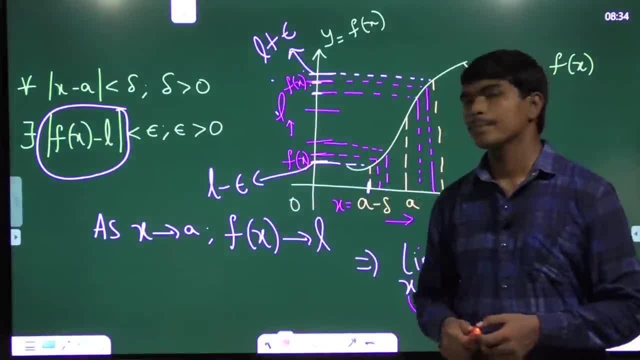 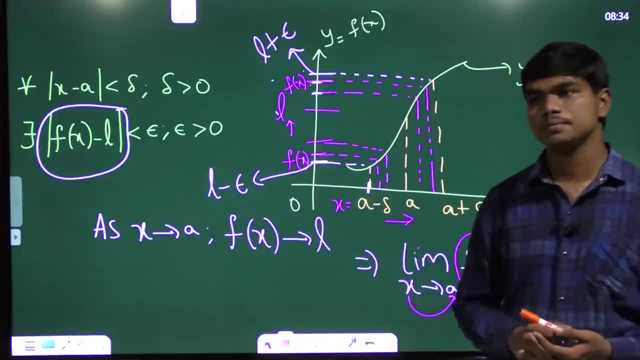 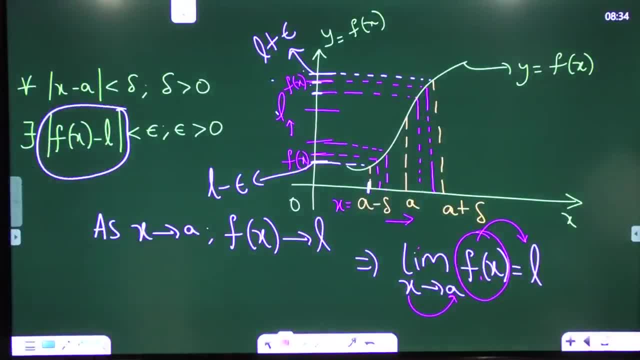 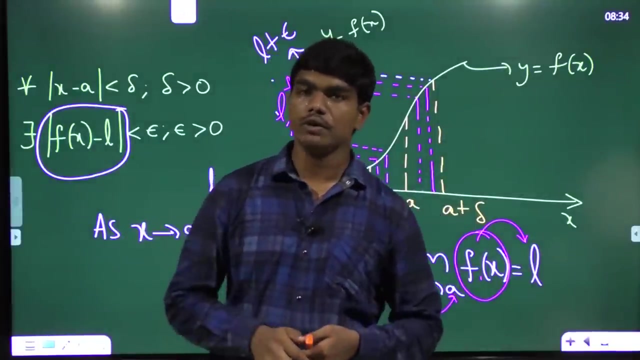 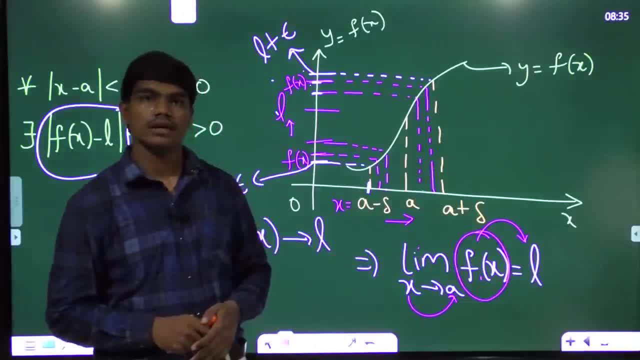 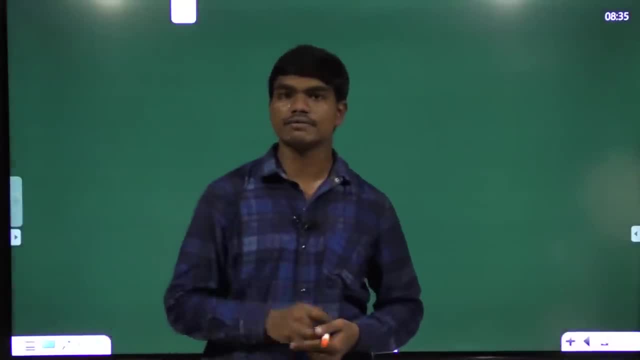 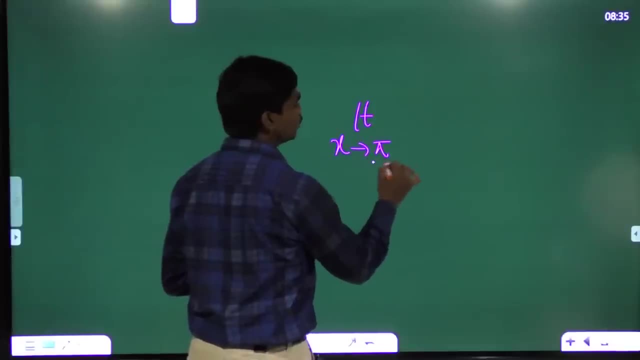 clear. so, now that you have got the definition of a limit, now, before proceeding further in limits, it's always how. it's always good to have knowledge on graphs when dealing with calculus, because, for, for example, if i ask you what's the value of limit, x tends to pi by 2 tan x. 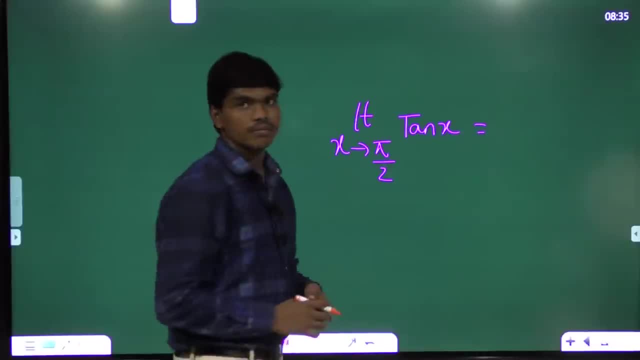 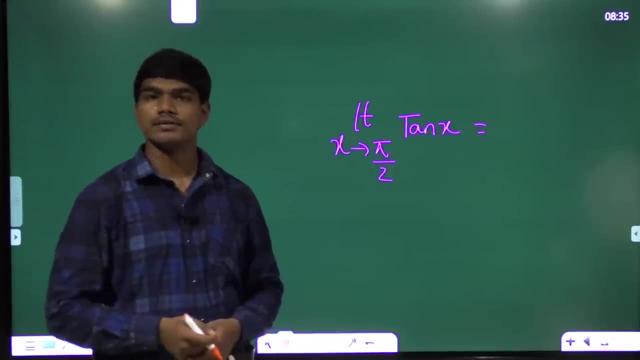 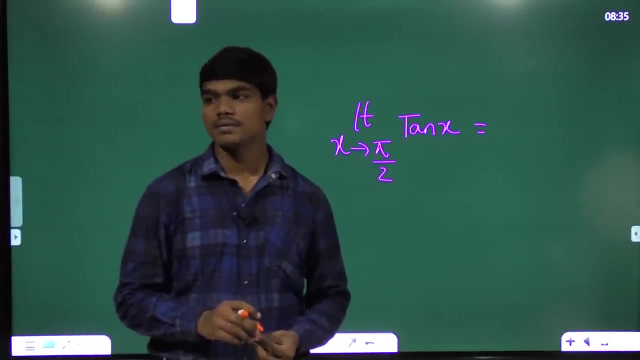 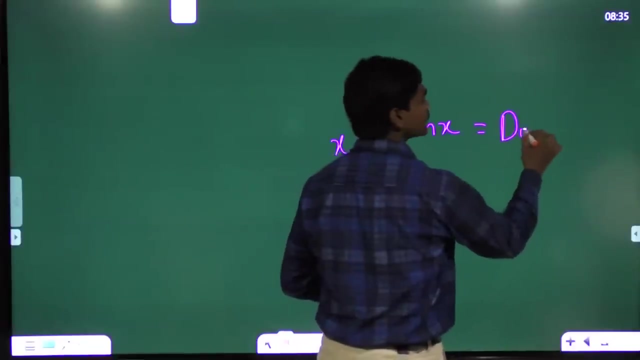 x. limit x tends to pi by 2, tan x. what could be the answer? i'll give you a moment. write it in the box. what could be the answer? infinity. okay, that's what some of you are thinking, but actually the answer is not infinity. the answer is: does not exist. 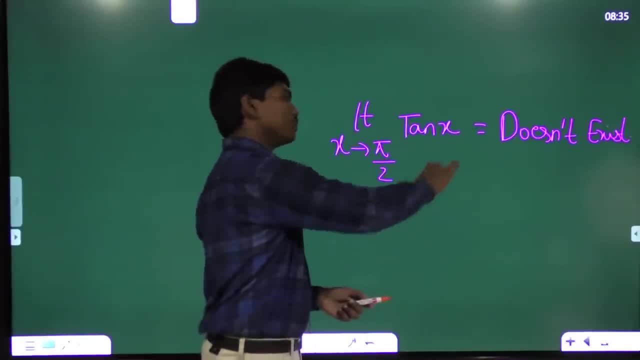 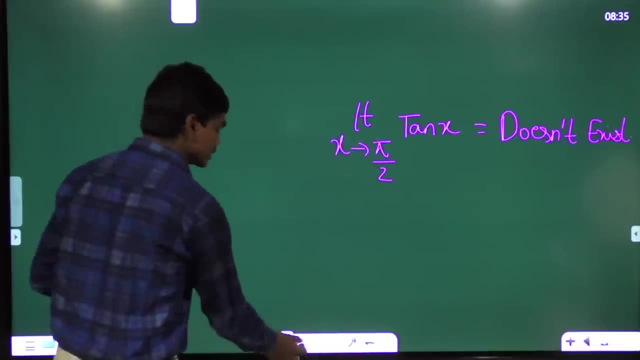 yeah, because it's. it's certain that you may think that it's infinity, because when you put x is equal to pi by 2, it's infinity. so that's what. that's the reason why you could tell infinity, but it's actually not so. we'll see why these situations are arising. okay, for the time being, i'm taking this don't. 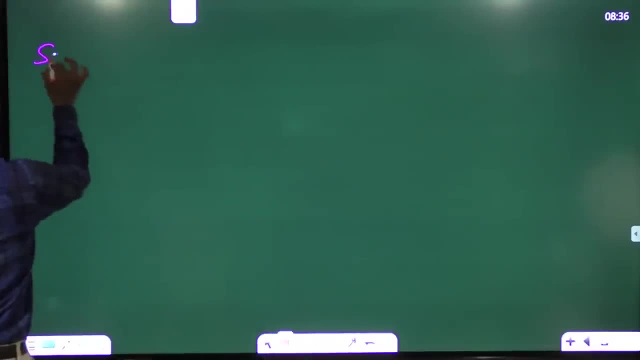 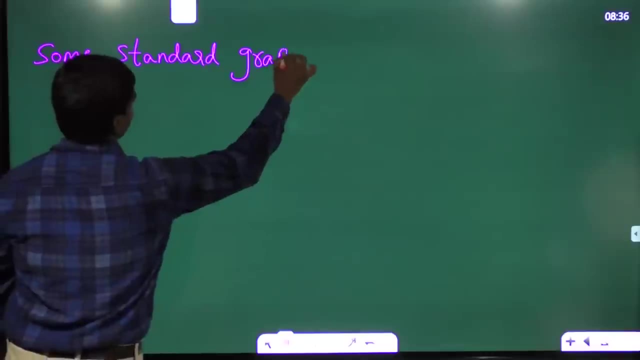 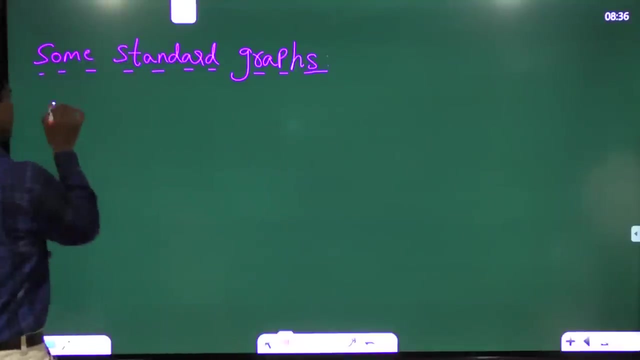 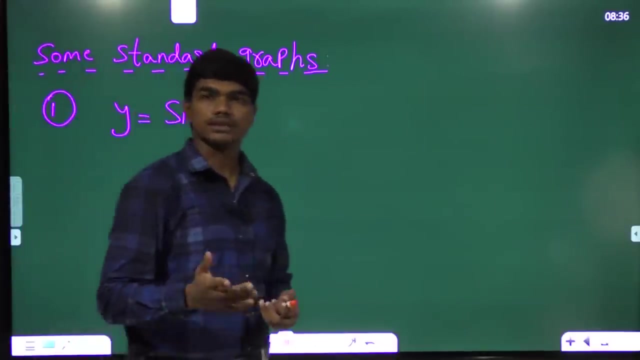 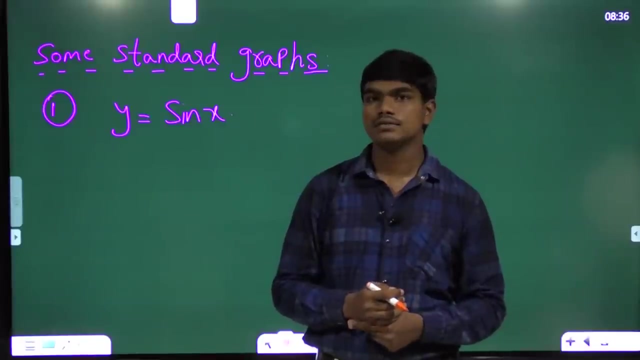 worry, i'll give it again when needed. so some important or some standard graphs. some standard graphs first, graph y is equal to sine x. i hope some of you know for this, just right before i draw the actual graph here. just right, okay. so if you have tried, now i will be drawing the actual graph. 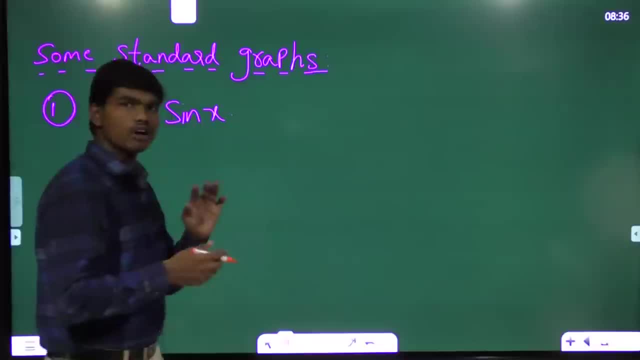 please check here now. first of all, for drawing graph of any function, there are certain few basic or certain key points, so let us first of all follow that. first of all, let us set up the axis. since this is a two variable function, i mean single variable function. let us plot example y. 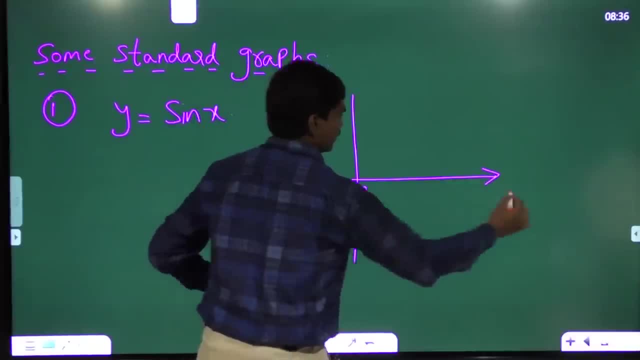 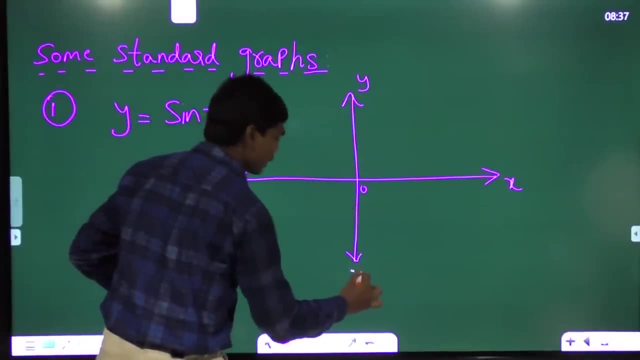 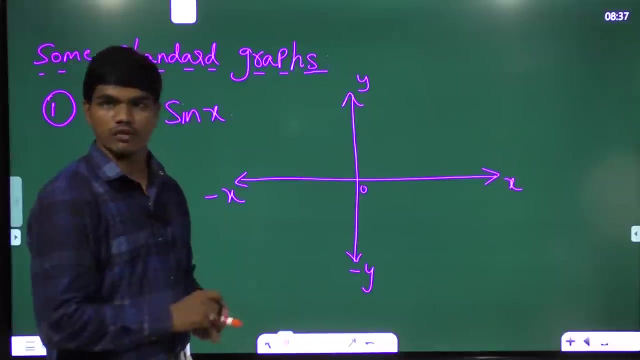 axis zero x. let me write this: minus x, y and minus y. now, after setting up the axis, alright, look for the maximum and minimum limits of this function means, whatever the value you put in place of x, this sine x doesn't go beyond plus one and doesn't come back beyond plus 1. okay, because you set up the. at x and instead of x you are setting up the y star value, and that isn't going to change an acting case. because let us see, at example x we're- oh, let's take the definition of that- square light and that's how you come over our left hand side and on afar. but there is this next: actually x can act as: 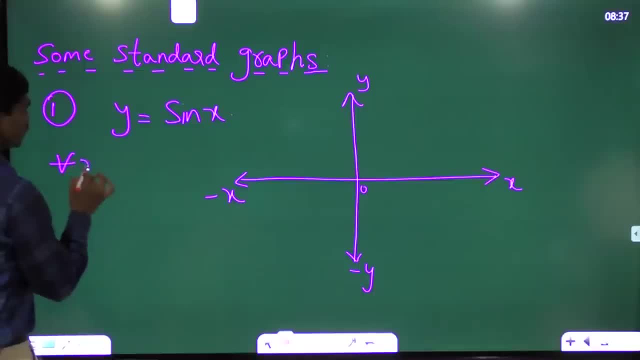 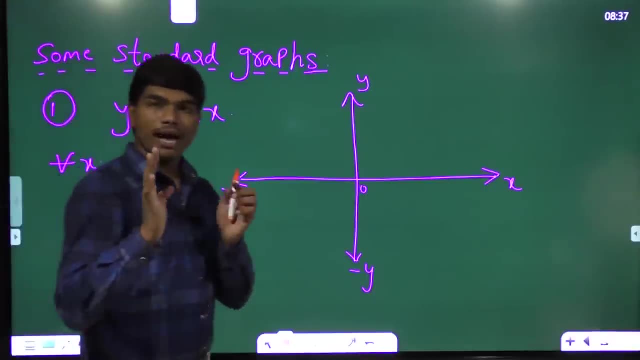 on minus 1.. So for all x, you know one thing: for all x, this minus 1 is less than or equal to sin. x is less than or equal to 1, which means if the maximum value of y is 1 and the 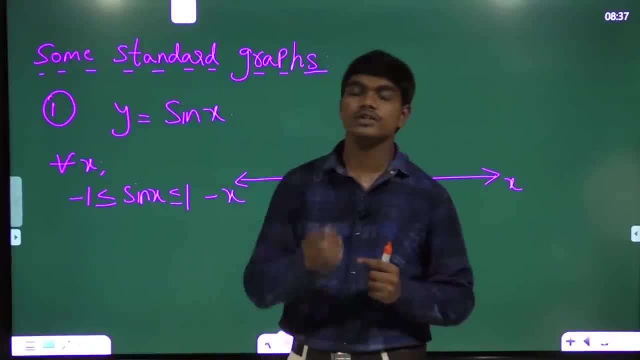 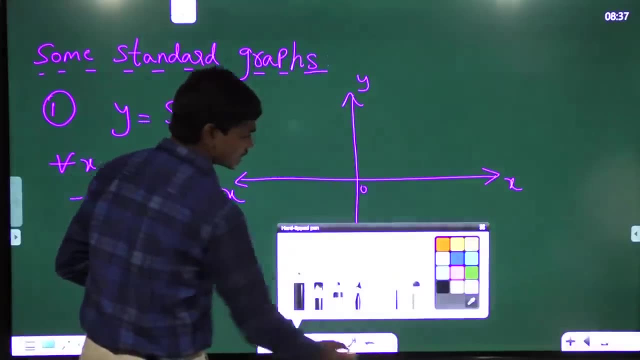 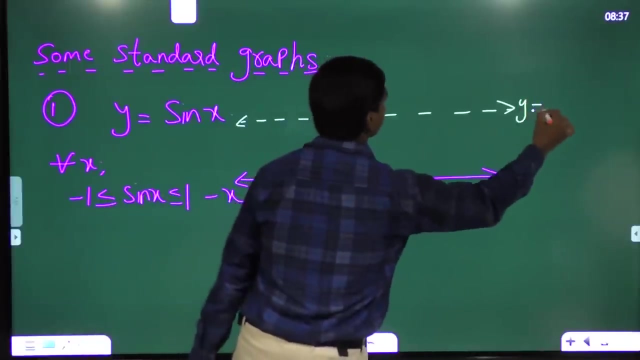 minimum value of y is minus 1.. So for the given function, which is here, your next second step is you need to look for maximum and minimum limits of the function. Now, if I try to draw the lines, y is equal to 1 and y is equal to minus 1, see here: this is: y is equal to 1. 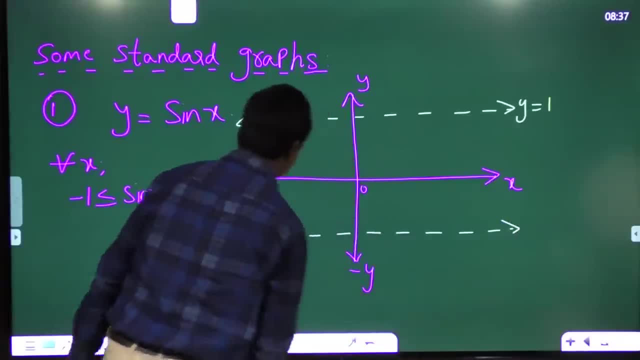 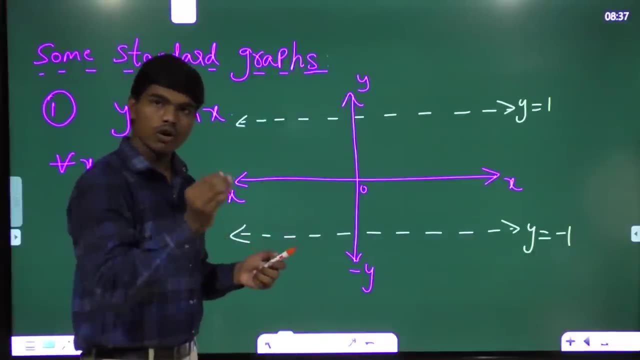 and this line could correspond to: y is equal to minus 1.. The reason for setting up these two lines is now: whatever the value you put in place of x, there is one thing very clear: the graph cannot go beyond these lines, correct. Now, whatever you draw, you should. 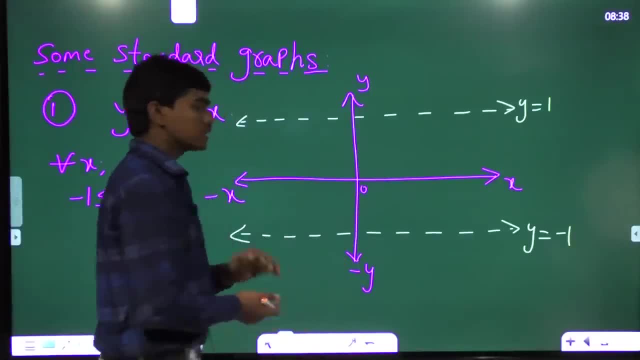 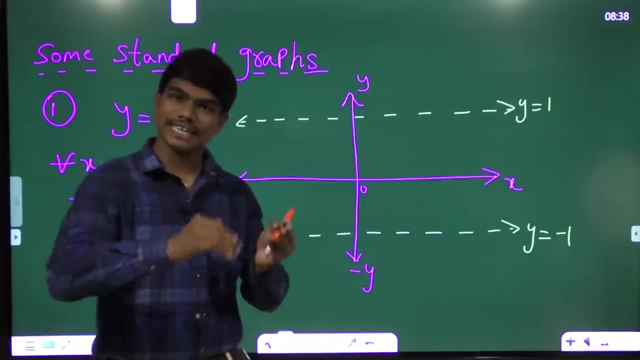 draw inside these green lines correct. Now the third step is you should look for the patterns means. for example, if you take sin x, the graph of sin x which is in between 0 to 2 pi is same as, again, from 2 pi to 4. 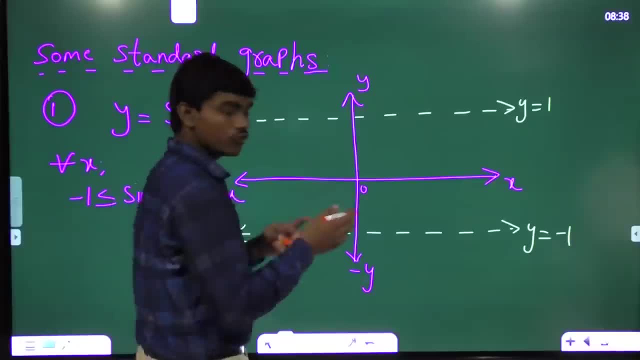 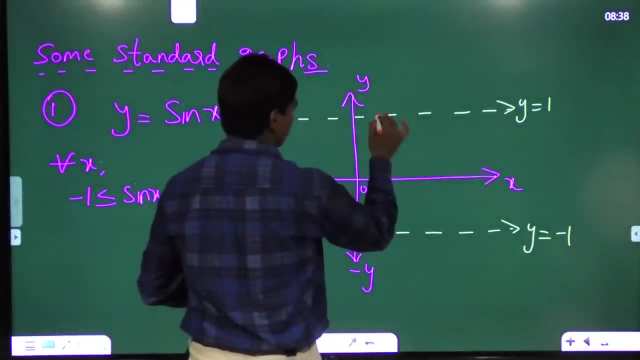 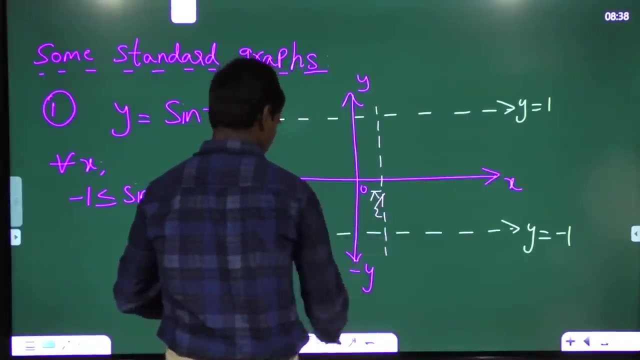 pi, because quadrants repeat, correct. So first of all, we should look for periodicity of the function. Now that let me do. now let me use this color. For example, if this is pi by 2, let me correct this a bit. 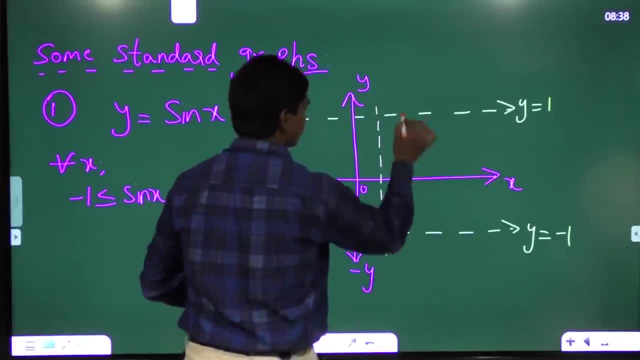 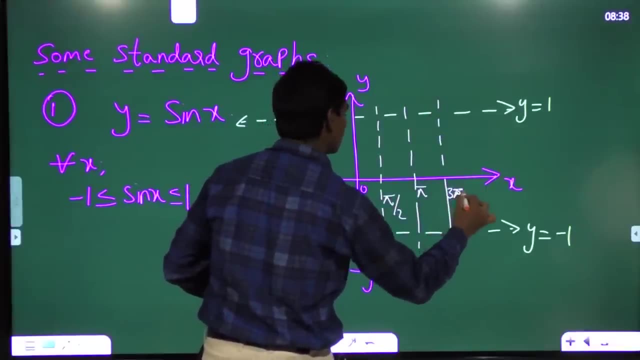 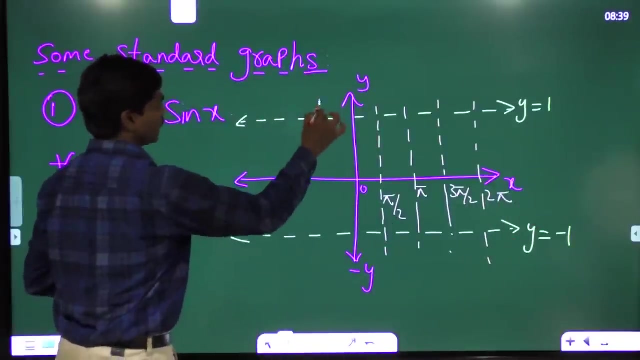 This is pi by 2. and let us suppose again: this is pi. and again, this is 3 pi by 2.. This is 3 pi by 2 and this is 2 pi. Similarly, if you come to this side, this is minus pi. 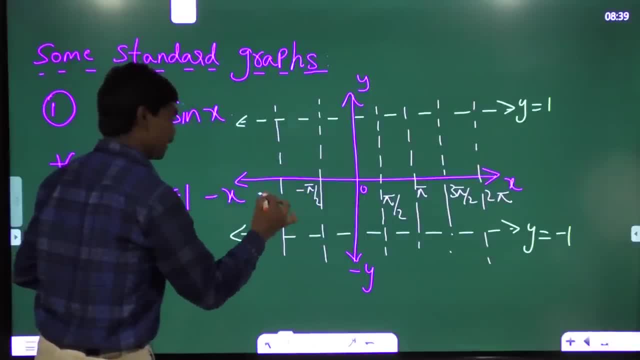 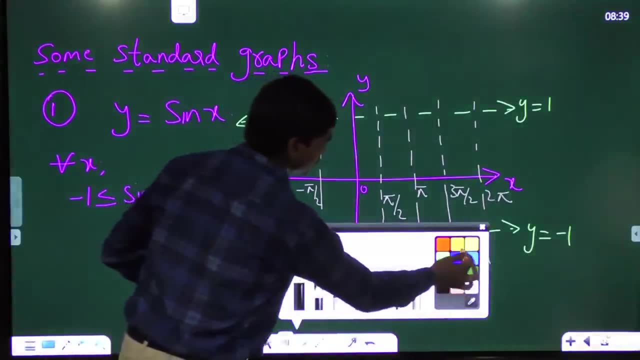 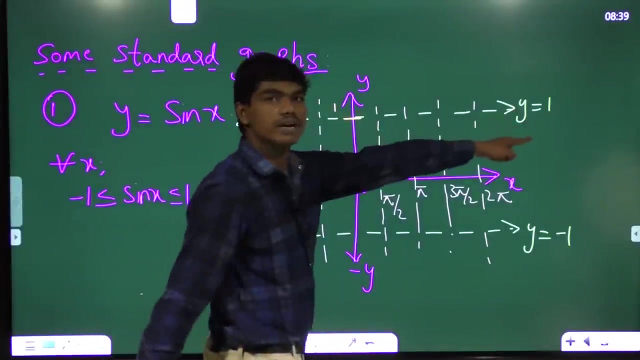 by 2.. Right, this is minus one, and of course i'm stopping this because you'll get one full loop here on the right hand side. okay, now, if you try to draw the graph of this, you need to check the points where this function is getting maximum value. you know this value is one because you set up this line. y is 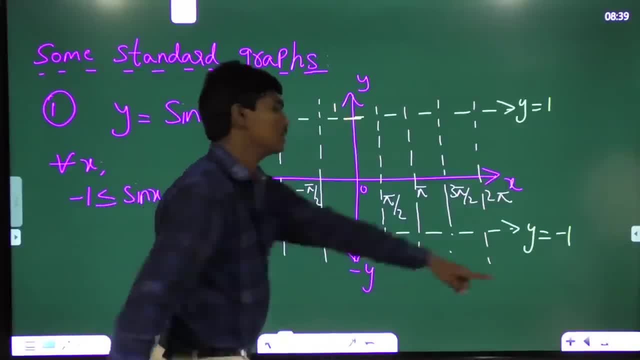 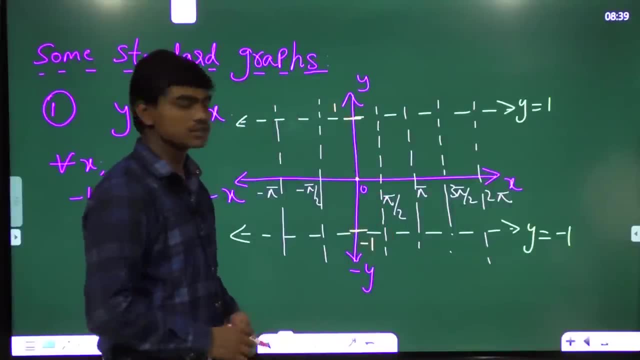 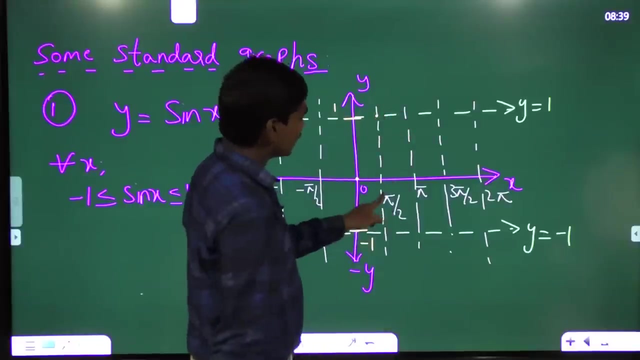 equal to one. similarly, you know this value is minus one, this is y is equal to minus one. now you know sine zero is zero. okay, we'll see why sine zero is zero after two lectures, okay, when i deal some more advanced topics in calculus. so this is zero. so sine pi by two is one, means at sine 90 the. 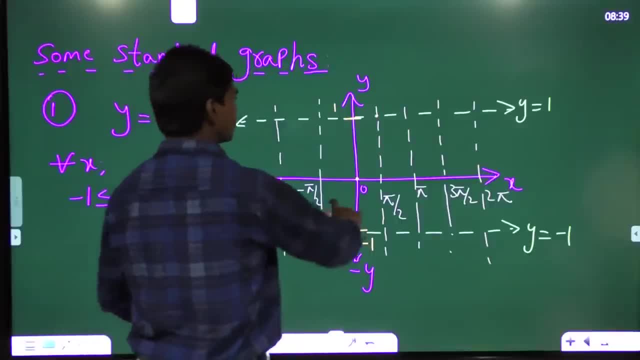 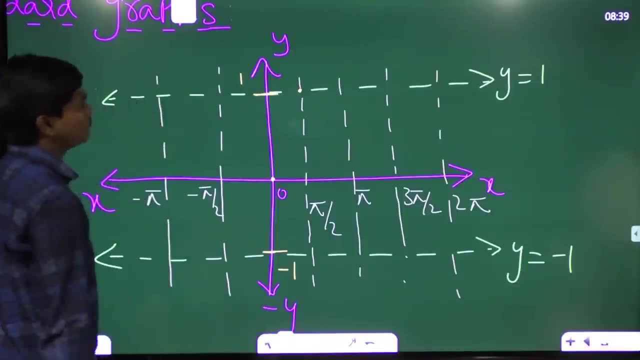 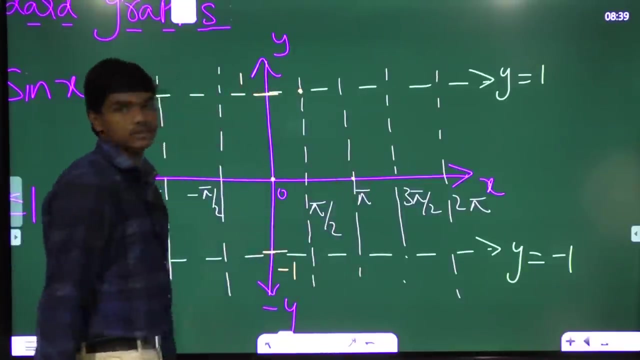 value of this is one for the time being. let me enlarge this graph for you so that you can have a clear understanding. is that better? now clear? okay, so now this is sine x, which is one here. next, the value of sine pi is again zero, because sine 180 is again zero. now sine 270: 3 pi by 2 is 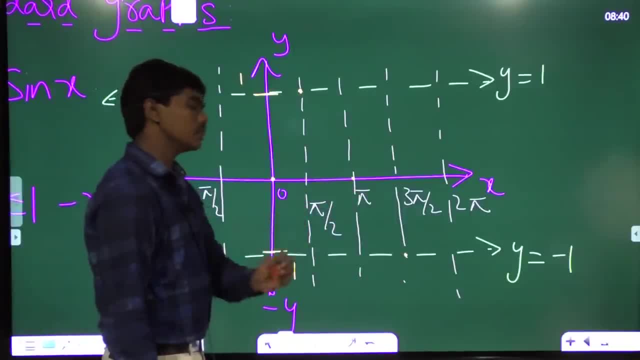 again minus one, because 3 by 2 falls in the third quadrant and you know sine is negative in the third quadrant. and now again, sine 2 pi is same as sine 0. this is here. so if you try to draw the graph of this or again, 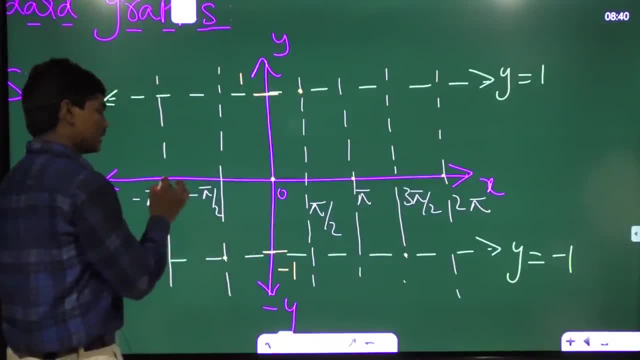 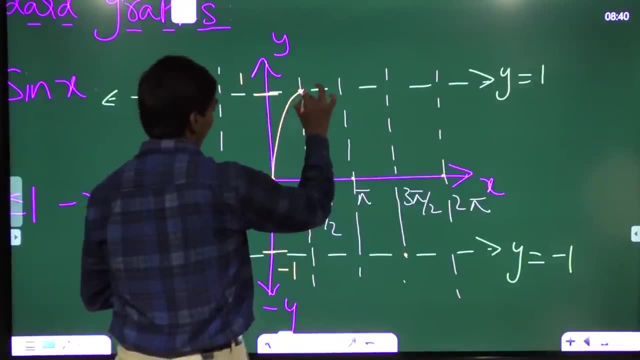 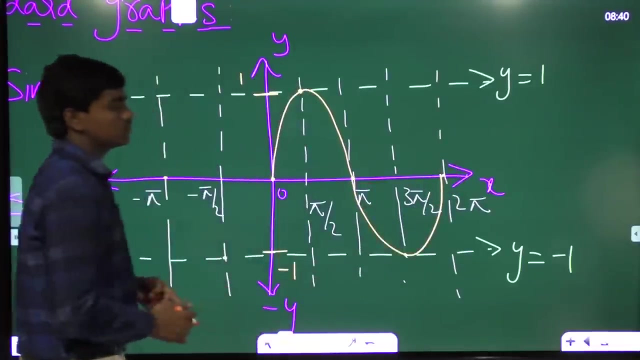 sine minus pi by 2. you know sine of minus theta is minus sine theta and similarly this is 0. so if you try to connect all these points to the smooth curve, our actual plot could look something like this: this is one full loop of sine x. so this is the standard way which you adopt in drawing. 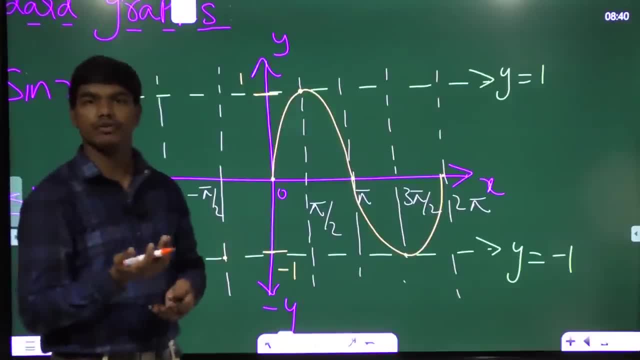 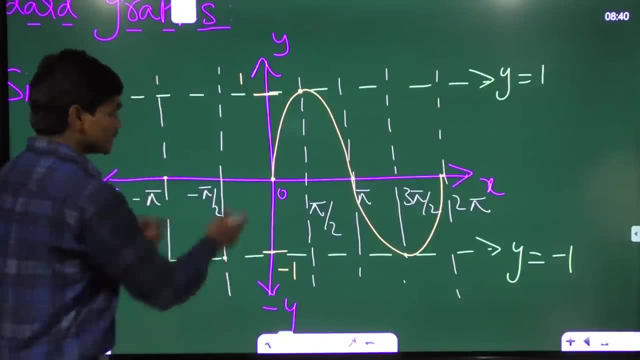 any graphs, because this is a sine x function and this is a simple function which many of you could know. but if i ask you to draw the graph of x into sine x, what could you do? could you give a tie for that? tie it later. so this is the three general standards that we purchase, that we follow to draw. 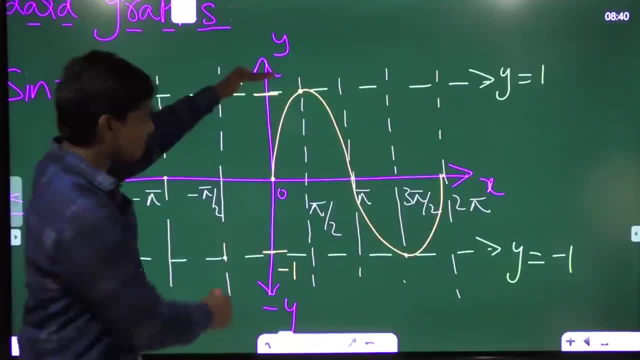 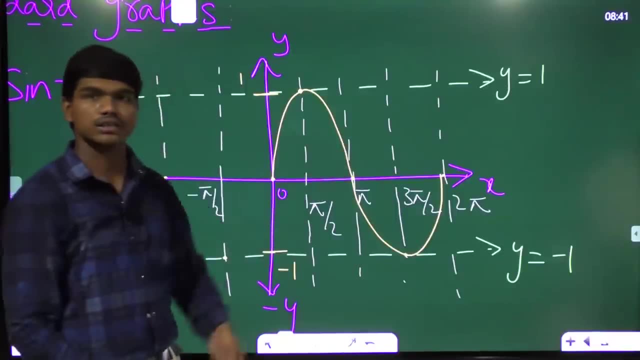 any graphs. first of all, setting up the axis. second thing: look for the maximum and minimum limits of the function. which is the maximum and minimum of the function? basically, third limit is look, i mean. third key point is to look for the patterns. if there are any repeating patterns. let me join these points also with my smooth curve. 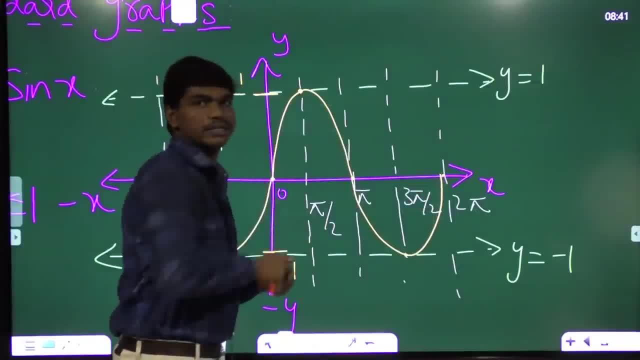 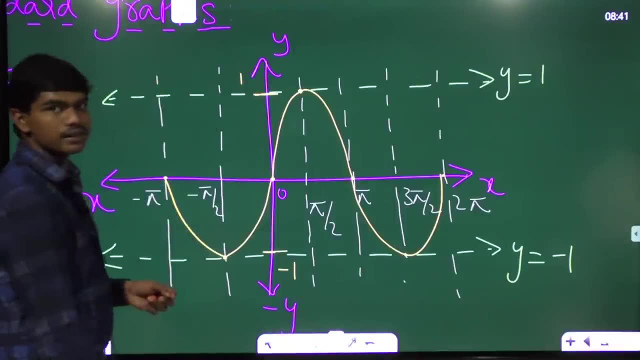 so basically, this loop, which is in between 0 to 2 pi, keeps on repeating. so this is how graph of sine x looks like. okay, now i think it's visible for you clearly. take it now. suppose if i ask you to minus 3 by 2, this loop would have gone up. 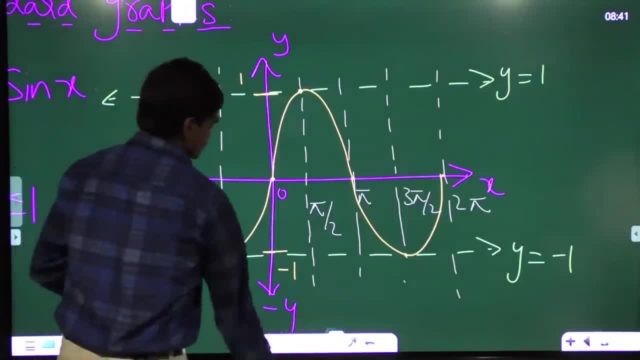 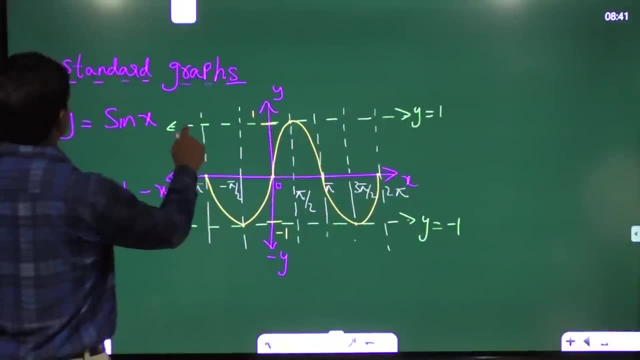 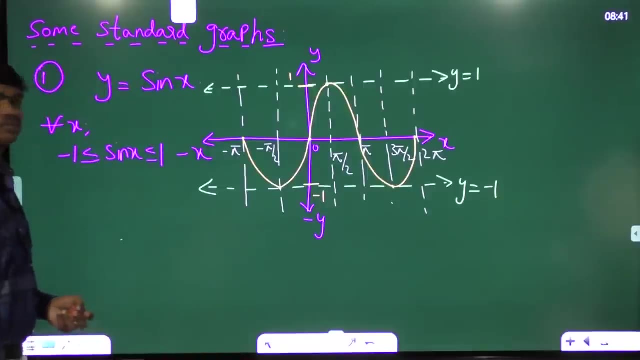 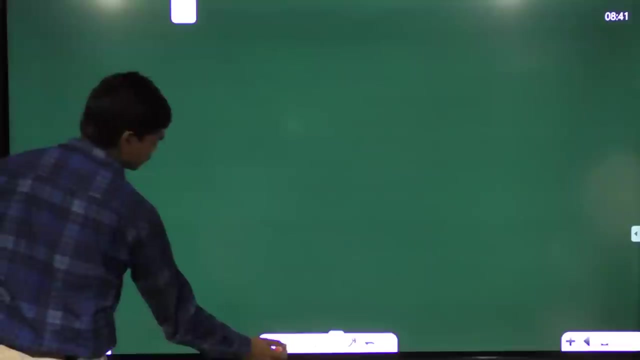 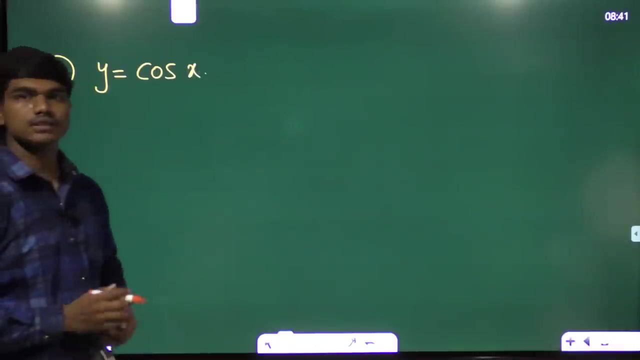 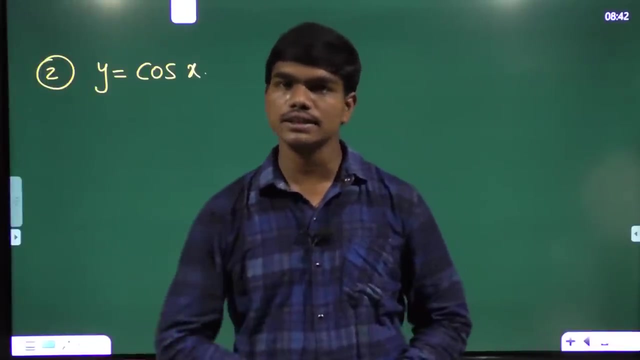 3 by 2. so okay, now second graph. sorry for this second job. y is equal to cos x. Could you do a graph for this? Why is it equal to causes? How does it look like? Very much similar to sine x, but shifted away 90 degrees towards negative x-axis. 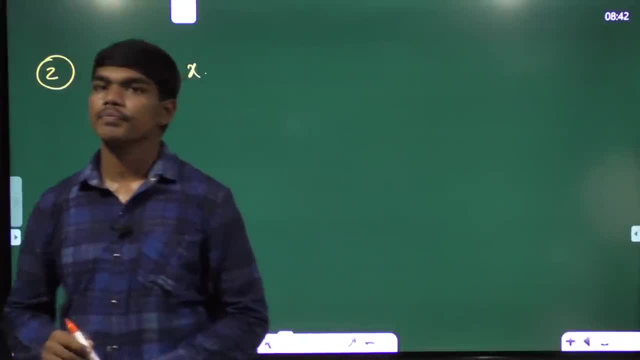 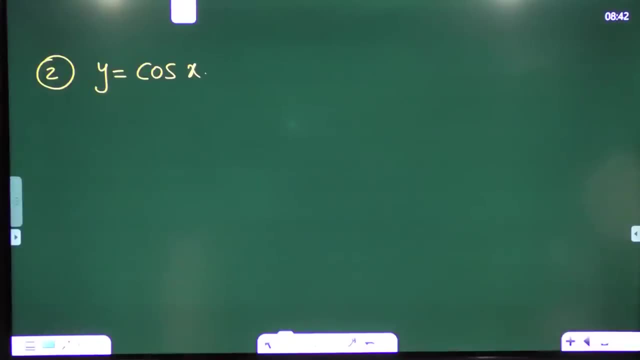 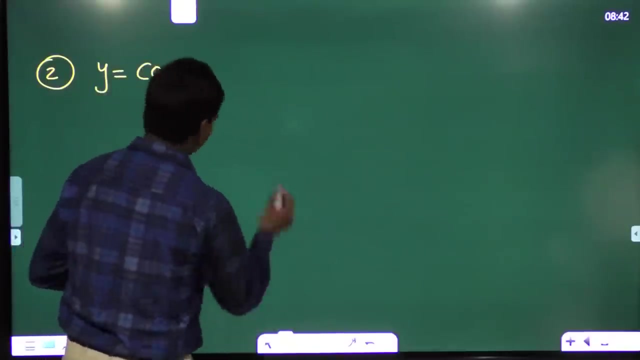 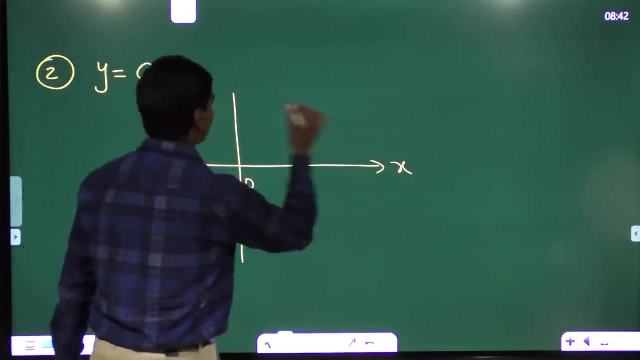 Please try to do this graph in a minute. I suppose that you have done this, so let me give a quick figure of this graph. Setting up the axis is the first step of my minus x, x, y and minus y Again, setting up the limits. 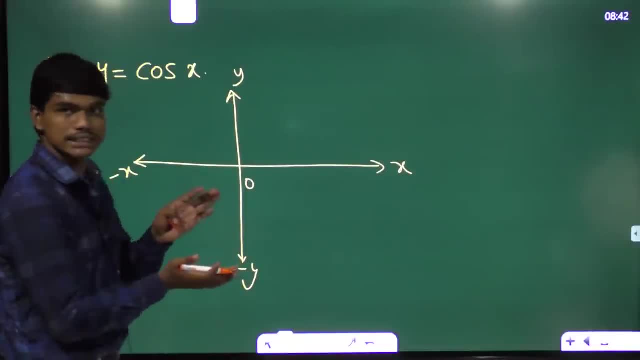 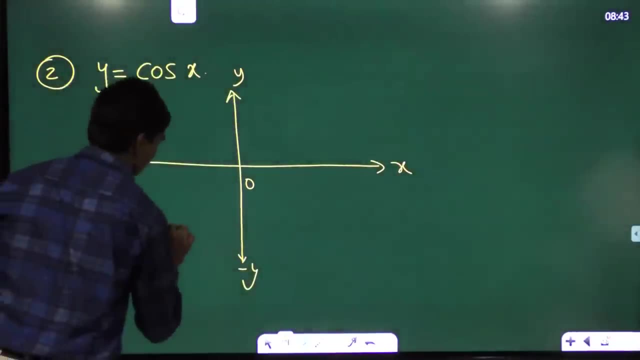 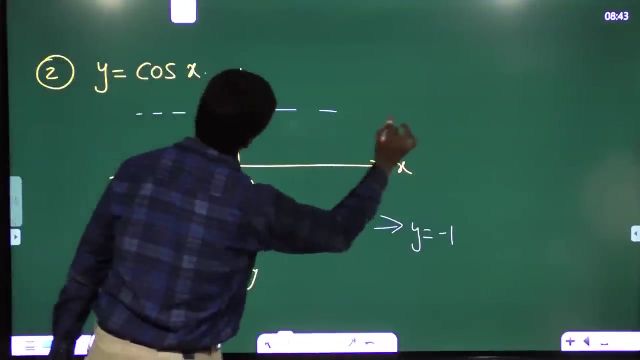 across. it's also, whatever the value of the x cause, x always lies in between minus 1 and 1.. Let me write that Minus y is equal to minus 1 and 1.. Now again, look for the patterns. 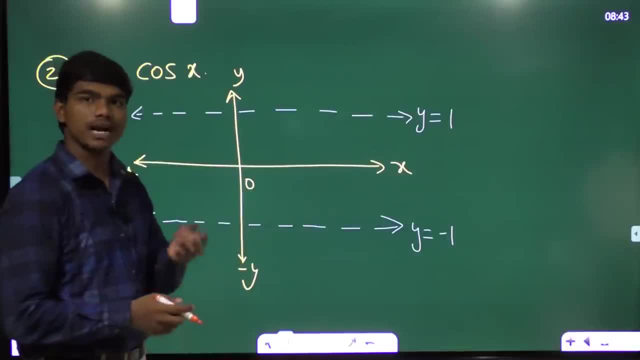 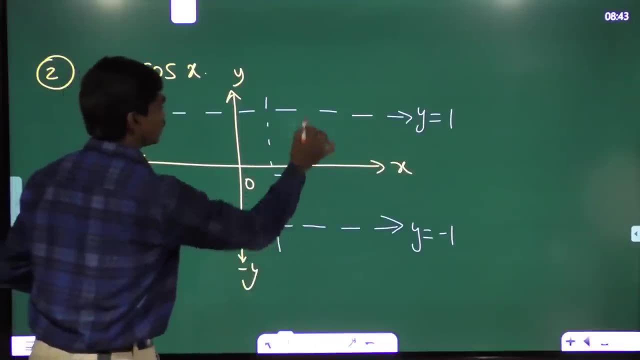 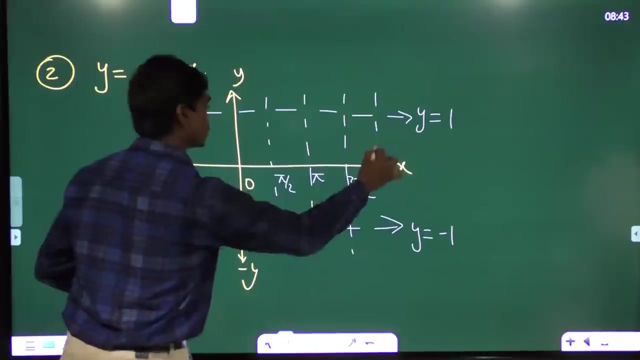 and again. cause is also a periodic function with period 2. pi. It means after every 2 pi interval it gets repeated. Now let me split this interval Again in a similar way: pi by 2.. Pi, pi by 2, and of course 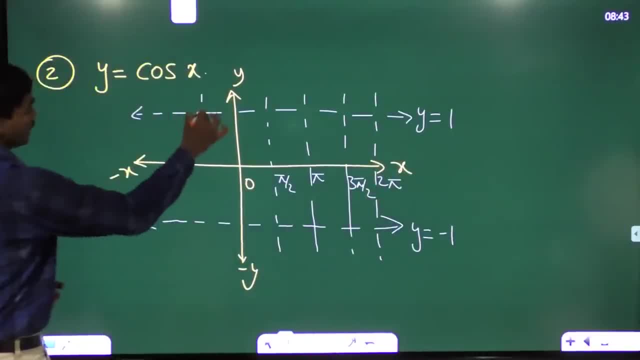 this could be somewhere here, which is 2 pi. Similarly, on the left-hand side, this is minus pi by 2, and this is minus pi. We intend to draw here because one loop is sufficient, because loops get repeated as many times. 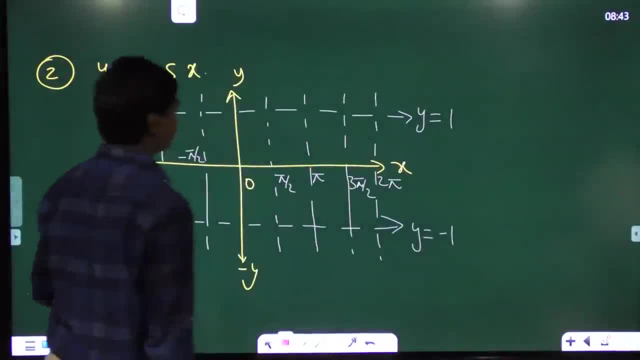 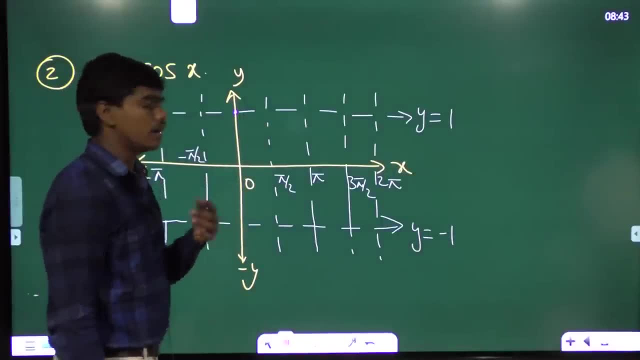 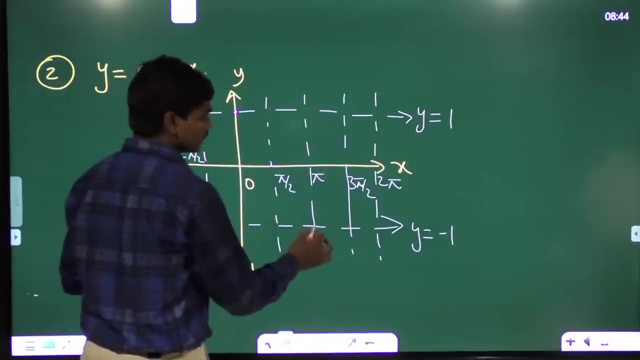 So now, what's the value of cos 0? 1. 1.. We will see again why cos 0 is also 1 in the next lecture. Cos 90 is 0.. What about cos pi? This is minus 1, because in the third quadrant, I mean in both second and third. 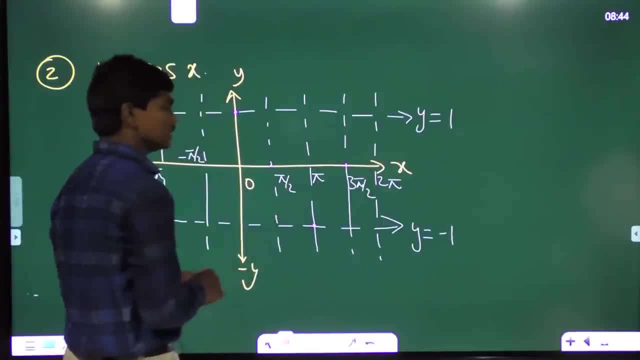 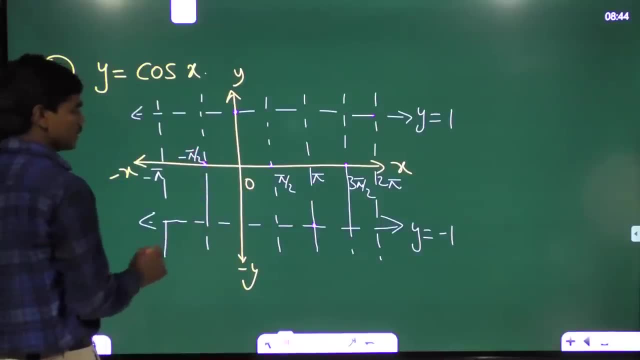 quadrants, cos is negative. At 3 pi by 2, again this is 0.. So now again at 2 pi, this is 1.. Similarly here this is cos minus 90 is 0, and again this is minus 1.. So now if 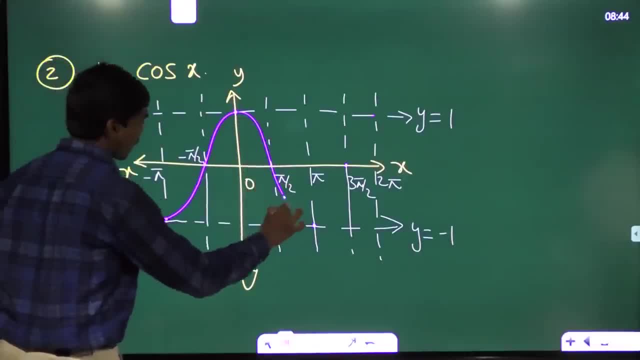 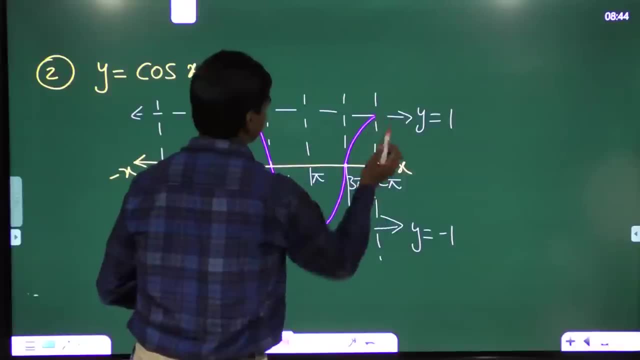 you try to join these points with a smooth curve, something like this: And this loop which is here is a complete loop and that gets repeated. You may extend this further, No issues. So this is how graph of y is equal to cos x looks like. Now one important graph. 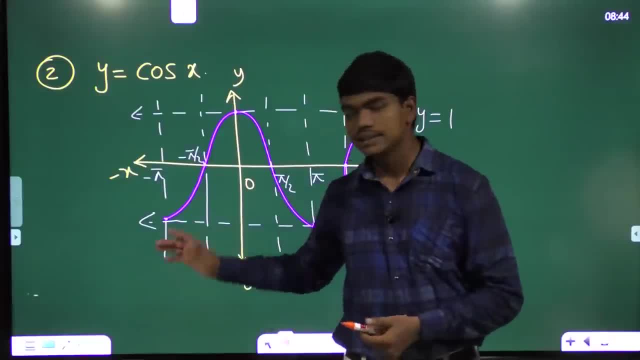 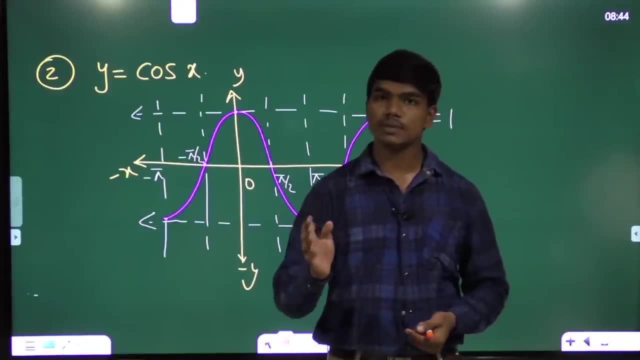 that we talked about tan x graph And that's the reason why we are discussing sin x graph and cos x graph to dot tan x. Now, when I dot tan x graph, you yourself will understand why limit extends to pi by 2. tan x is not infinite. 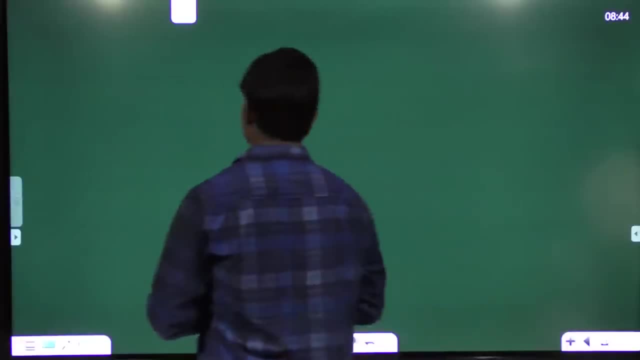 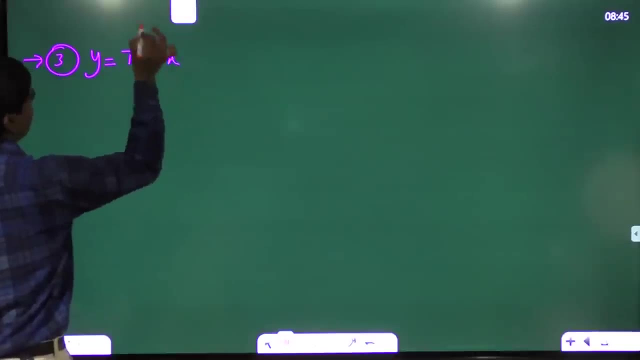 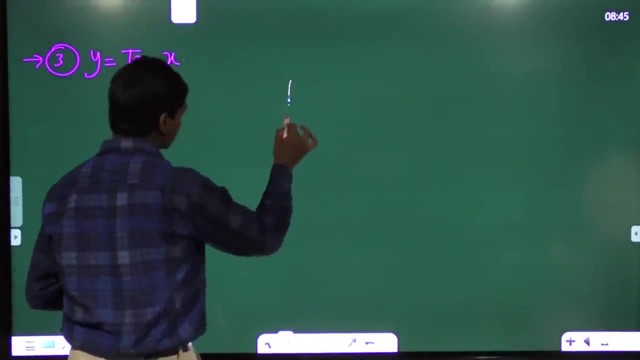 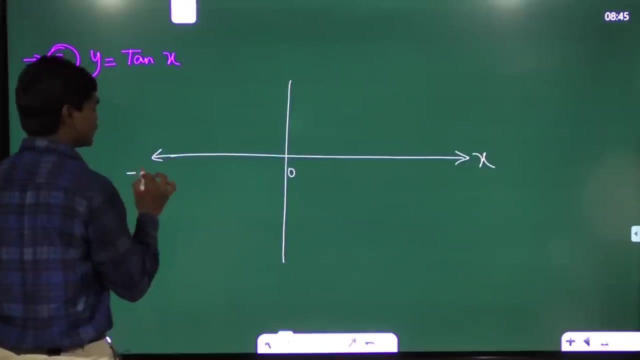 And why it does not exist. Correct, See here. Third graph: y is equal to tan x. Now again, let us follow the standard procedure that we have First of all set up the axis. So if we are setting up the axis x, 0, minus x, this is y and this is minus y. Now let's 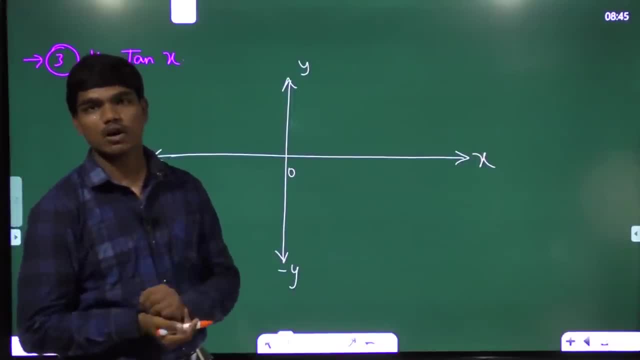 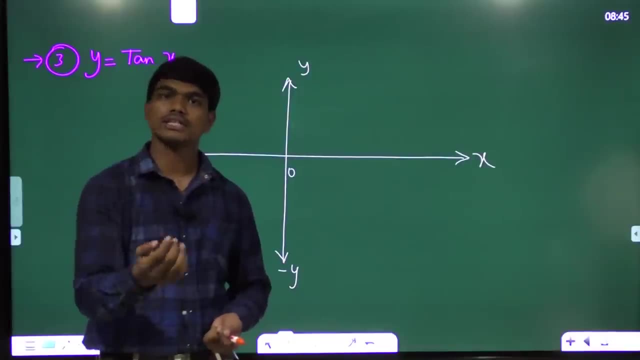 set up the axis Now. second thing is look for the maximum and minimum value of the function. Now you know tan x has infinity as the maximum value, Because when cos x is 0, since sin x by cos x is tan x, and when cos x is 0, your answer goes to infinity. So let us suppose 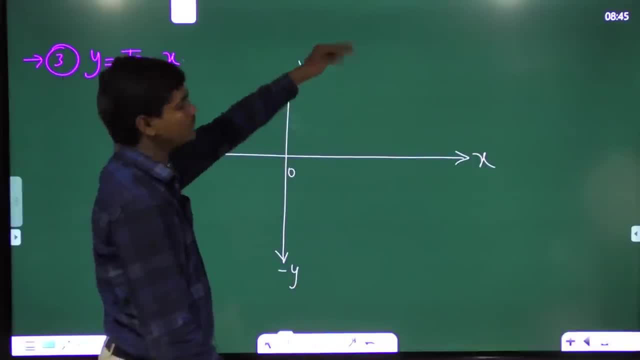 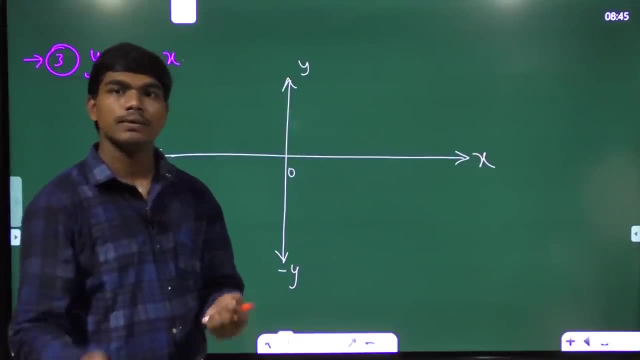 we don't have any horizontal lines this time to dot, because limits are infinity and minus infinity. Now we should look for patterns. Since sin x and cos x are repeating after every two pi intervals, tan x also repeats after every pi intervals. Okay, So let me. 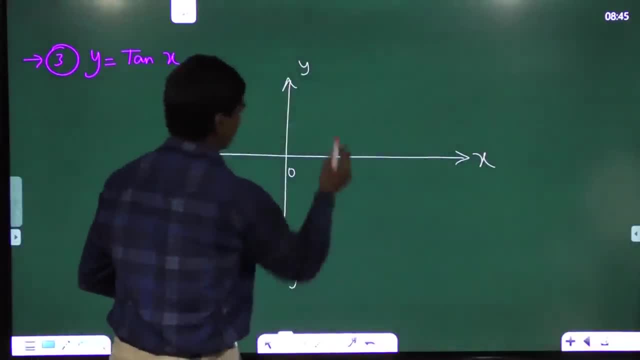 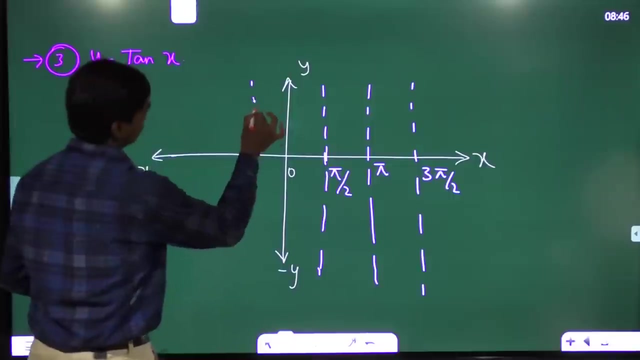 try to draw that. First of all, let me draw this partition lines. This is pi by 2.. Let me write it a bit clearly. This is pi by 2.. And this is pi, And this is 3 pi by 2.. And 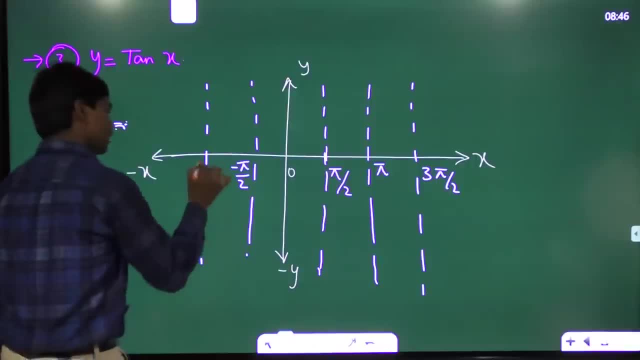 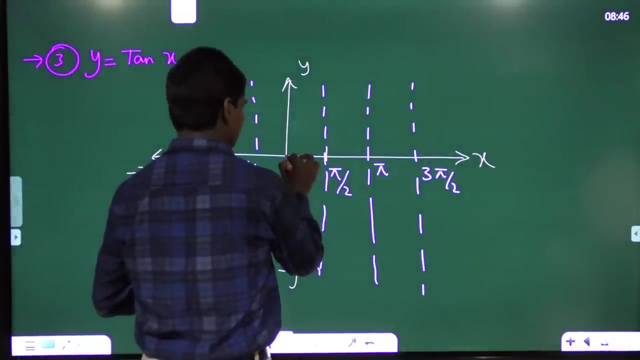 this is minus pi by 2. And this is sorry for this. And this is minus pi, Correct. Now if you see what's the value of tan 0?, Let me use a different color so you could appreciate the things Now. for example, 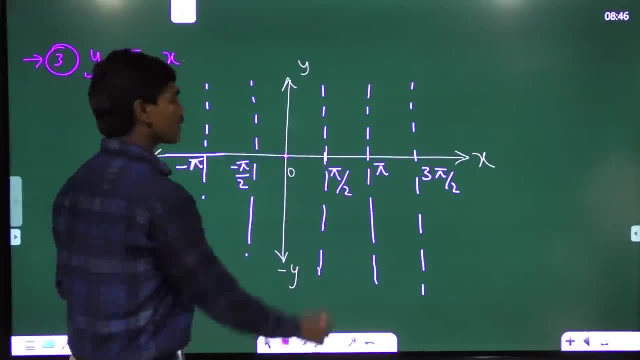 if you see, this is tan 0,, which is 0.. Correct, Now tan 90 will go to infinity, as you know, And similarly, tan minus 90 will also go to minus infinity. Okay, So which means, if I try to draw the graph of these functions, I could get something. 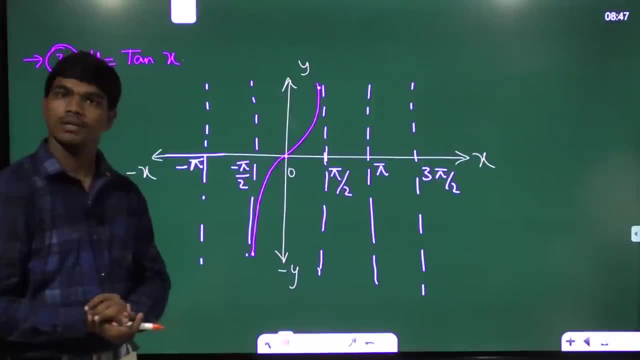 like this: In between minus pi by 2 to pi by 2. Means our interval of pi Correct. Now what happens after pi by 2? Or to the later of pi by 2? Minus pi by 2? This pattern gets. 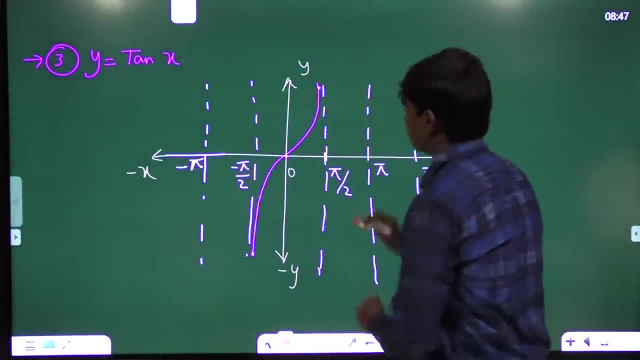 repeated: Okay. So if I repeat this pattern, which is from minus pi by 2 to pi by 2, here you could clearly see one thing: The graph looks something like this: Okay, And of course here it looks something like this again: 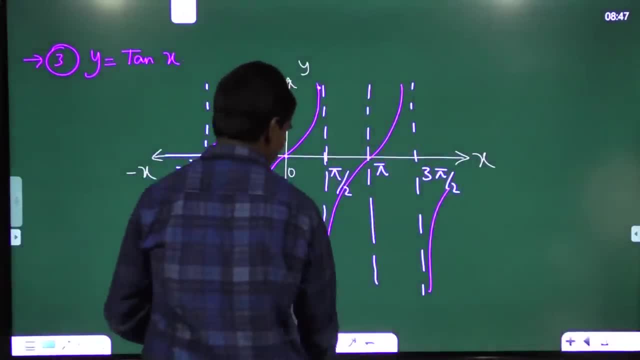 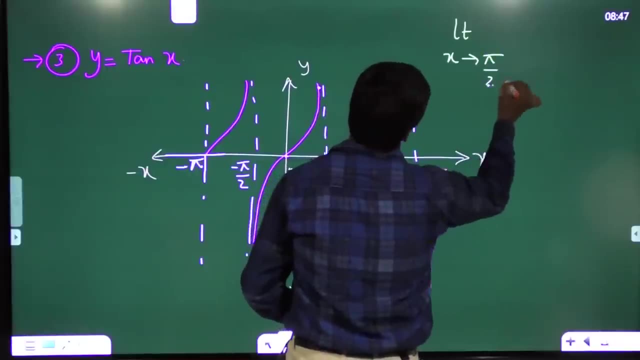 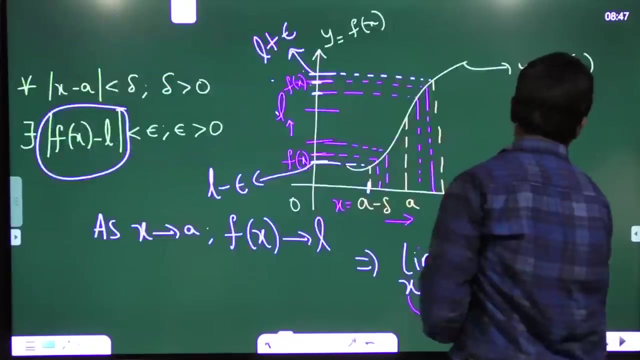 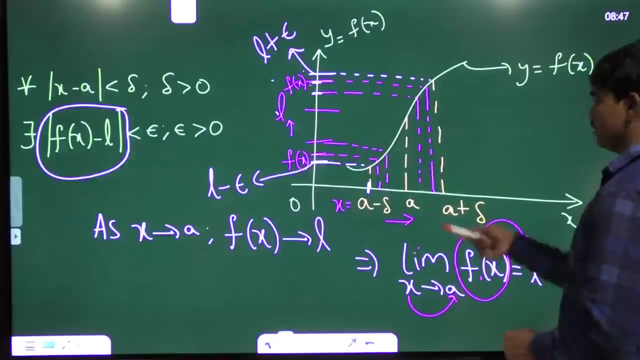 Let's look Now if you see clearly what's the question that we were talking about initially. Limit x tends to pi by 2?? Tan x- Correct. Now if you see the definition of limit that we were talking a few lectures ago, for example. yeah, here Here I have written one thing. 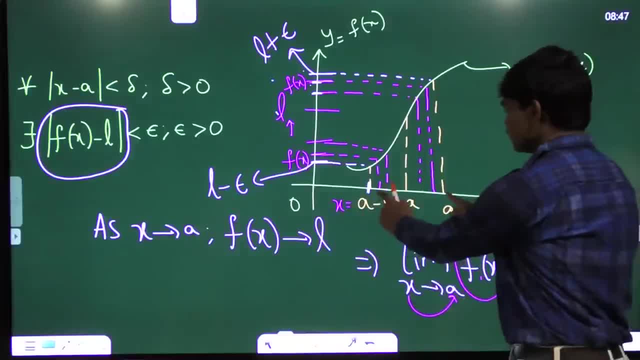 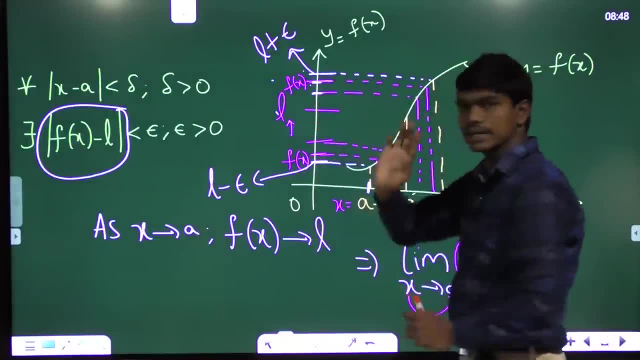 as x tends to a, f of x should tend to l. That's what you have seen here. Okay, So you have seen, whenever this x, which is here, is tending towards this a, this f of x, which is here, is also tending towards this l. Correct, Now, when I am writing, this definition did. 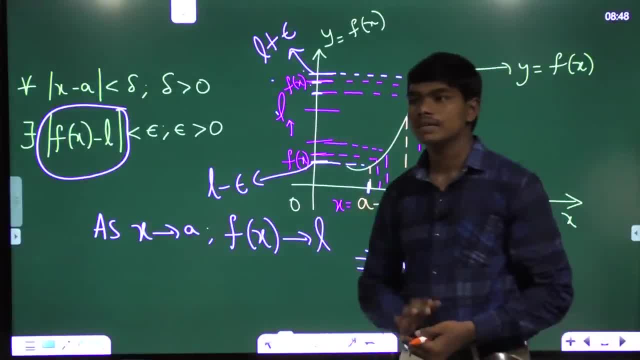 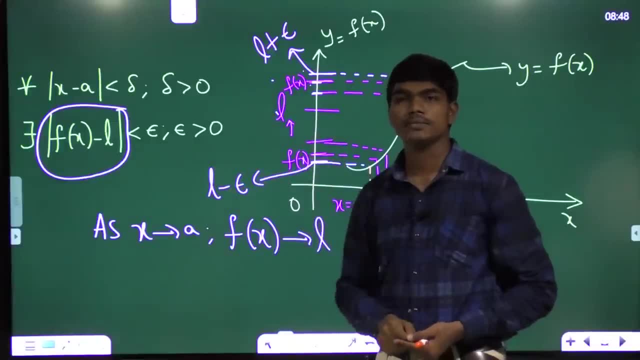 I mention you x should tend to a from left-hand side or right-hand side. Did I mention that? No, I didn't mention. I just told you x should tend to a, but I didn't mention the direction in which it should tend to a. Correct. So which means if you tend towards a, either. 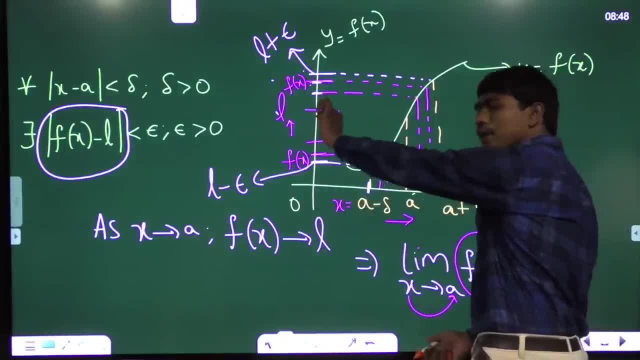 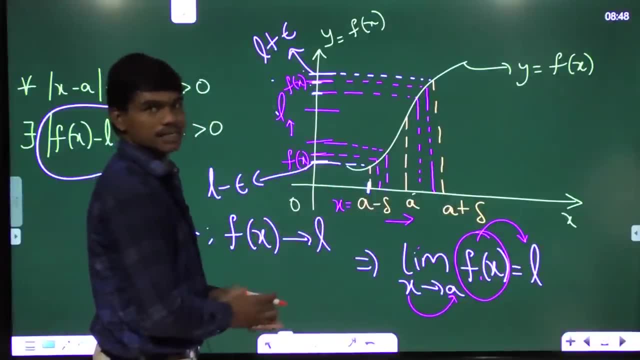 from left-hand side or from right-hand side, you should get the same value, l, which is happening in this case, actually Correct. So that's why the concept of left-hand limit and right-hand limit comes actually, If you are tending towards a, either from left-hand, 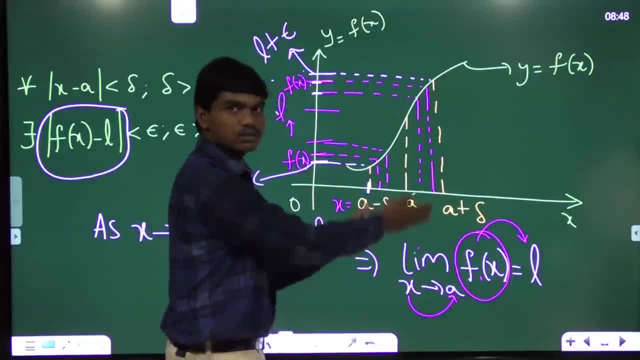 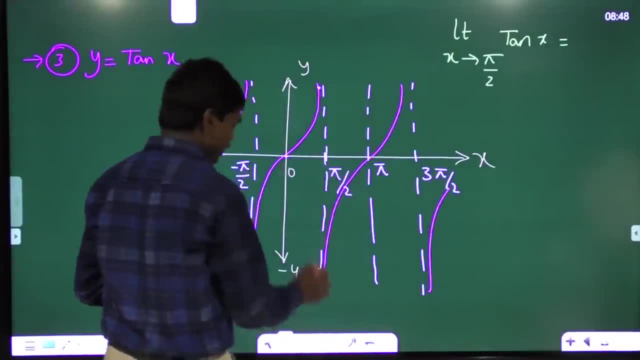 side, which means x is in left neighborhood, or if x is in right neighborhood, both are same. So, going back to our things here, this is: y is equal to tan x. Now, at pi by 2, at x is equal to pi by 2,. if you see, this is the point of interest- x is equal to pi by. 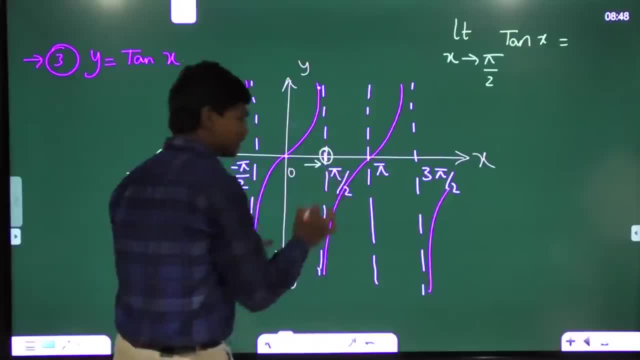 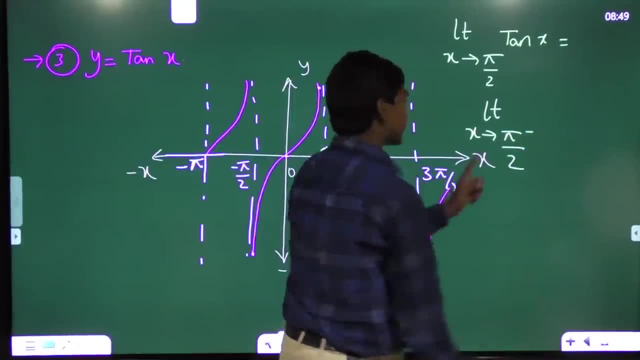 2. Correct. So as a left-hand side means limit, x tends to pi by 2 minus. please make a note. this is pi by 2 minus and not minus pi by 2.. Okay, Please make a note of that. So when x is tending, 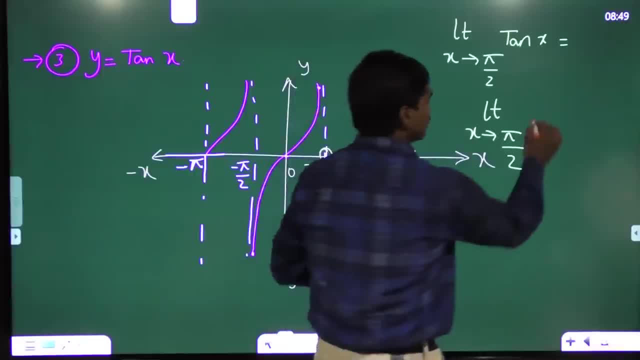 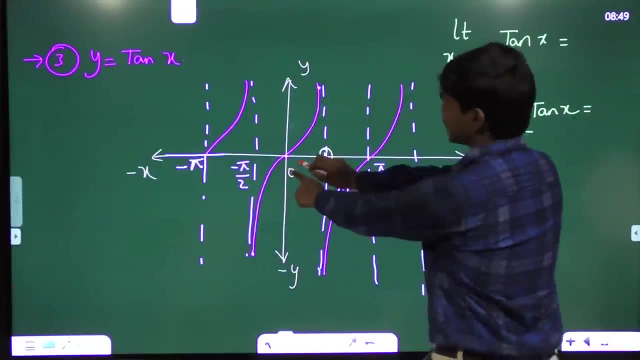 to pi by 2 from left-hand side means x is tending to pi by 2, minus the value of this tan x. When x is tending to pi by 2 from left-hand side, this tan x is tending to. you can see. 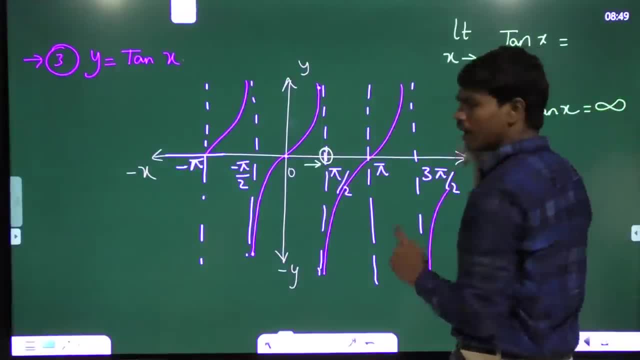 the graph. here, the tan x is tending to infinite, Of course, which is plus Correct. Now, similarly, if I talk about limit x from right-hand side, when I am talking about either from left-hand side, l is equal to pi by 2 left-hand side. Therefore, x is tending to pi by 2 from right-hand. 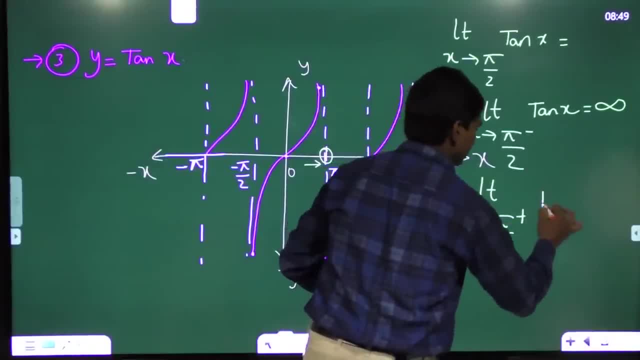 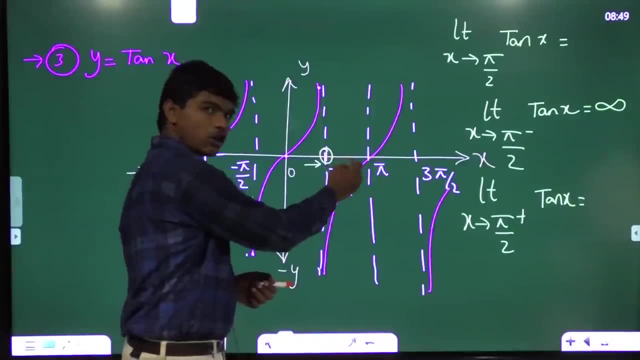 tends to pi by 2 plus tan x Means x is tending to pi by 2, plus implies x is to the right of pi by 2 and x is coming towards pi by 2 from right hand side When x is tending to. 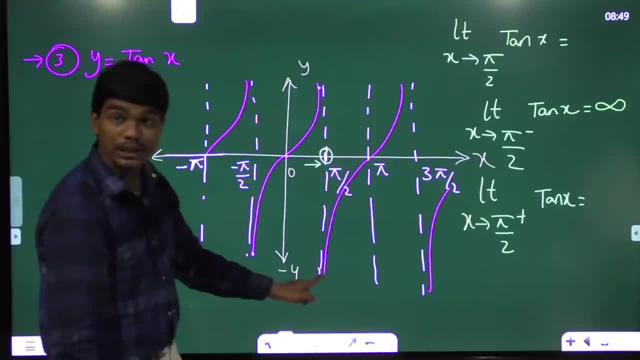 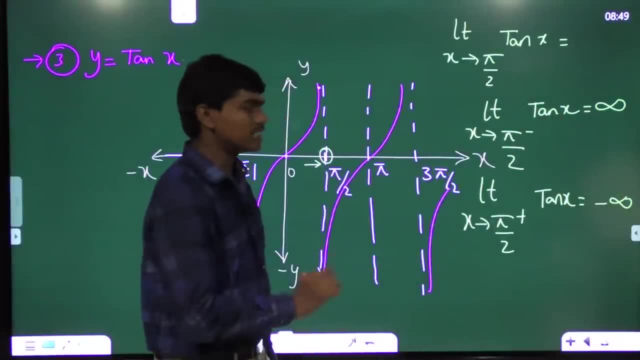 pi by 2. from right hand side, the value of this f of x is tending to minus infinity, Which means the value of limit x tends to pi by 2 plus tan x is minus infinity. And we have seen, when x is tending from left hand side the value is something different than. 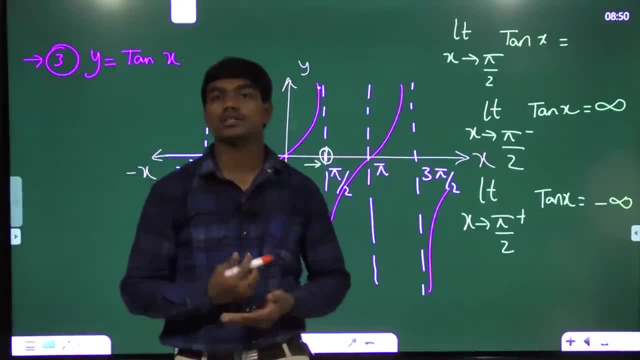 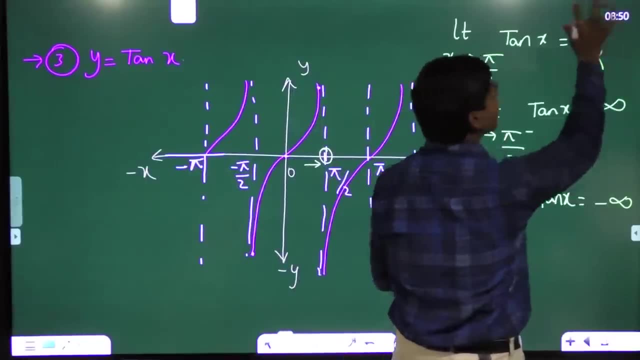 when it is tending from right hand side. So these two values are not the same. So that's why, when left hand limit and right hand limit are not same, we say this limit does not exist. This is the symbol for existence, which I already used earlier. So this is the symbol for does? 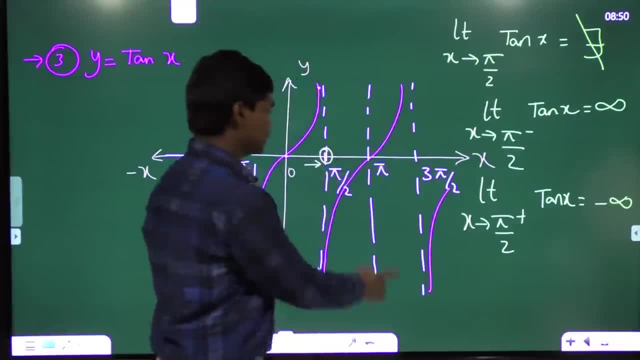 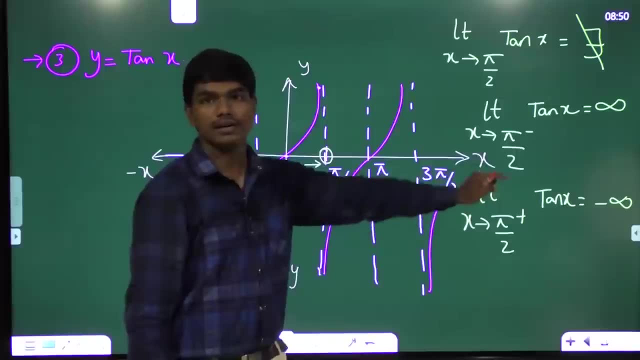 not exist and limit extends to pi by 2, tan does not exist. This is the reason why: Because functional values does not match each other. So please take this tan x curve and divide it, This limit. this was asked in gait exam a couple of times. Please take a moment and 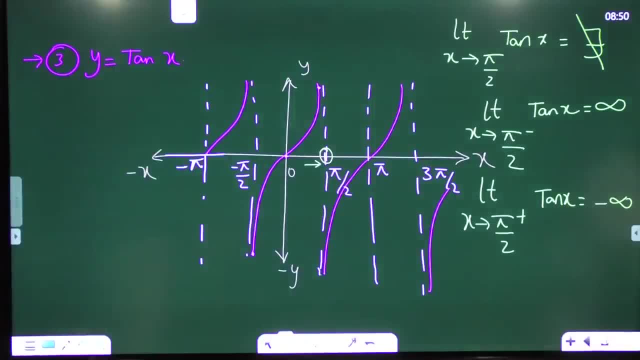 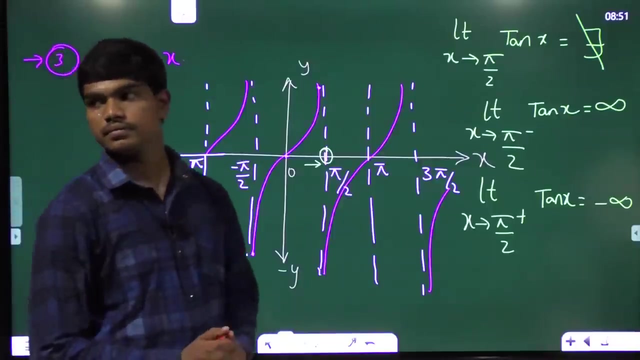 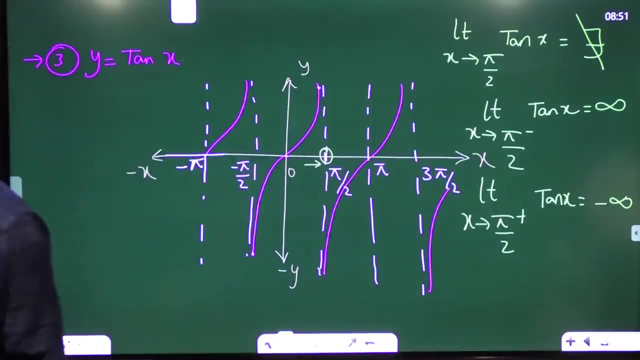 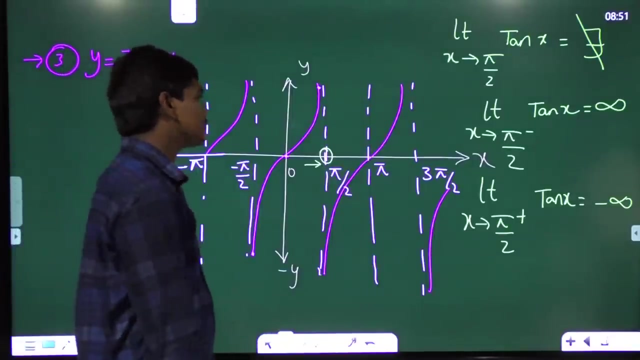 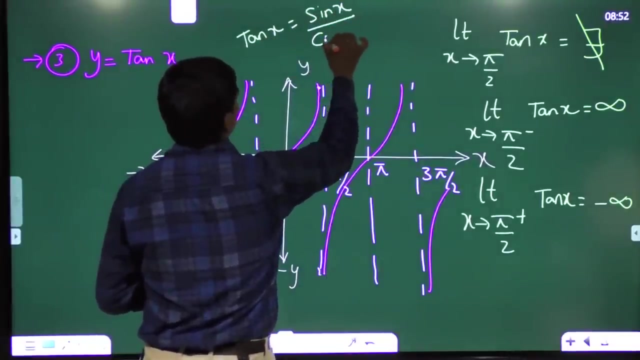 take for this. Notes will be provided in content. Okay, take it. So look here Now. one of the question was: why is tan x curves looks like in different in shape from sine x and cos x? Look this: tan x is basically a ratio of sine x above. 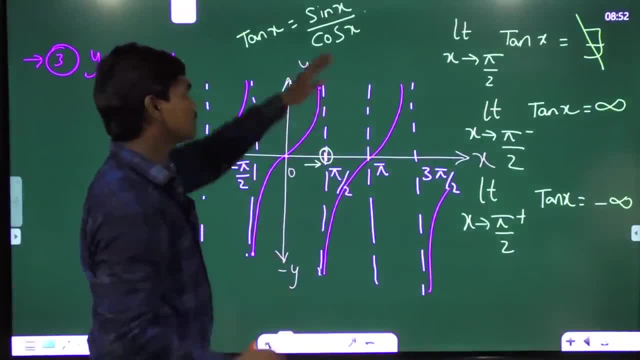 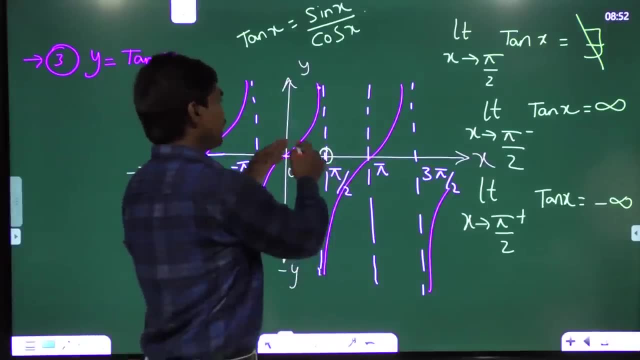 cos x. Now, if you recall the graphs of sine x and cos x, one thing is very clear: When sine x increases, cos x decreases simultaneously. So whenever numerator is increasing and denominator is decreasing, the value increases more steeply than when compared to sine x and cos x. And 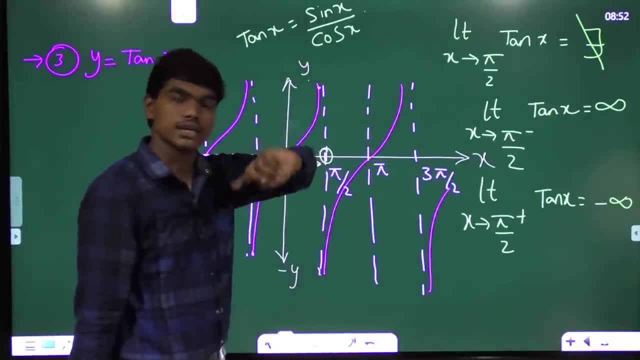 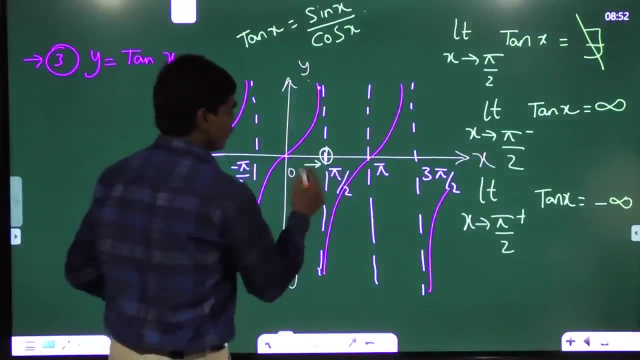 also the limits are plus infinity to minus infinity. So this is the reason Now why limit extends to pi by 2 does not exist is again see here. Then there is my x here and x is tending to pi by 2.. This f of x which is initially here, 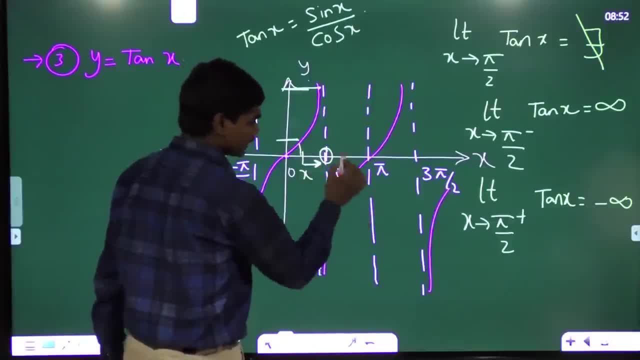 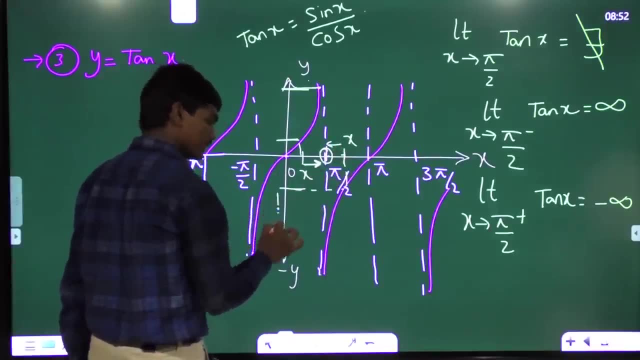 is changing to here by the time it reaches here. Similarly, on the right hand side, if x is initially here, this f of x is initially here, And when x tends to pi by 2 towards this direction, this f of x is again tending to minus infinity. So in both the cases it's 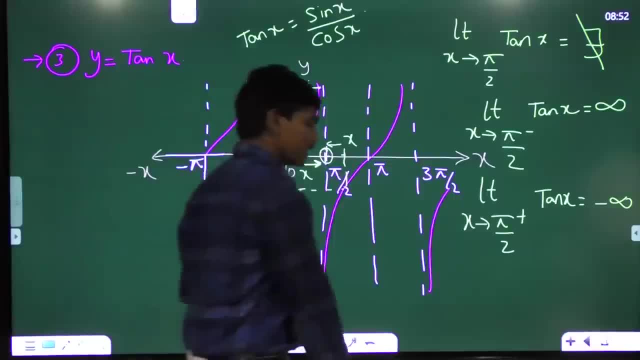 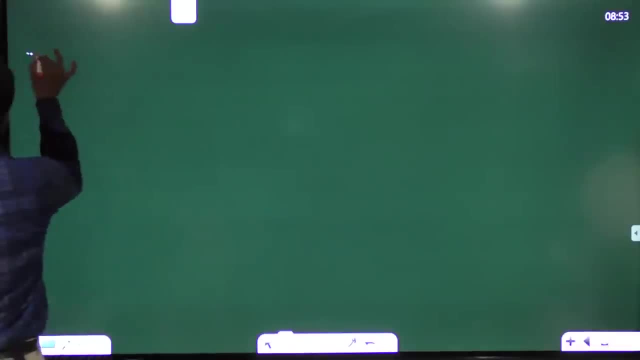 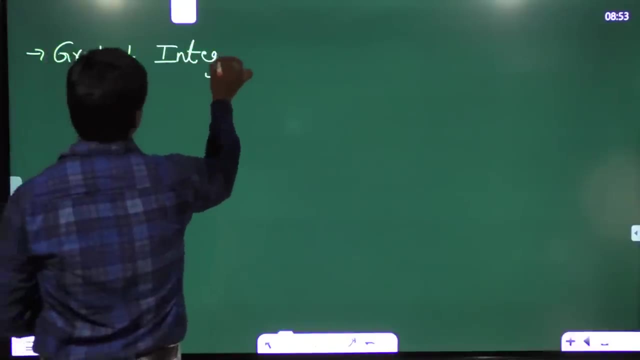 tending to two different values: plus infinity and minus infinity. So this is the reason for the minus infinity. Next, there is one very important function which is called- and also in 2019, a question came from this particular function, which is the greatest integer function. 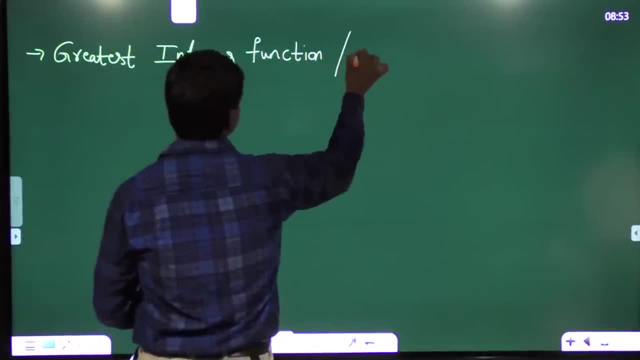 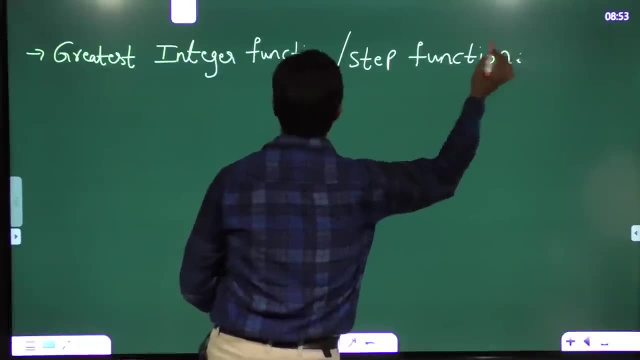 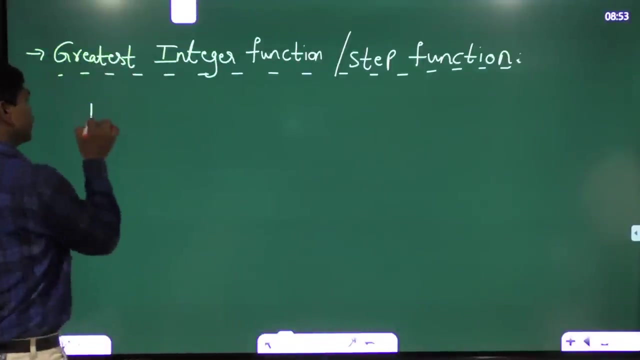 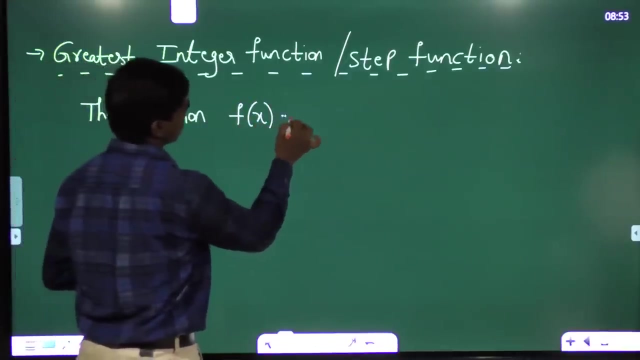 or this is also called with another name, which is called step function. We will see why this function is given the name step function. Thank you. Now what is this greatest integer function? Look, the function f of x is equal to integer. 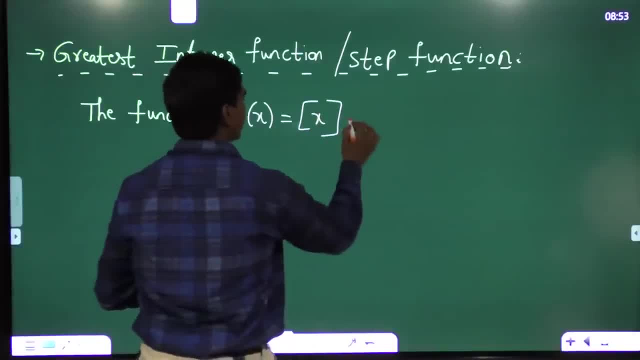 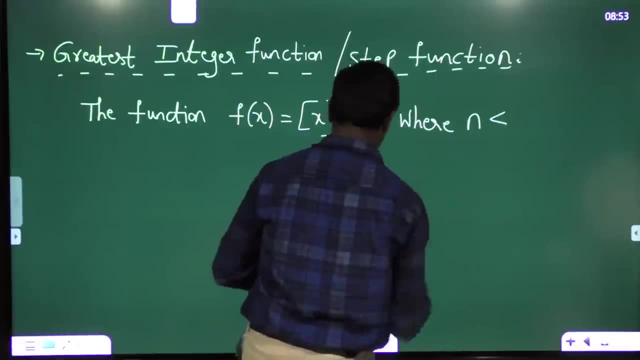 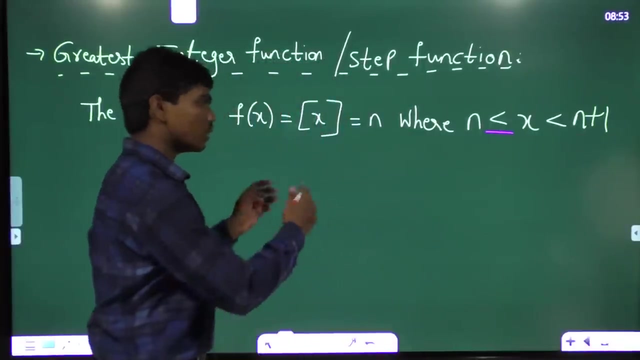 part of x is equal to n, where n less than or equal to x less than n plus 1.. If you see one thing clearly: I did not put the sign equality here, but I put only here, Now, what is the geometrical meaning of this function. Let us see, Let us move this a bit so that you could. 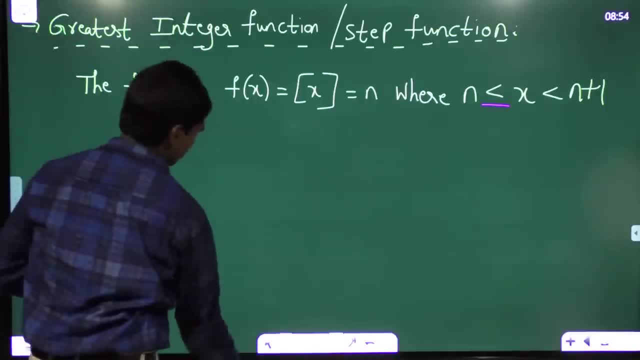 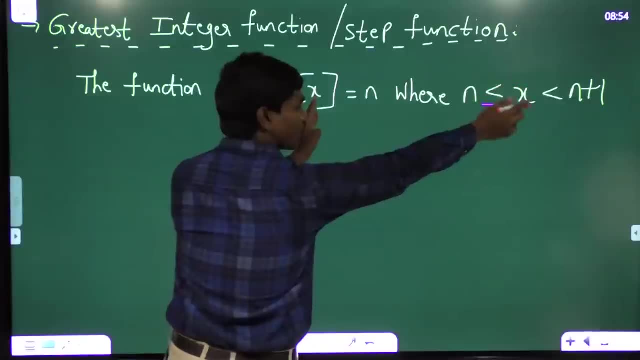 see the thing. So now see here What is the meaning of this function. Now I told you. when x is lying in between n and n plus 1, of course including n in this, the integer part x value is n. 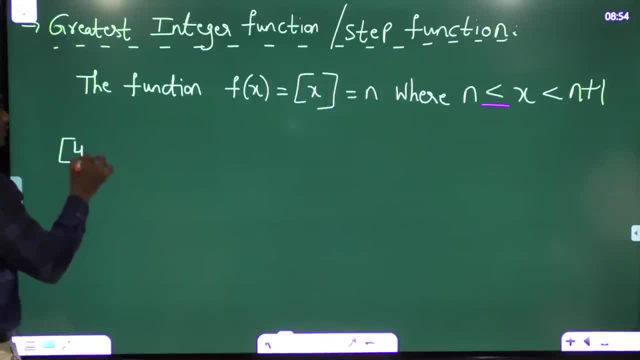 Means. for example, if I ask you what is the value of integer part of 4.12,, what could be the answer? What could be the answer for this Integer part of 4.12? 4.. Because this 4.12.. 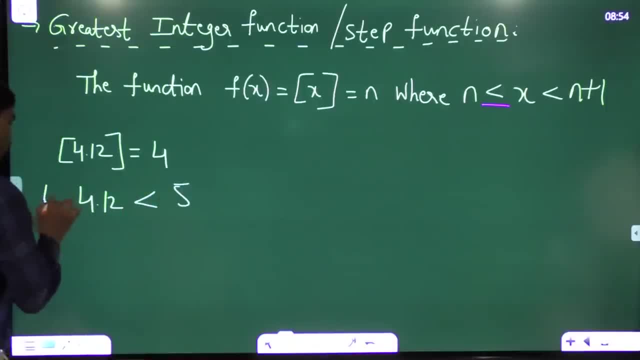 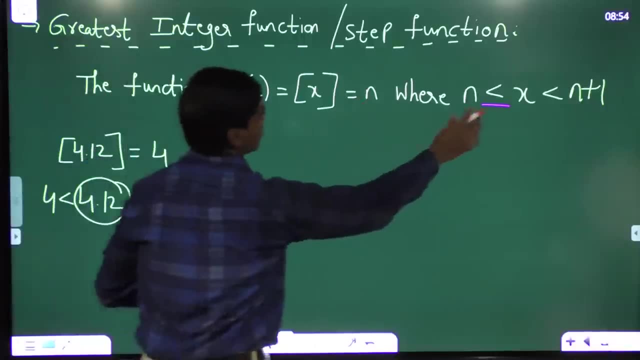 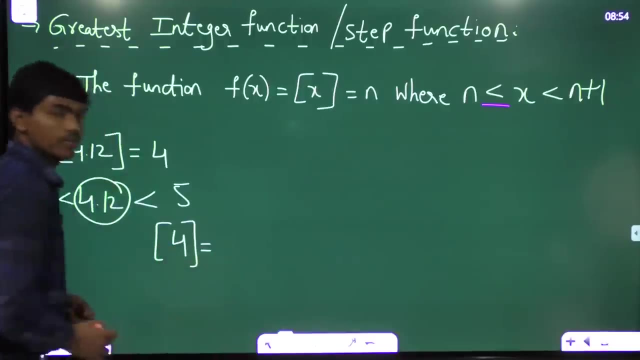 Lies between 5 and 4.. So when this is lying in between 4 and 5, the value is n, when x is lying in between n and n plus 1.. Now what is the integer part value of 4? It is also. 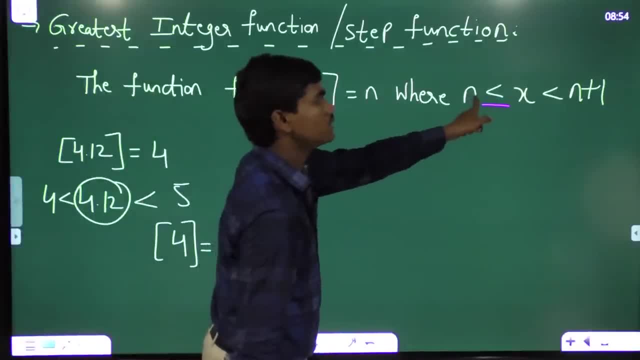 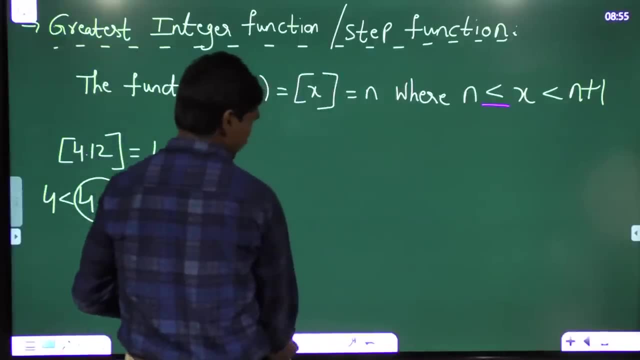 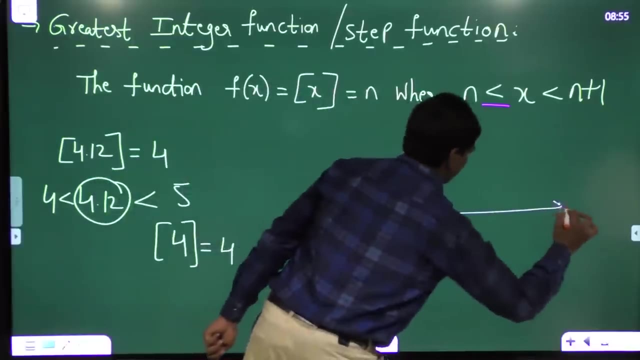 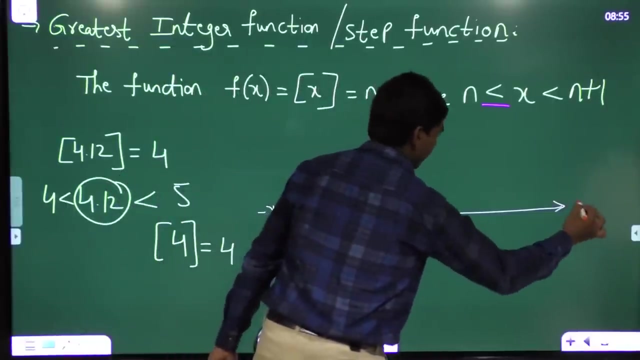 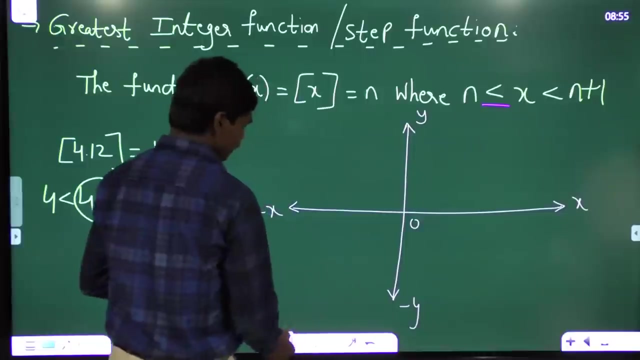 again 4.. Because of this equality sign here, when there is 4 here, 4 is equal to x. then integer part x is same as that integer which is here. Now, if you try to plot this function, what is the value of integer part x? 0 minus x, y, x and minus y. Now let me divide this. 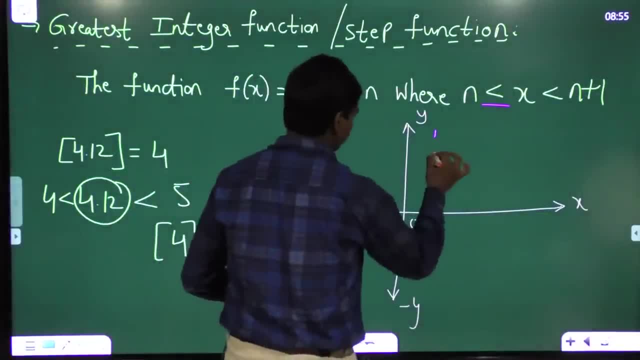 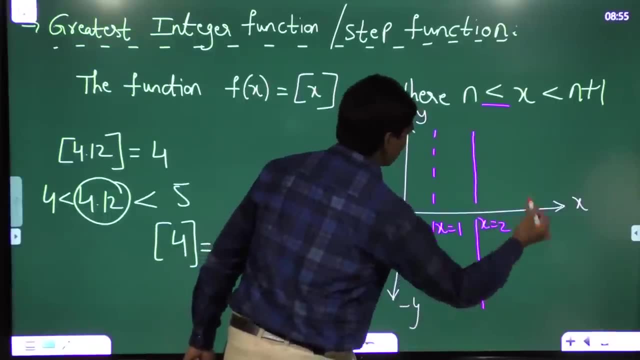 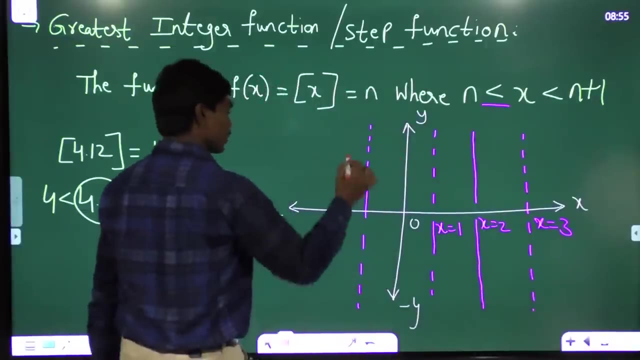 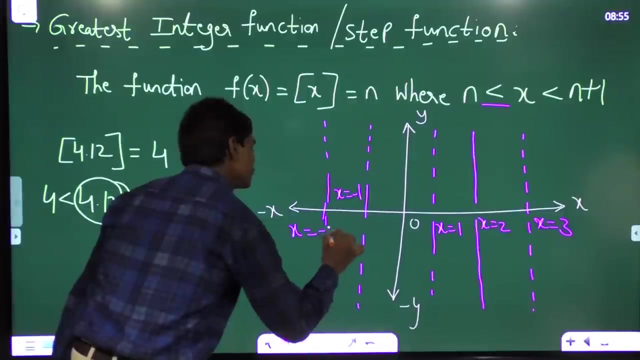 x, y axis into certain partitions. Let us suppose this is: x is equal to 1.. x is equal to 2.. x is equal to 3.. x is equal to minus 1.. x is equal to minus 2.. Now for. 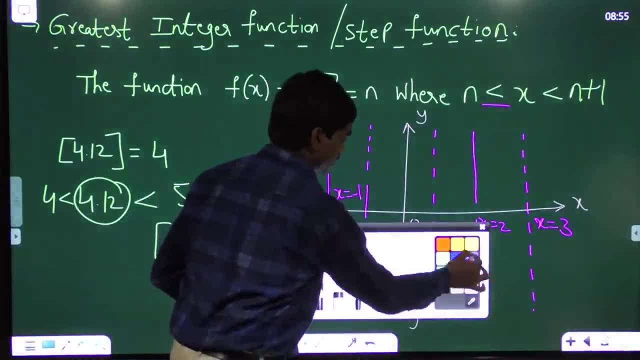 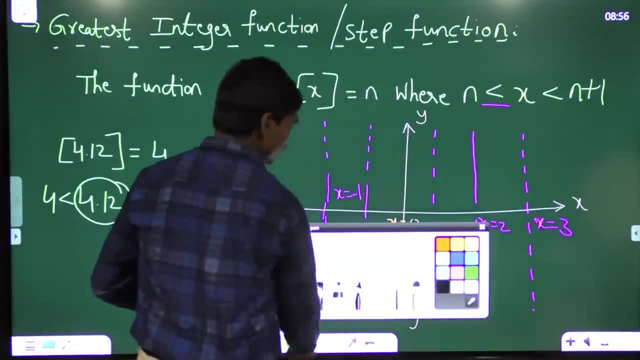 any value of x in between 0 and 1.. Let me use this color Now for any value this is. x is equal to 0, of course, And let me partition y axis as well So that you can see that. 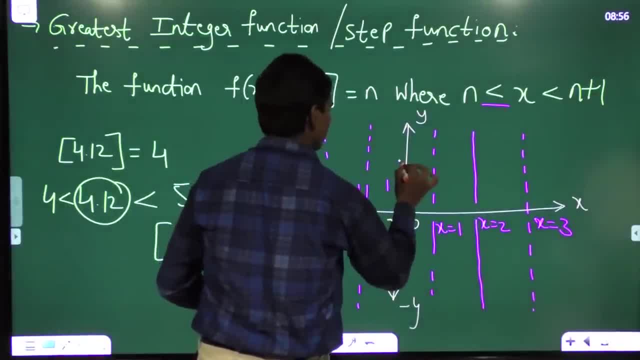 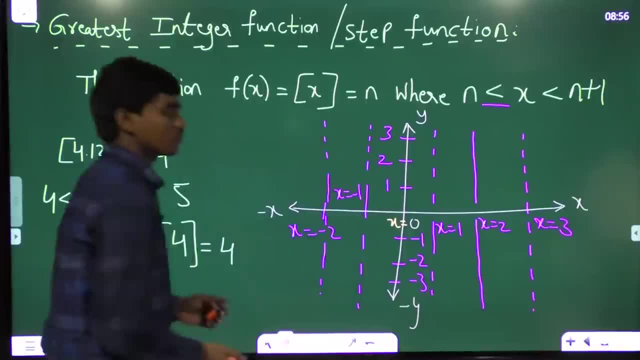 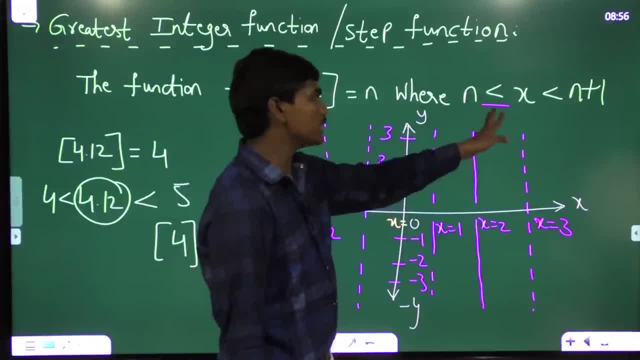 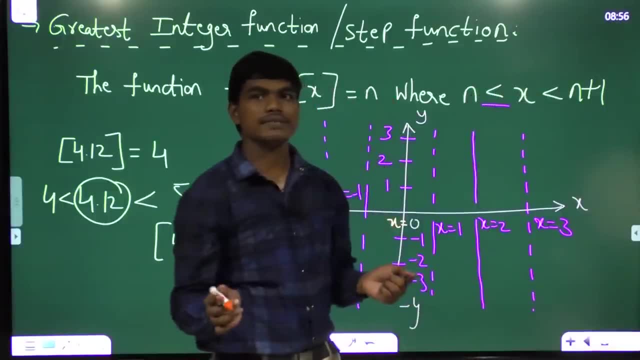 0 and 1, means if you put 0 in place of n, this inequality becomes 0 less than, or equal to x less than 1. Means for every value of x which is in between 0 and 1,. what could? 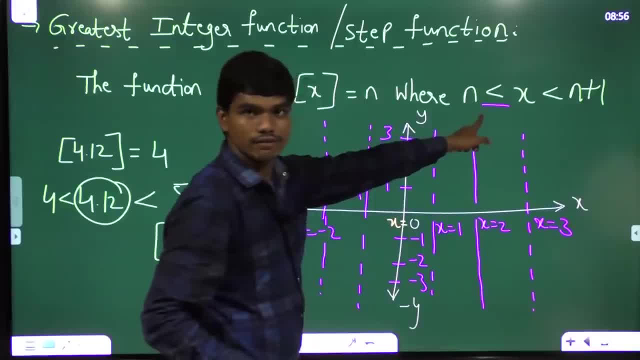 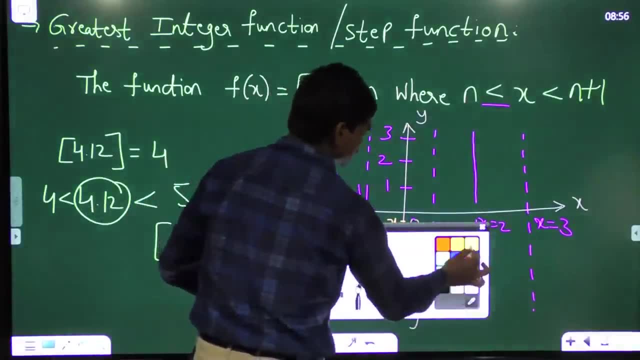 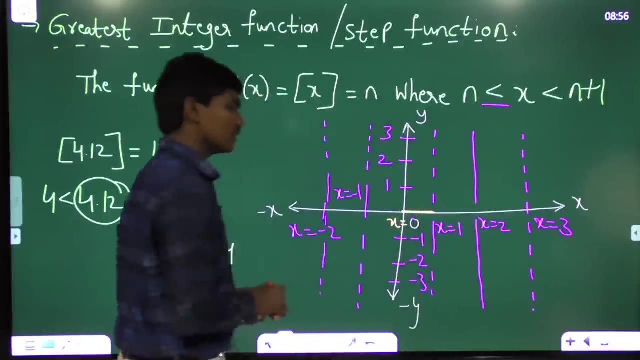 be the integer part x value n, Correct? And since you can see that, you can see that you have 0 in place of n. the value of this integer part x is 0. Which means, for every value of x which is in between 0 and 1, the value of integer part of x is 0.. Correct, Now for. 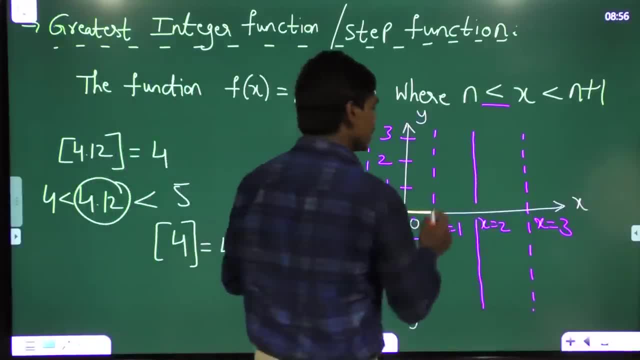 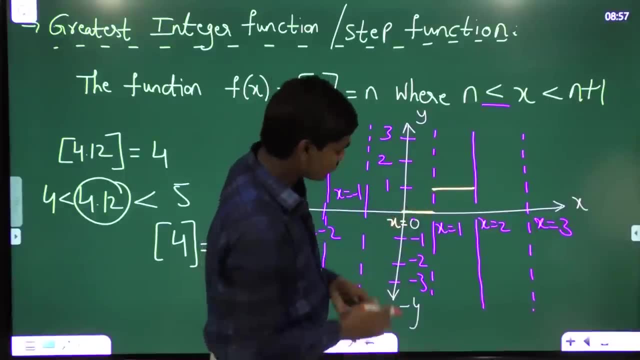 every value of x, which is in between 1 and 2, what could be the integer part of x. It's again 1.. Correct, If you see one thing clearly. let me tell you one thing here, a very important thing. 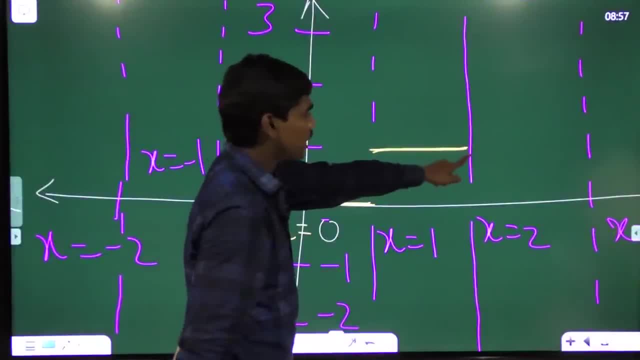 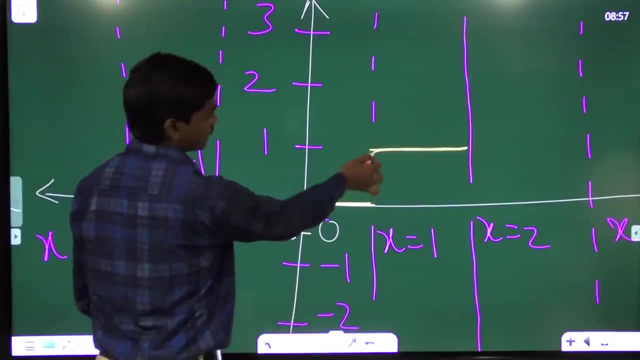 If you see, clearly, I didn't touch the line with the line. x is equal to. I have touched here at x is equal to 1. Of course I have touched it because you can see the line clearly touching this line, this pink line. But here I didn't touch The reason for not touching. 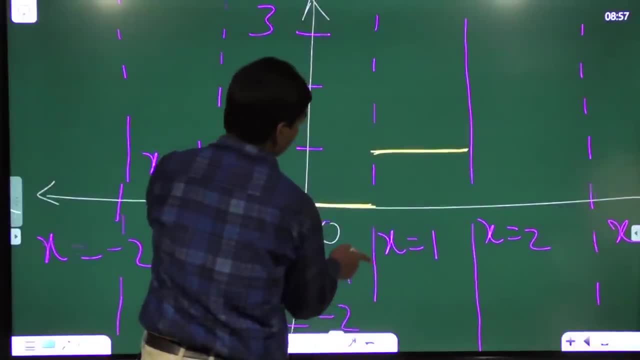 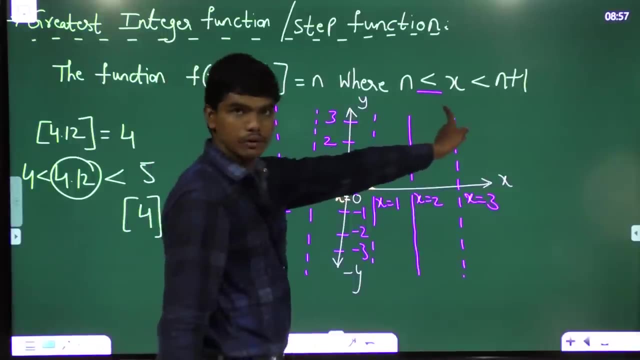 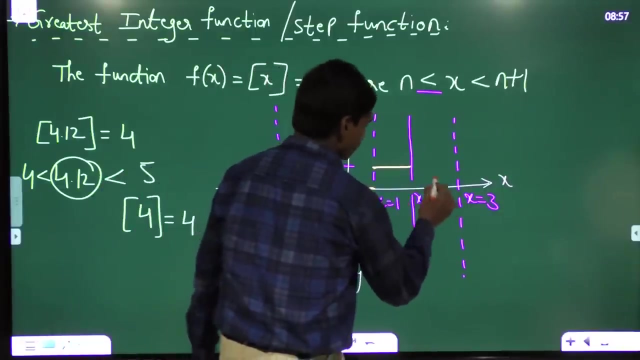 this yellow line, with this pink line, is because I didn't put the equal to. Since there is an equal to only here, I touched only with the left hand value of y, but not with the right hand. So see, For every value between 2 and 3, the value of integer part x is 2.. Okay, Next, For every 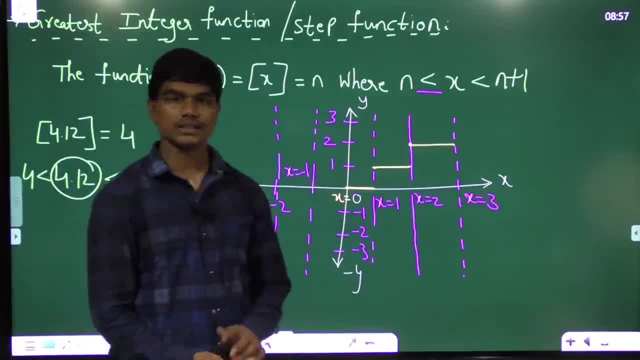 value between 0 and minus 1, what could be the integer part x value? Could you guess? For every value in between 0 and minus 1, what could be the value of integer part of x? Could you guess What's the answer? Any comments on that? 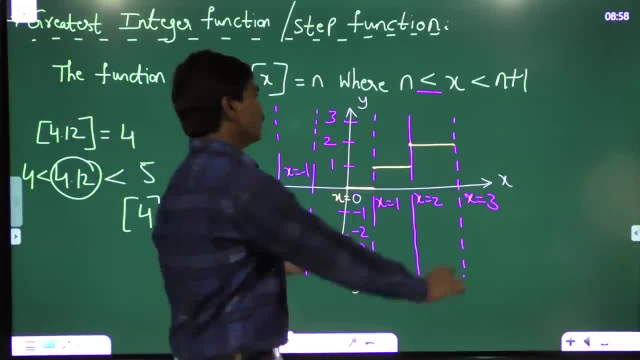 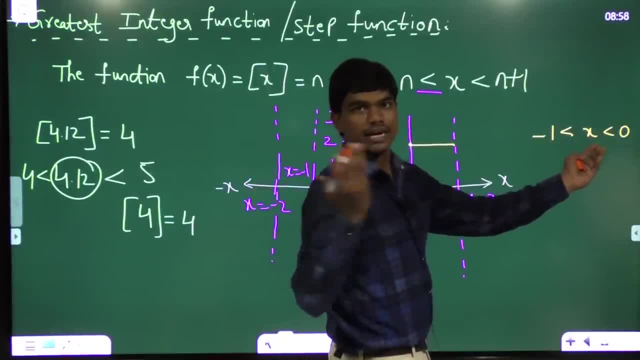 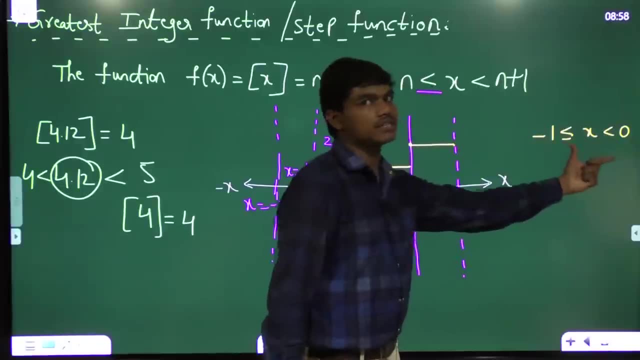 the inequality which holds good in mathematics, because minus 1 is to the negative of x axis and that is clearly less than 0. So when you have a 0 equal to sign here, for every value of x lying in between minus 1 and 0, the value should be minus 1, in accordance. 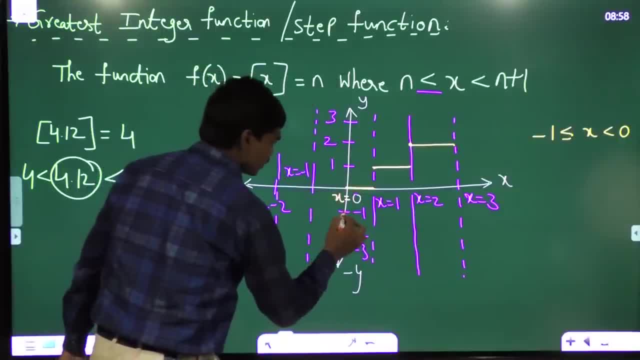 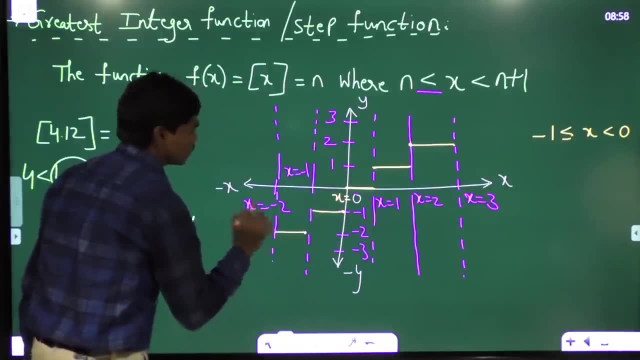 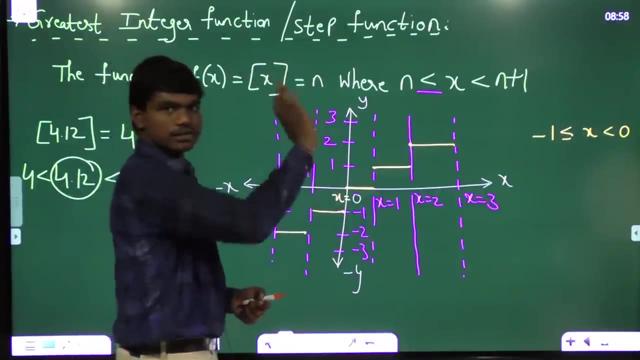 with this definition. So for every value between 0 and minus 1, the value is this, something like this: Similarly, here, this is minus 2.. So this is how the gate integer part function looks like. Correct Now, if you see, the name step function came for this graph because you can. 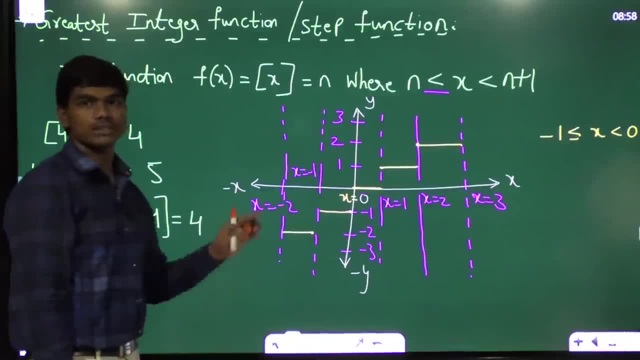 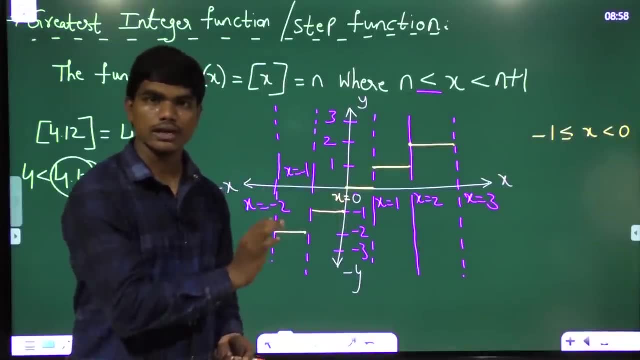 clearly see there are steps Clear. So please take this definition and remember this is a very important function as far as gate is concerned. So please take it clearly. If you don't understand why I am putting this 4, 4 and drawing this graph, you please ask. 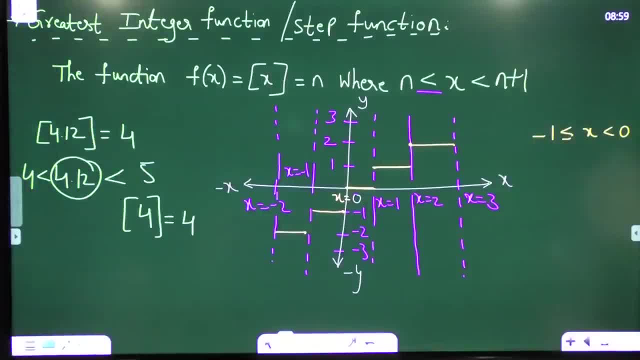 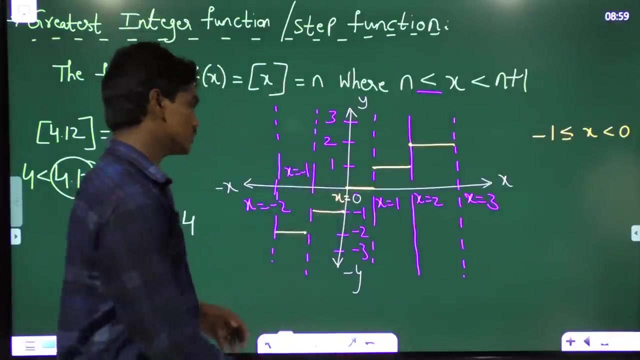 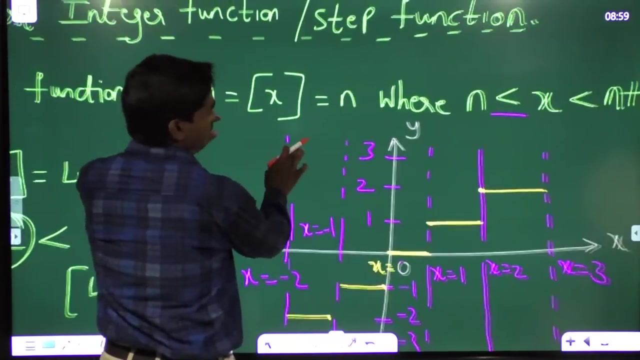 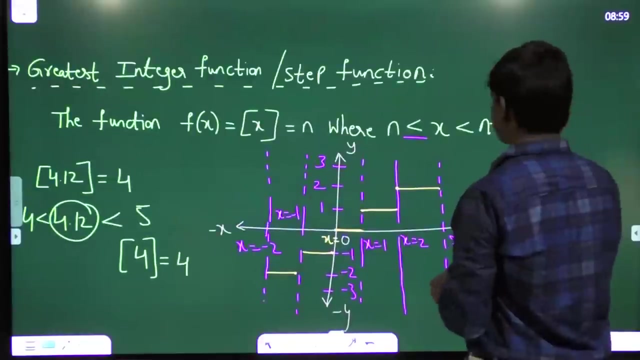 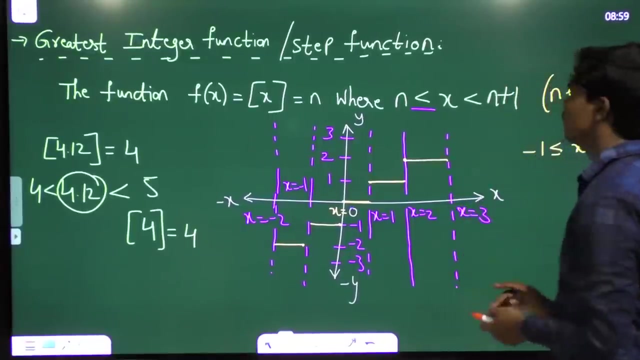 me. I will repeat it. 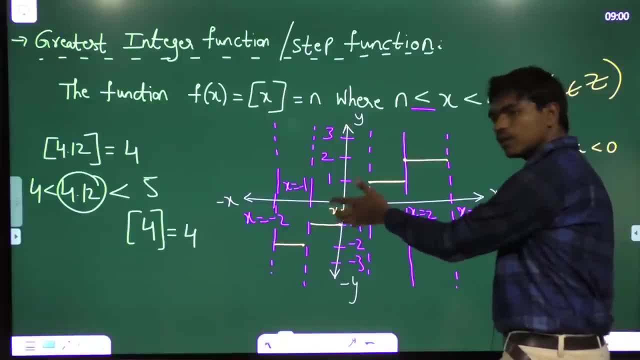 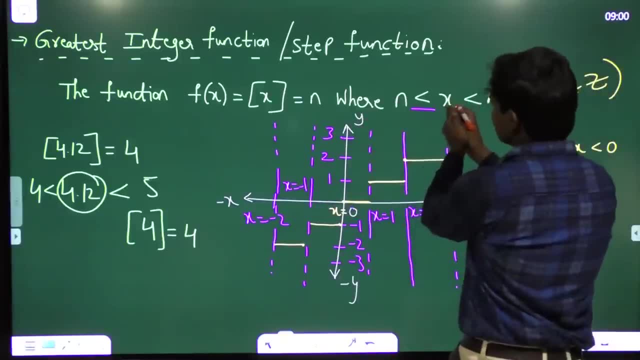 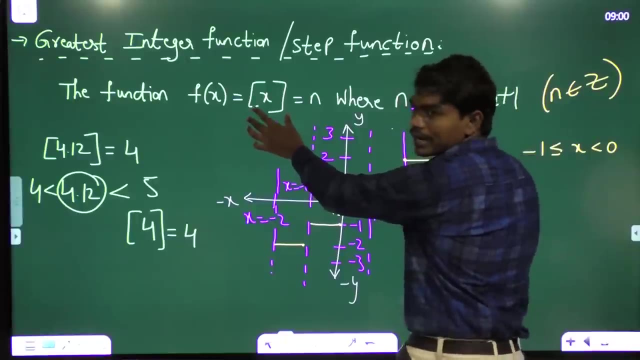 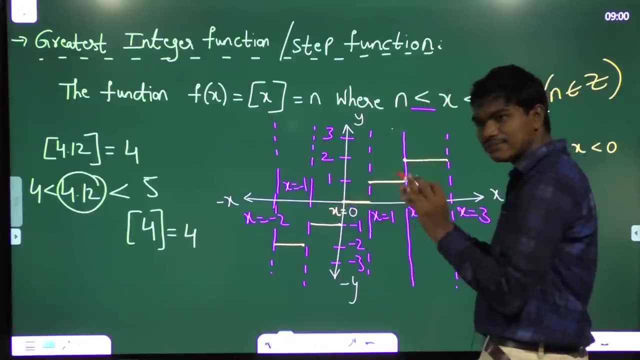 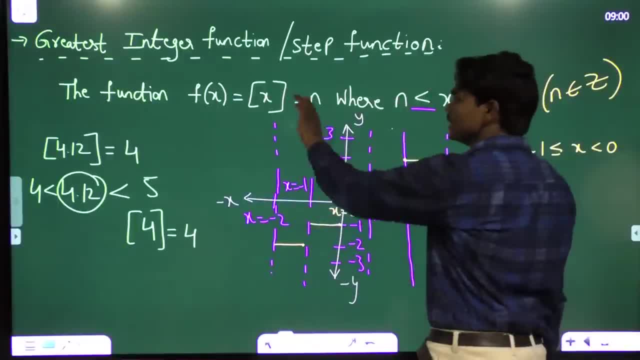 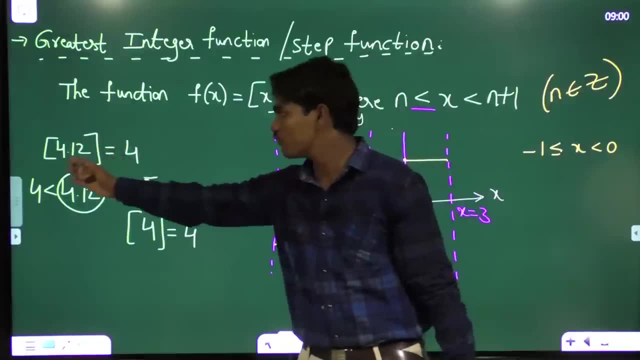 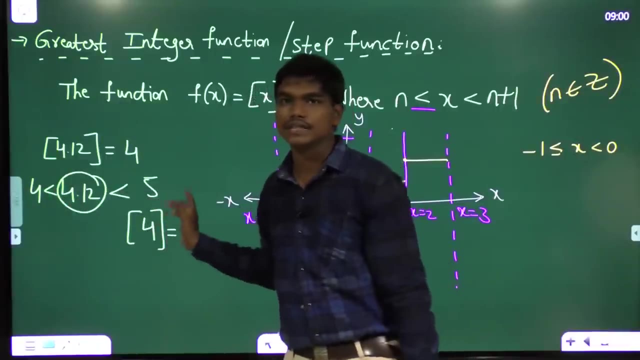 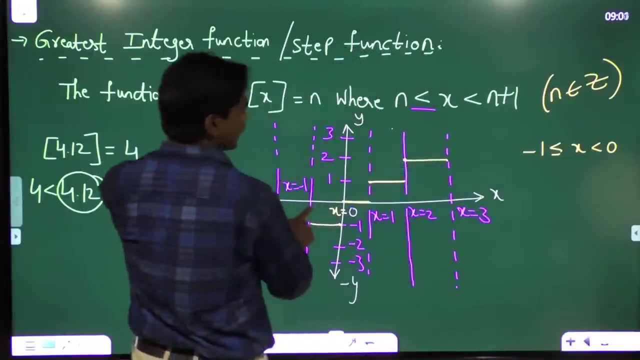 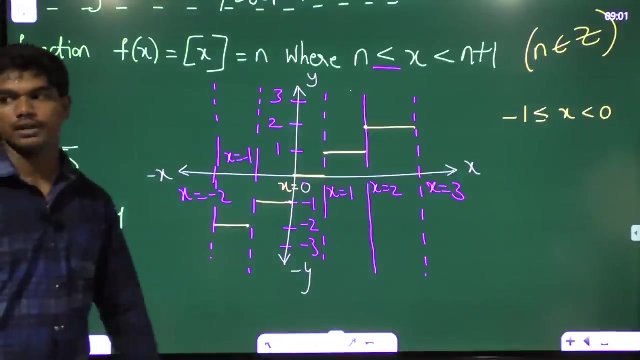 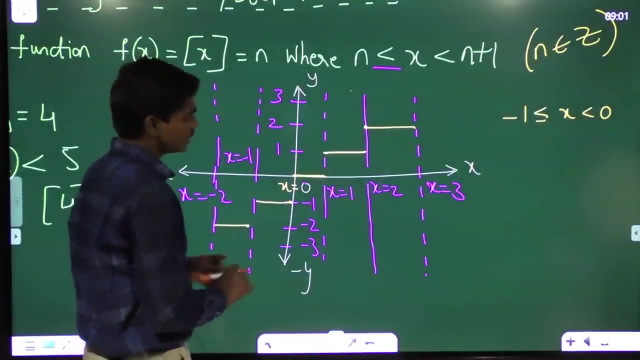 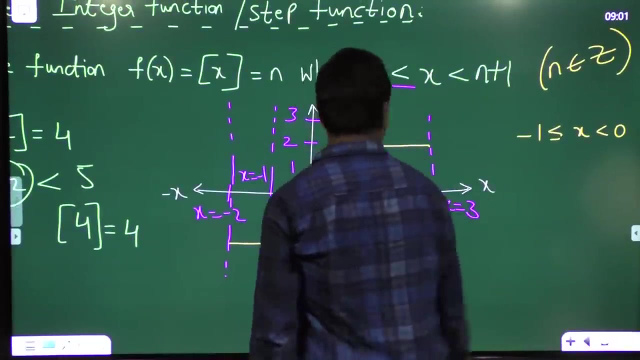 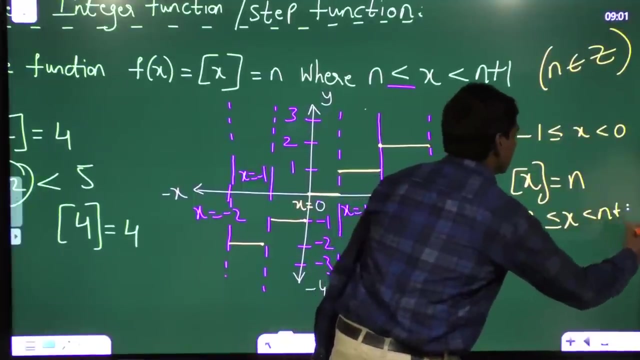 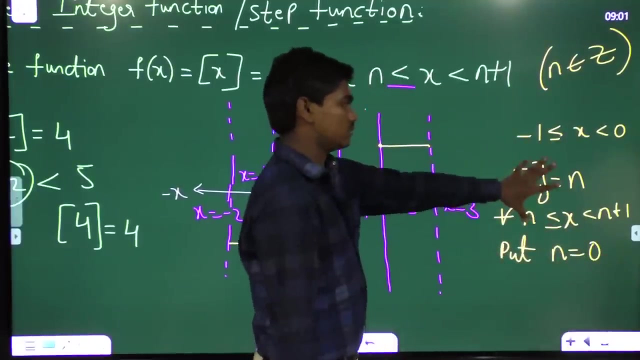 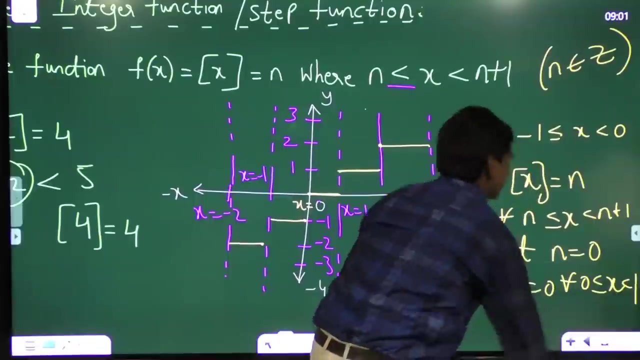 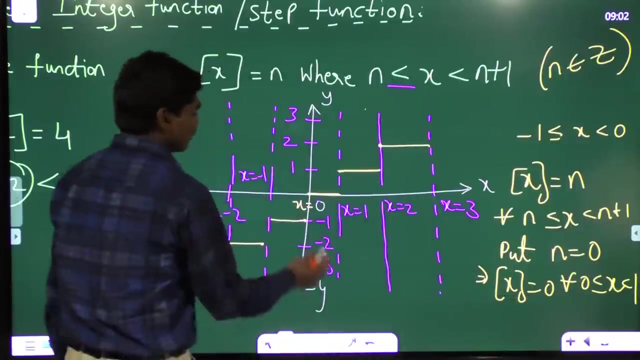 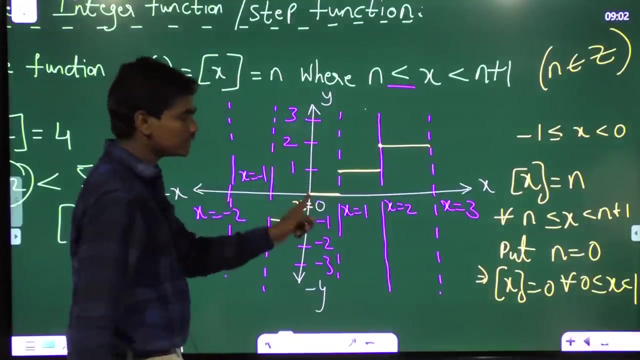 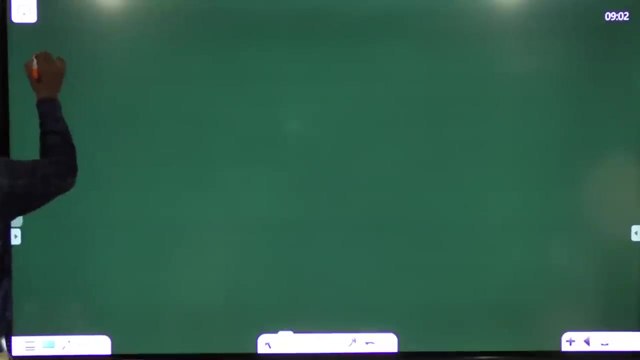 or this is also sometimes written as very carefully taken out of this maximum of minus. 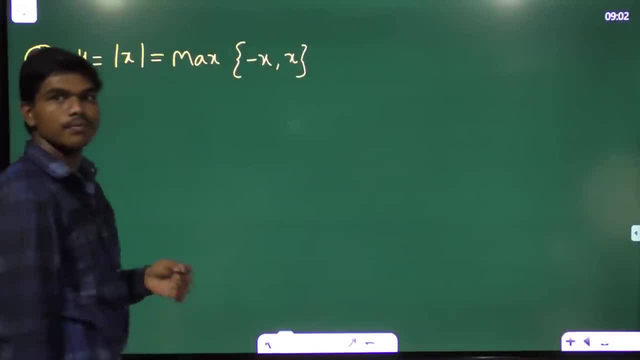 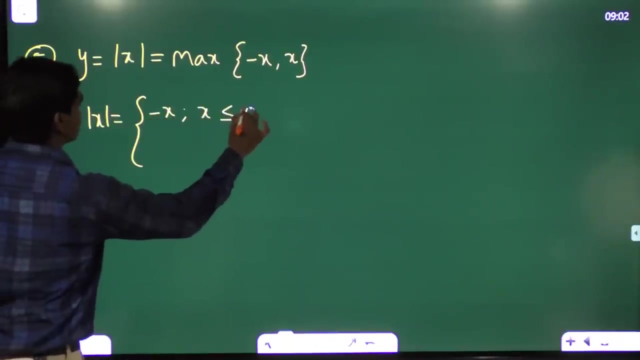 x, comma x. these two functions are same, okay, minus x, comma x, because if one is negative, the other is positive and value is obviously positive. okay, and this mod x function is defined as: mod x is equal to minus x when x is less than, or equal to zero x when x is greater. 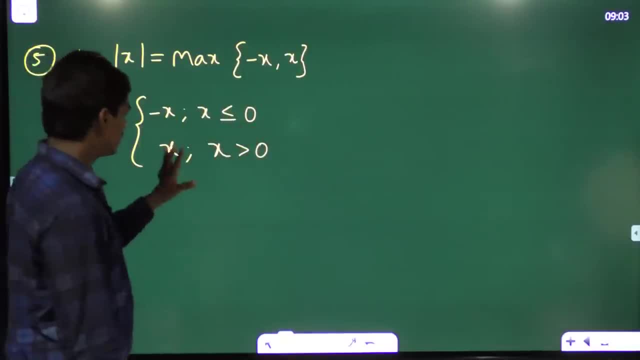 than zero. of course, if you need, you can put the equal to sign anywhere, it doesn't matter. this function is stated this way. now let me tell you an example. if i ask you what's the value of modulus of minus 5, what could be your answer? it's 5. okay, now you may doubt. 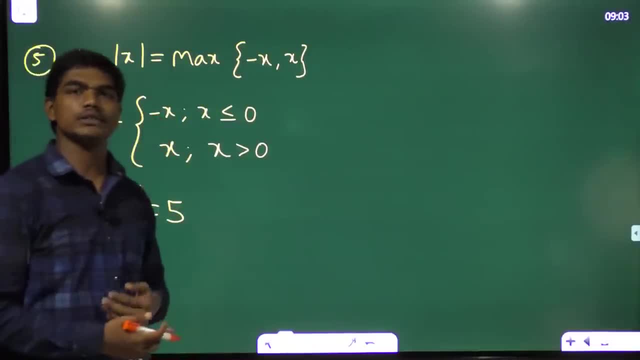 one thing: when i write minus x here, you may have a doubt. when mod x function is always positive, how come the mod x function give a negative value here? if you see clearly, i have stated x is less than 0. when x is less than 0, minus x is positive. okay, so mod x always. 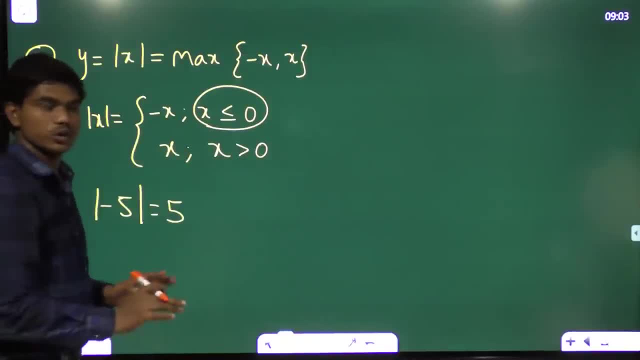 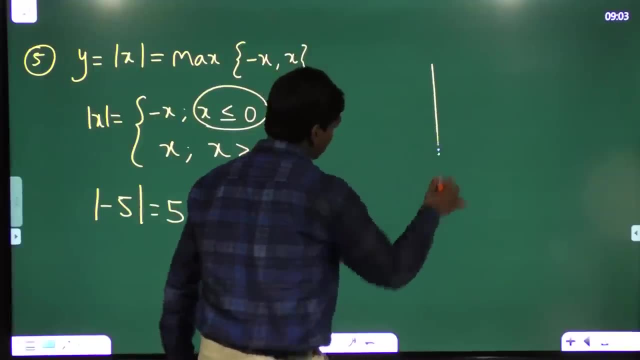 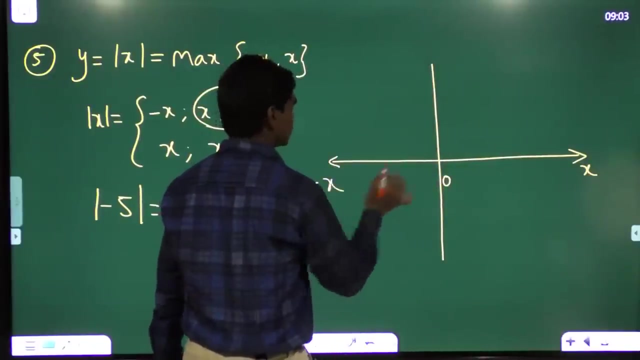 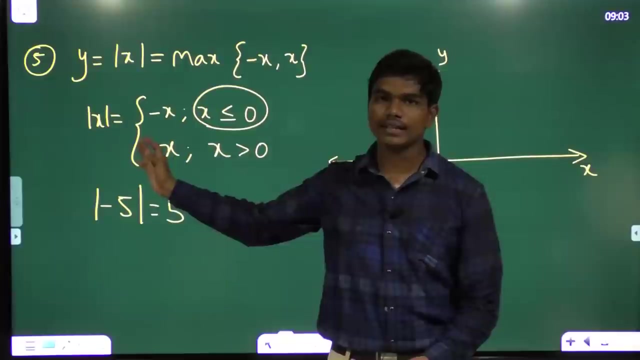 gives you positive values, and when x is greater than zero, this is x, no issues. now let me try to draw the graph of this. y is equal to mod x. again, setting up the axis x minus x, y and minus y. now one thing is very clear: whatever you put in case of x, this mod x is never negative. 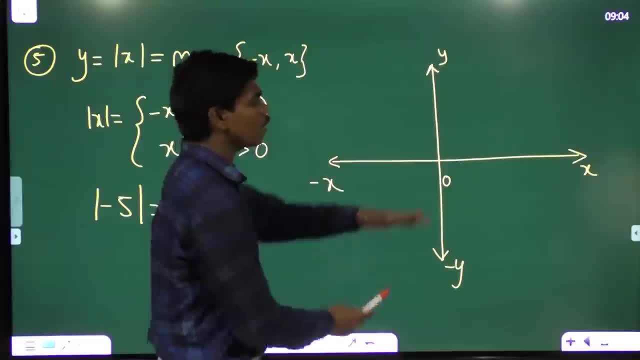 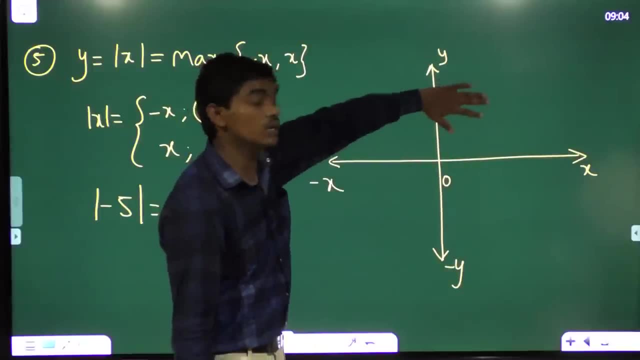 which means, whatever the graph you try to draw, that graph always lies negative above x axis, because this y values can't be negative and graph can't fall below this, which means the graph lies only in the first and second quadrants. so now let me try to plot. 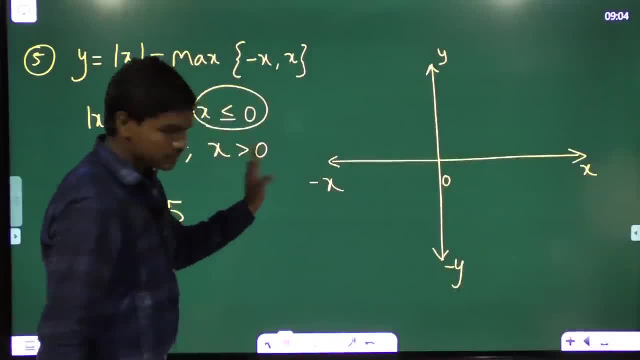 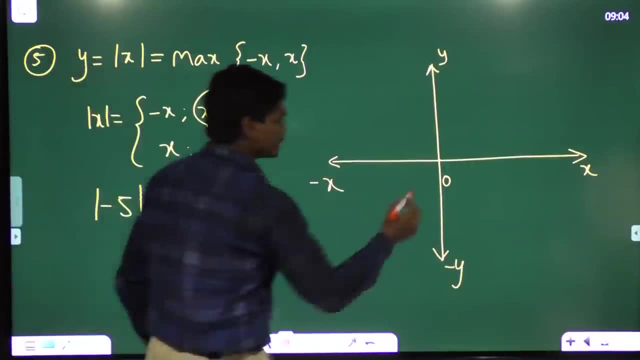 the function. if you see, for x is greater than 0, if x is equal to zero. first of all, what the value of this mod x? when x is equal to zero, mod x is equal to minus zero, which is zero. so something here: zero is the value. now, when x is greater than zero, the function is: 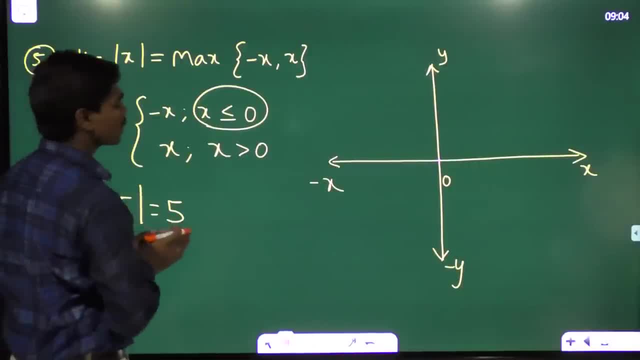 y is equal to. if this is y, basically y is equal to mod x. that's what we talked about. So if x is greater than 0, y is equal to x. You know the lines: y is equal to mx. 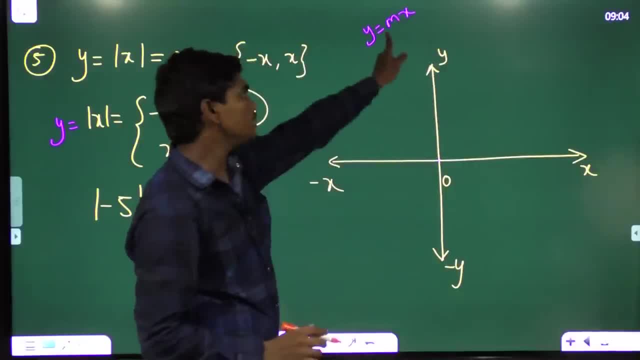 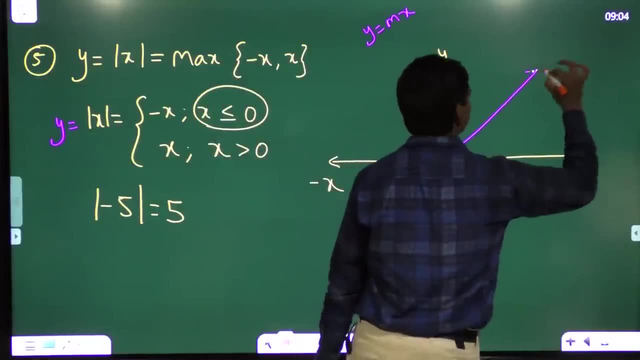 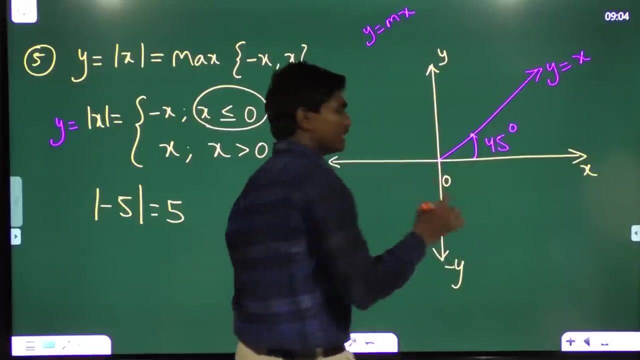 passes to origin, which slope has m, which means for the line y is equal to x. if you try to plot for x greater than 0, the graph looks something like this: y is equal to x And if you see, this angle is 45 degrees. Why this angle is 45 degrees? Because in this y is equal to mx. 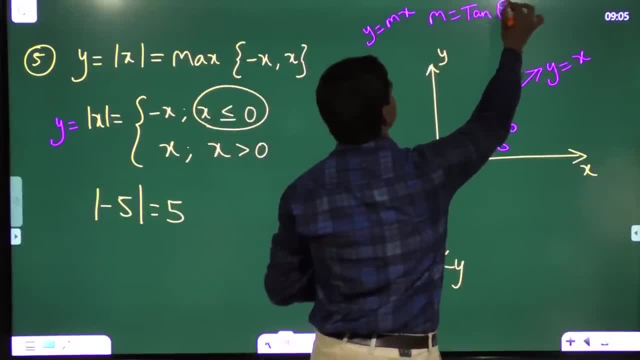 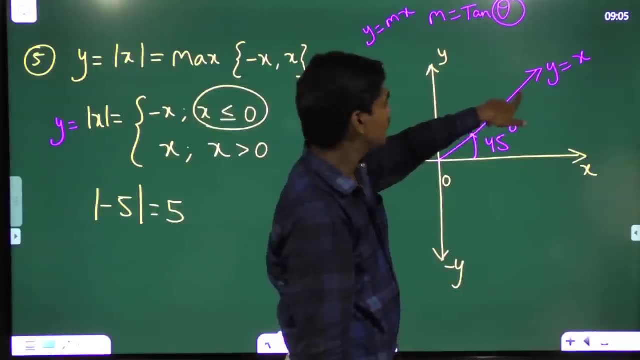 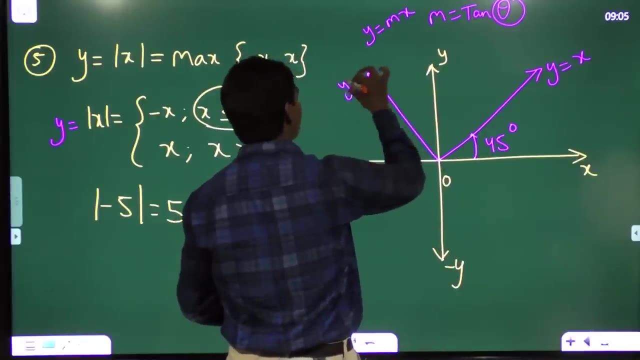 this m is nothing but tan theta, where theta is the angle made by the line with x axis. So here, in this case, since m is equal to 1, y is equal to x, so this angle is 45,, since tan, 45 is 1.. Similarly, this is how y is equal to minus x, looks like, because when y is 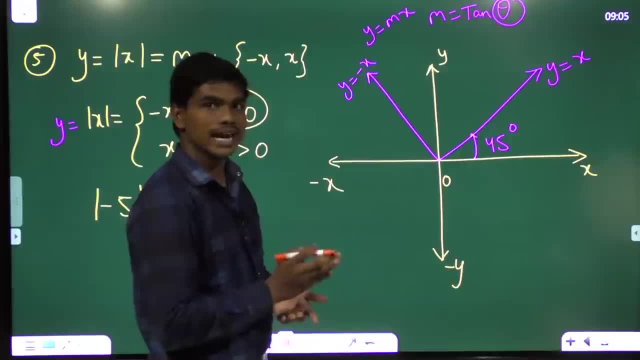 equal to minus x, slope is minus 1.. If slope is minus 1, slope is minus 1, slope is minus 1.. Then tan theta is minus 1, which means theta is 135 degrees from positive rotation of x axis. 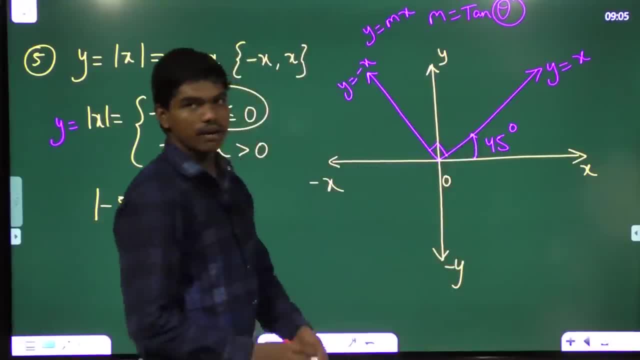 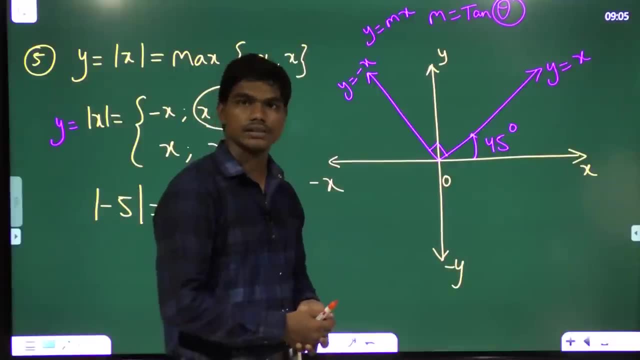 which means these two lines are perpendicular to each other. Now one thing at later stages we could talk about this mod x function is continuous everywhere. It doesn't have any break in between. So this is the graph of mod x, which is one of the important things. 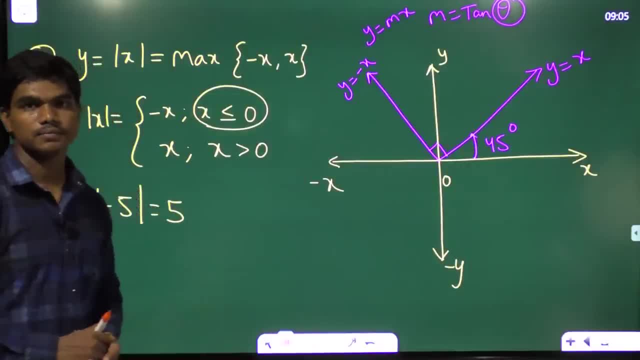 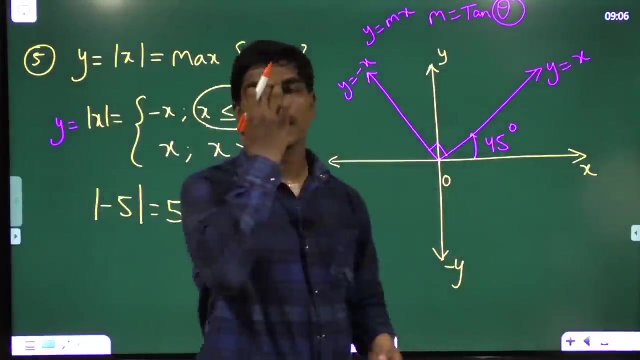 in terms of continuity and differentiability. Please take it. Well, a few of you are asking about the class timing. Generally, from Monday to Saturday, class will be from 7.45 to 9.15,, but I apologize for today. 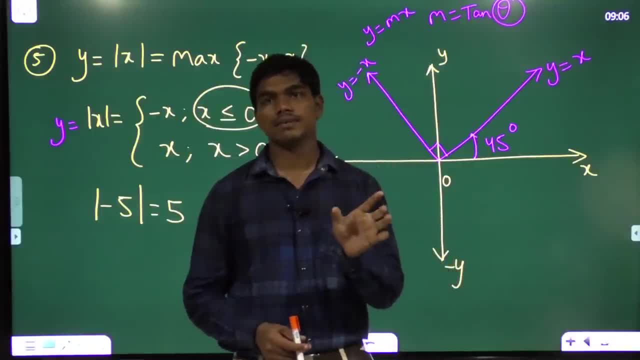 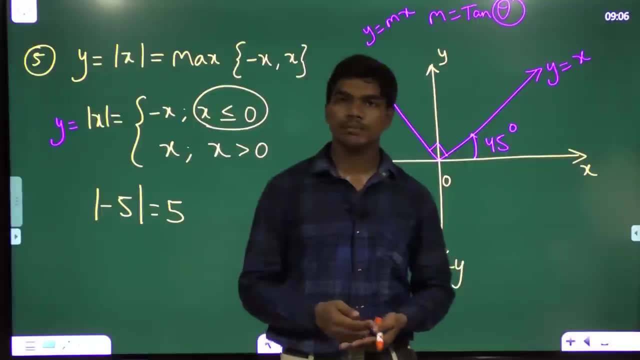 there's a technical slag here. So daily, from Monday to Saturday, class will be from 7.45 am to 9.15 am, And on Sunday we'll plan for a longer class. We took this decision because: 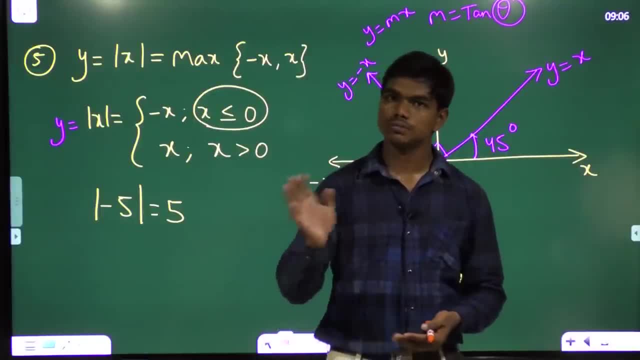 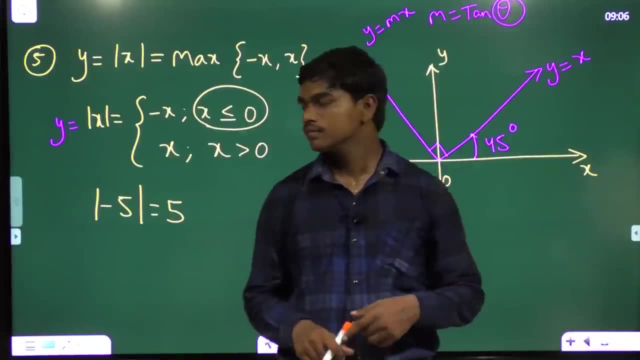 undergraduate colleges are offering their semester exam courses to students via online, So we need to plan before the college hours and after that, Don't worry about notes. I'll make a Google link and I'll upload in the comment box of this video. 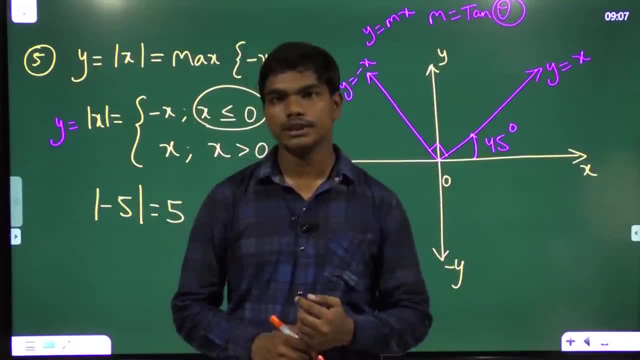 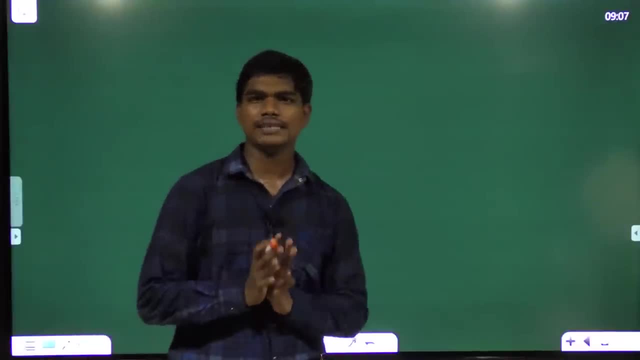 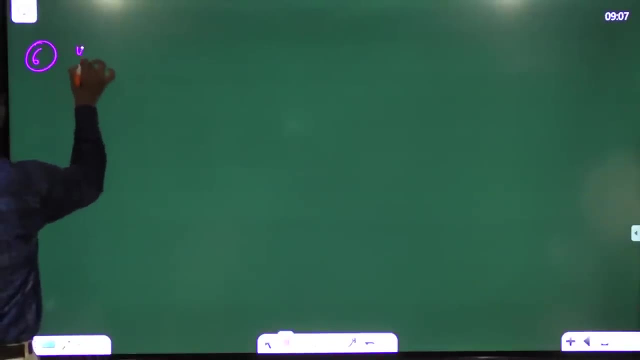 Taking this mod x graph done, Can we move ahead? Any issues so far? Okay, So next Next graph is very, very important in terms of gate. A lot of questions have been turned up and the graph is something like: y is equal to log x to the base. 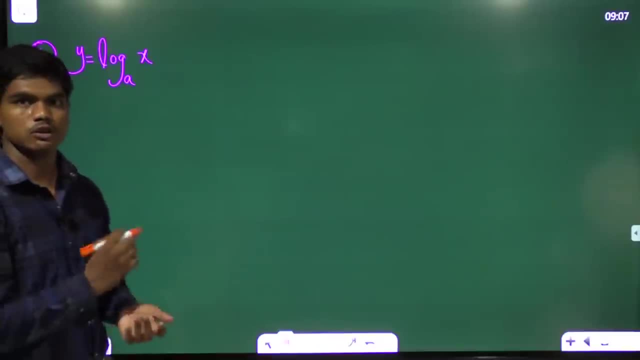 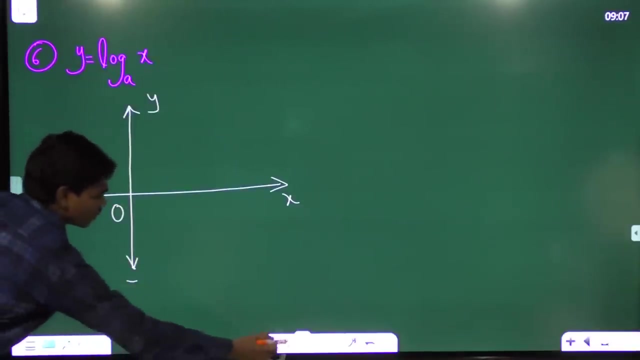 a. It means basically the log x graph, whatever could be the base. Now, if I try to draw this graph, 0 x, y minus x. I'm sorry, this is minus y and this is minus x. Okay, Now one thing you need to make. 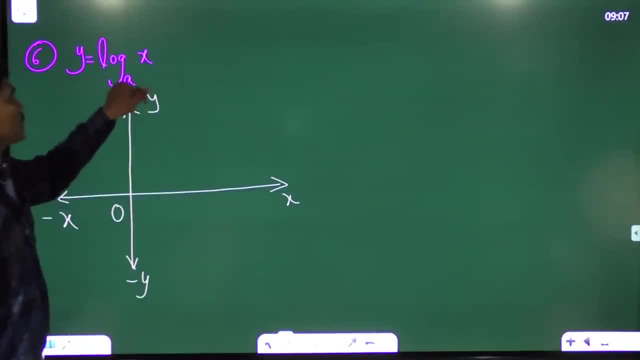 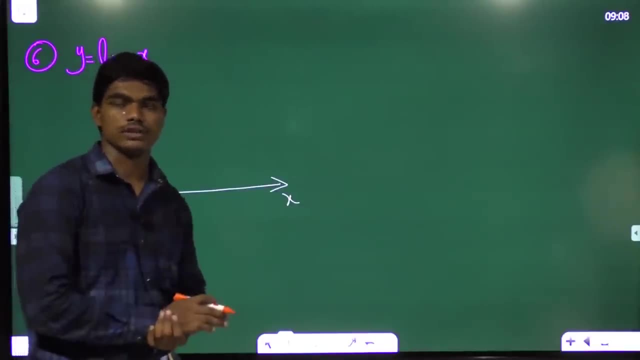 a note of This: as long as this a is positive, this x also should be positive. It means logarithms are not defined for negative real numbers, They are defined only for positive real numbers. Okay, So this log x graph. till this moment you are clear. 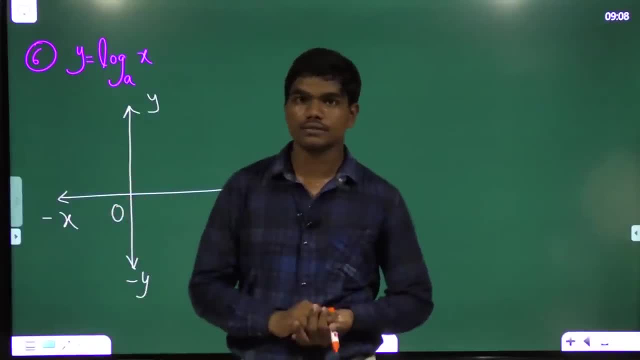 Now, this log x to the base a function has two graphs based on the value of this a, And that's the reason why this is asked in many interviews. They'll ask you to draw the graph of log x to the base a Then, without asking the value of a, if you start drawing the graph, 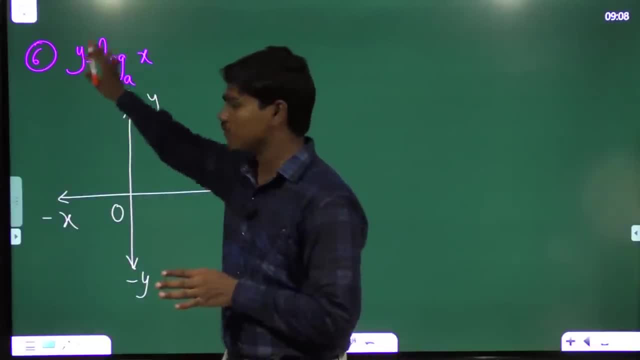 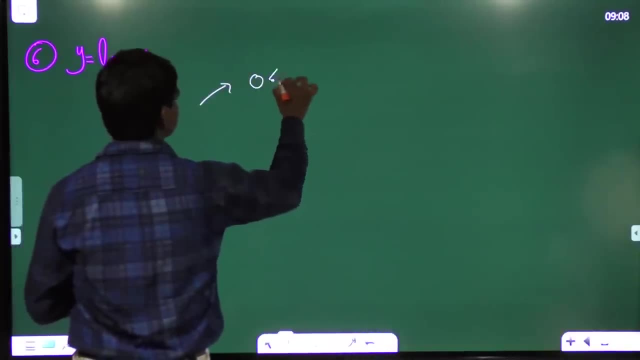 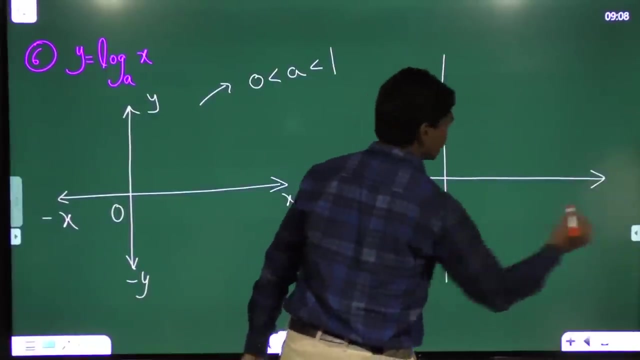 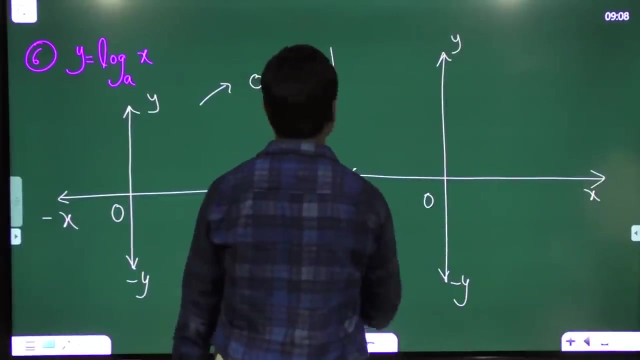 it's a mistake, Okay. So please, when they ask you to draw the graph of log x to the base a, kindly ask them, sir, what's the value of a? Okay, Because when 0 is less than a, less than 1, there is one graph for this, And similarly, 0, x minus x, y minus y. If you see, when a is greater than 1, there is another graph for this. 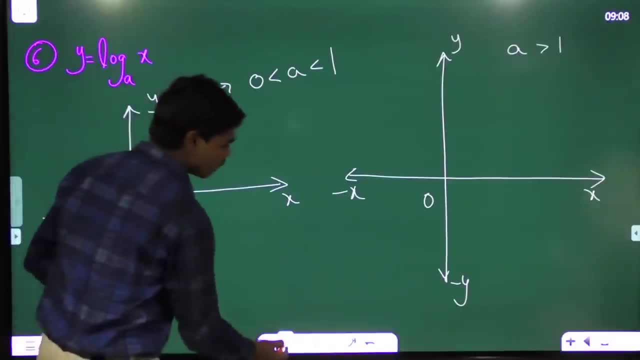 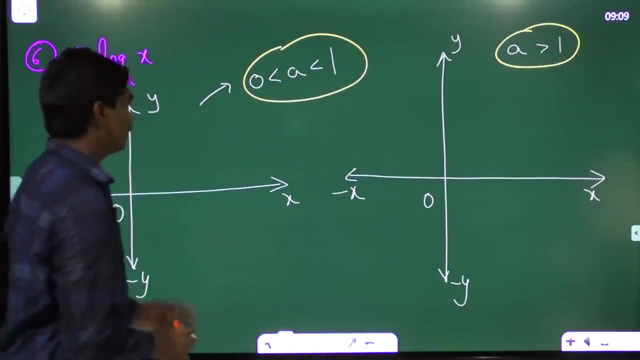 Okay, So there are two different graphs depending on the value of a. When 0 is less than a less than 1, and this is a is greater than 1.. So first of all, let us look at this particular case. 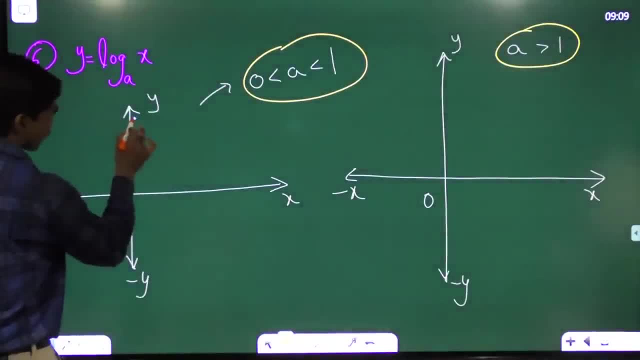 The graph for this looks like this: where this value of x is 1,- and you know, log 1 to any base is 0.. And when x is- I mean when a is- greater than 1,, the graph looks something like this: 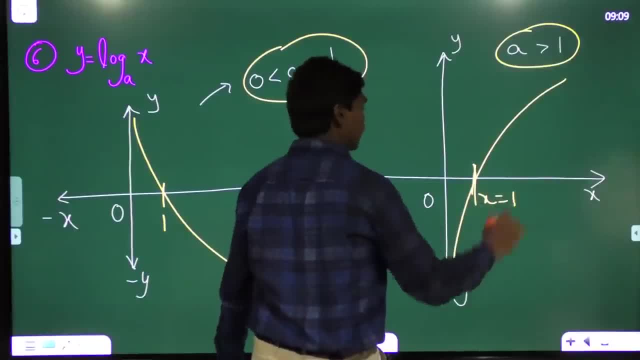 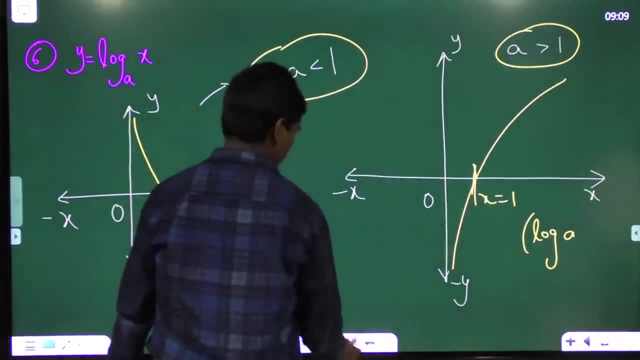 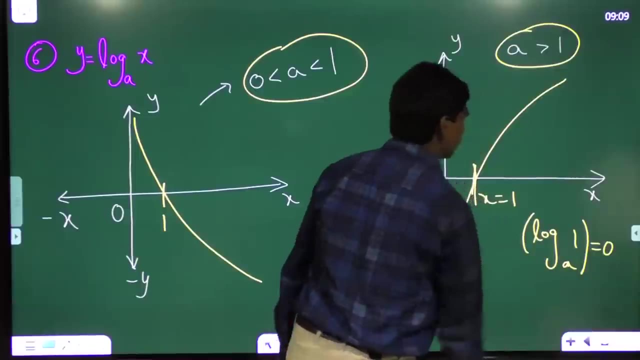 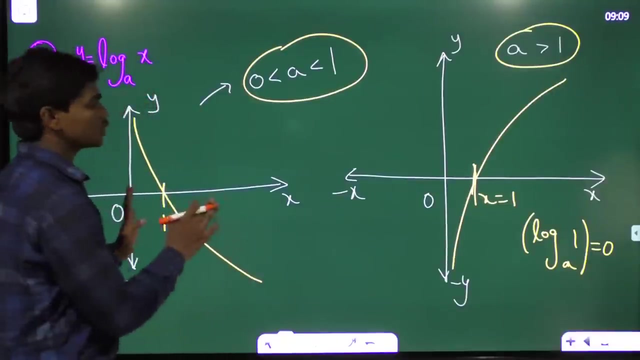 where this value is again, x is equal to 1.. And log a- I mean sorry, log x- log 1 to the base a is equal to 0.. And one thing is very clear: this base a is not equal to 1, and it's not negative as well. So log 1 to the base a is 0.. These are two different graphs based on different values of a. Okay, So in interview, if they ask you to draw the graph of log x to the base a, kindly ask them, sir, what's the value of a? Okay? 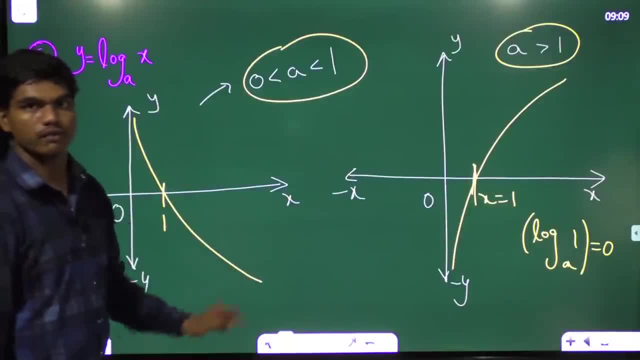 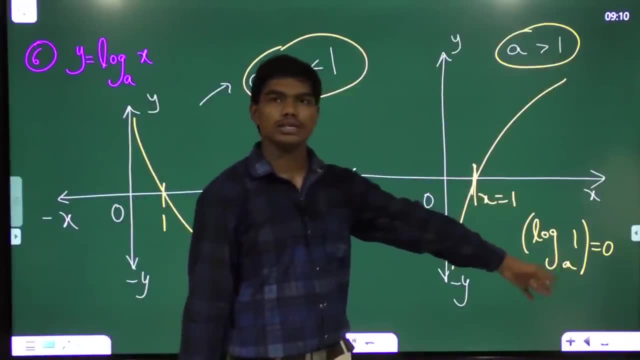 the value of a. now, depending on the value of a, you should choose one of this and, generally, if you see, if this a value is e, that you see in e, power x in that e, since the value of e is 2.7 around, will show you why the value of e is 2.71. now when i teach you. taylor says: but for the time being, 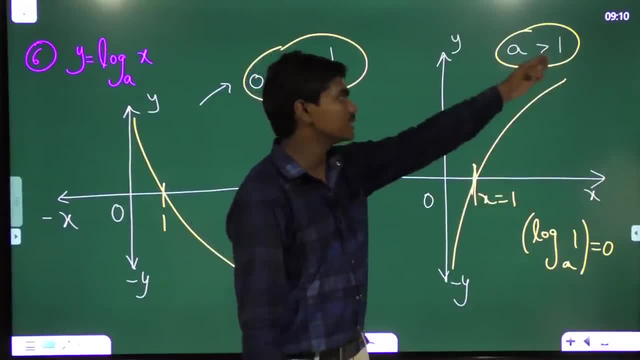 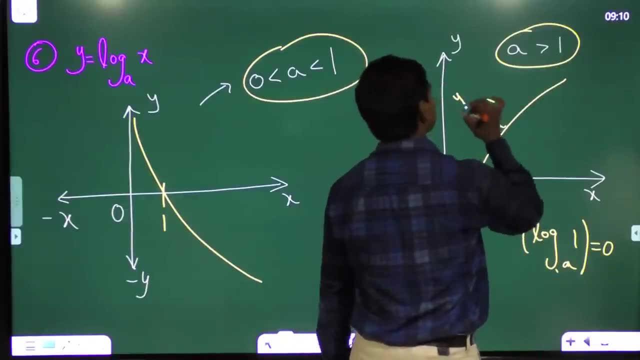 trust me. the value of e is 2.71. so since 2.71 is more than 1, log x to the base e graph will always look this way. okay, so this is. graph of y is equal to log x to the base a when a is greater than 1. 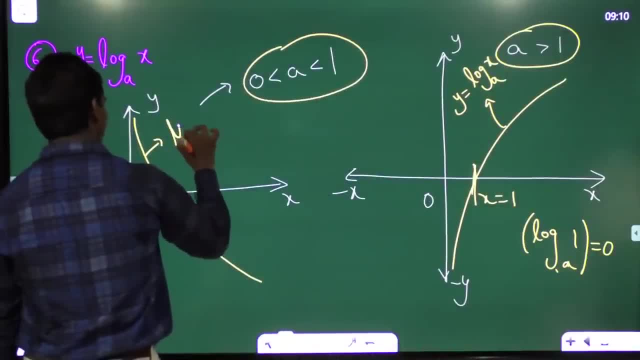 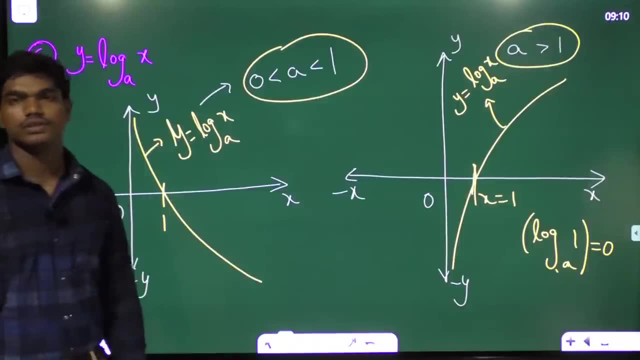 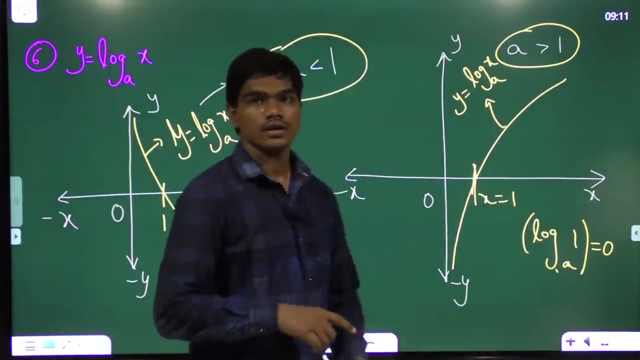 and this is y is equal. y is equal to log x to the base a when a is lying between 0 and 1. so these are the two graphs. please take care of this. you have you taken this clear? next we'll go for one function. it's also being asked in gate. 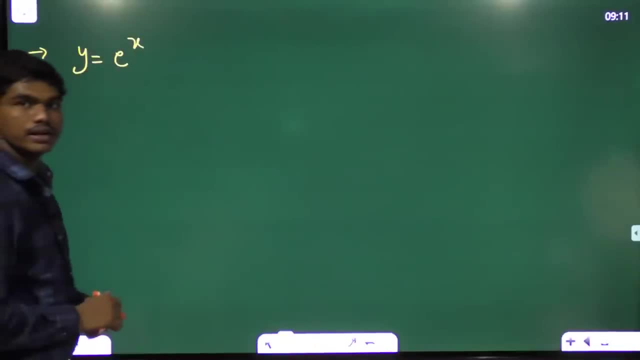 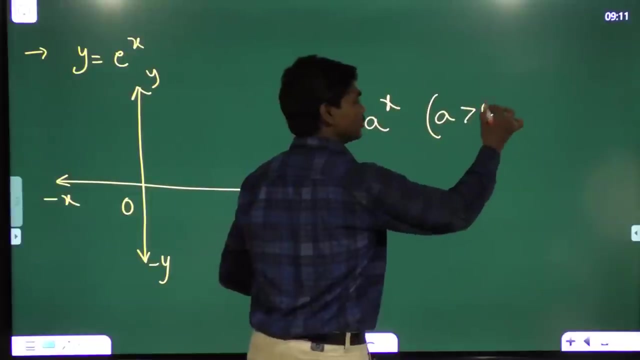 y is equal to e power x function okay. y is equal to e power x. now, if you see, this is 0 x minus x, y and minus y. now, first of all, tell me one thing: if i write a power x giving you that a is greater than 0, this number is positive. can this a power x be negative for? 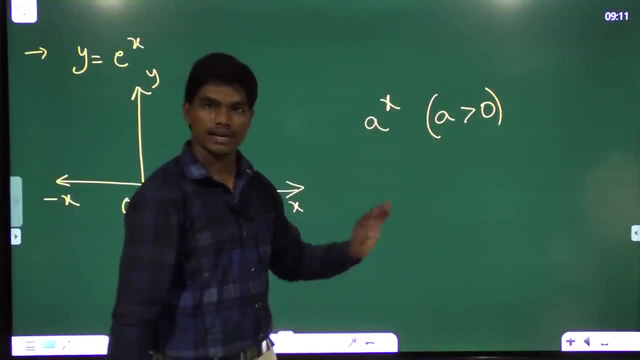 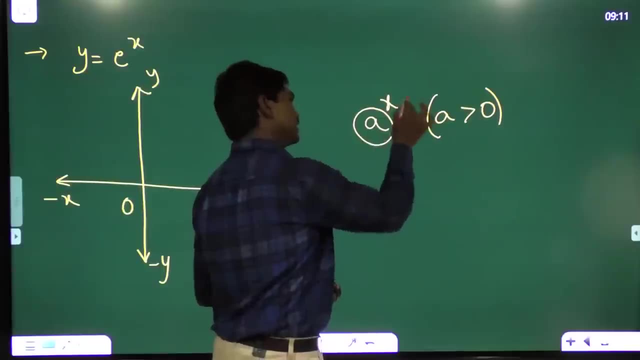 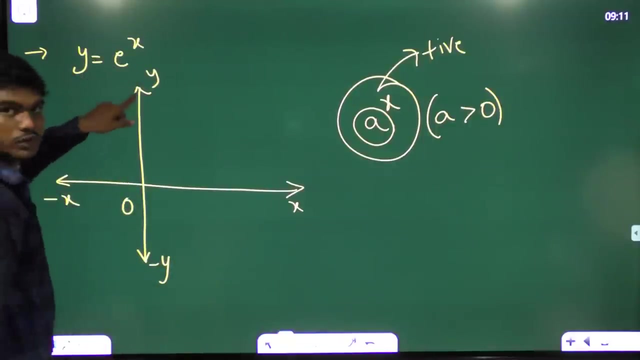 any value of x that you choose, of course, real values. can it be negative, yes or no? no, correct you so. which means, if this a is positive, this a power x is always positive. which means, when you are drawing the graph of e power x, since i have told you the value of e is 2.7, then this value, e power. 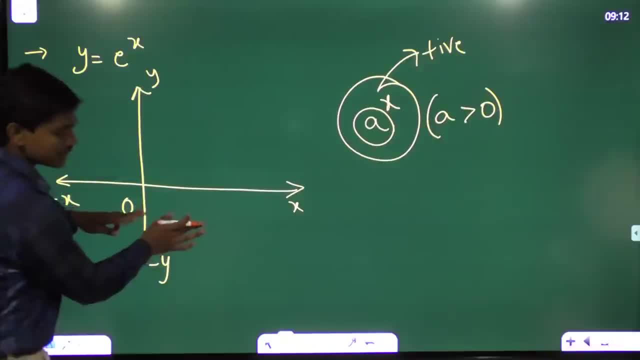 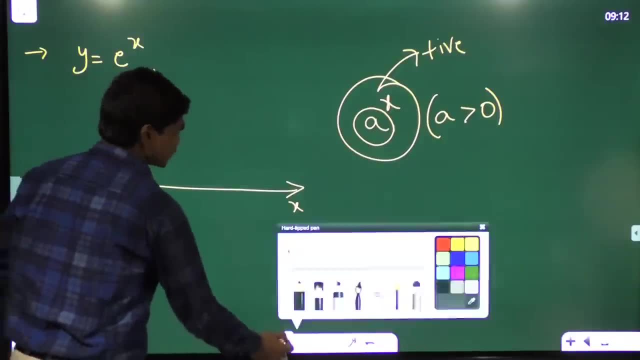 x is never negative, which means graph doesn't lie in this third and fourth coordinates. okay, graph lie only in first and second coordinates. now one thing you know well about this graph is: if you put x is equal to 0, anything to the power, 0 is negative. so if you put x is equal to 0, anything. 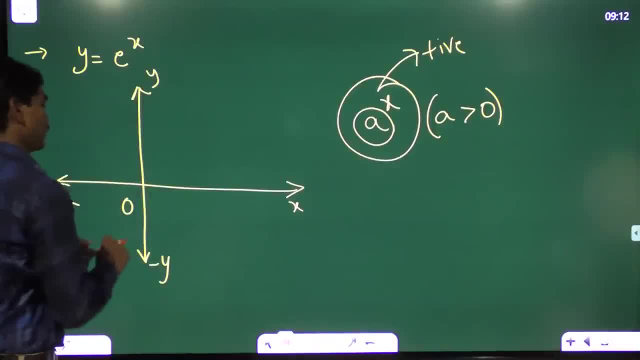 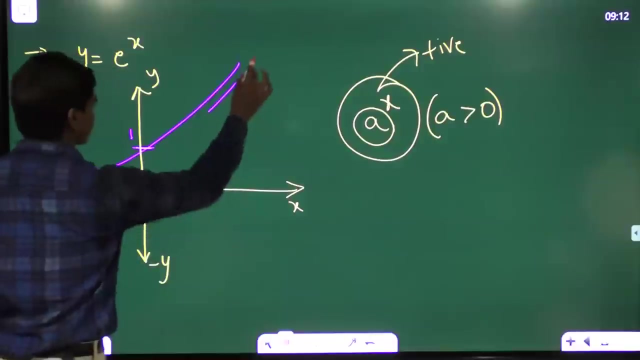 is one, of course, that anything is not 0. so e power 0 is 1, which means at x is equal to 0. you have the value of e power xs one correct. now if you similarly plot for other values, you could get a graph something like: sorry, we got a double line. actually, let me draw it again so you could. 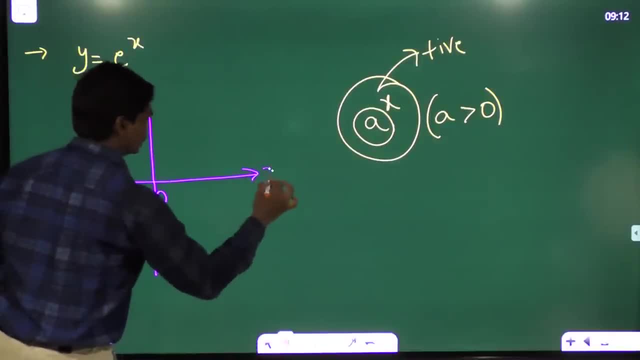 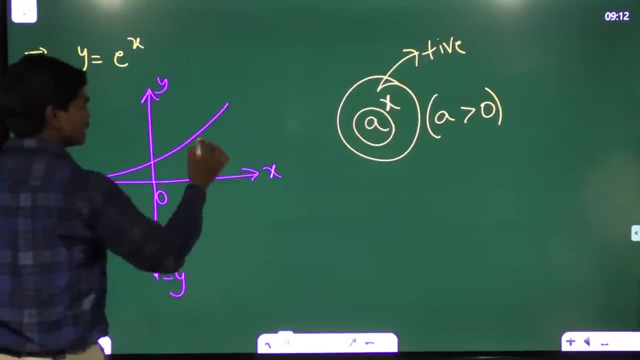 see it clearly: 0 x minus x, x, y minus y. and this is how graph of y is equal to e power. x looks like and this value is 1, since at x is equal to 0, e power 0 is 1.. Now, with the help of this knowledge, can you draw a graph for y is equal to e power minus. 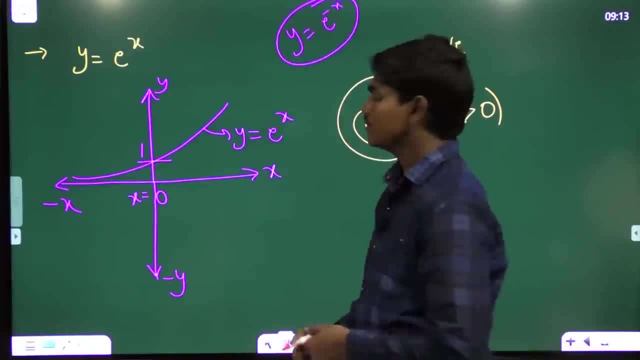 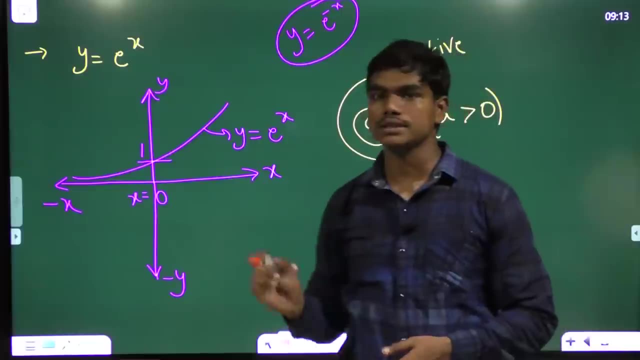 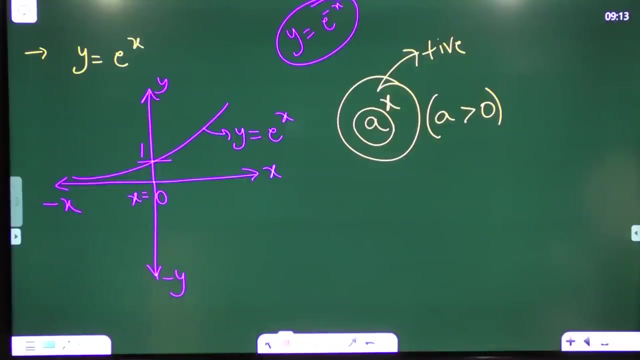 x. Please try to draw. Tell me how does it look like This is: y is equal to e power x graph. Now try to draw the graph for y is equal to e power minus x. Please try to draw the graph for y is equal to e power minus x graph. 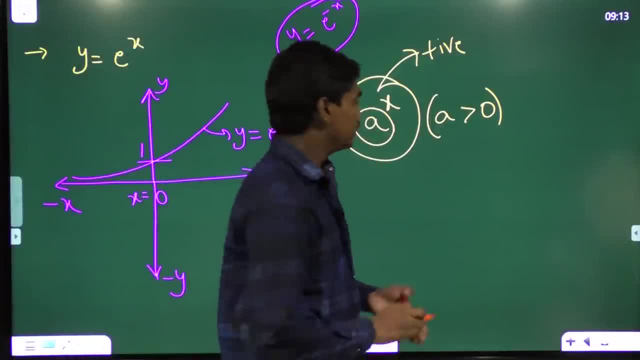 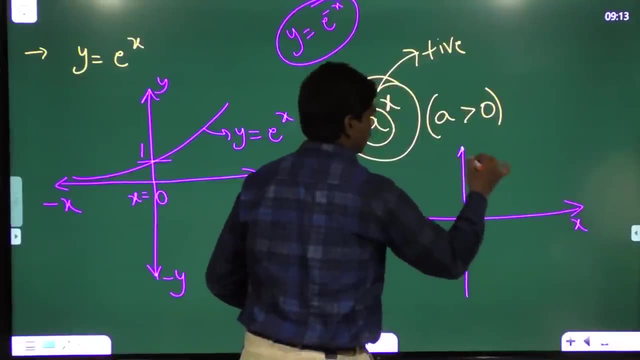 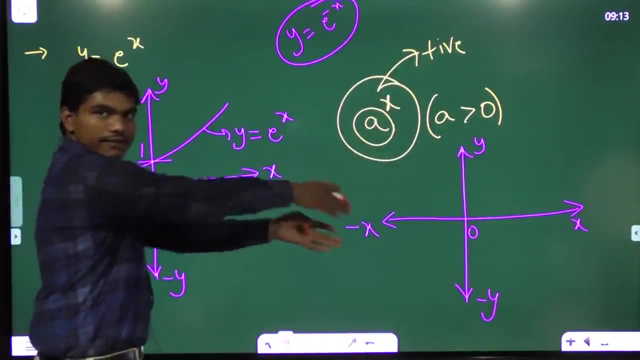 Okay, clear. So this is: y is equal to e power x. So y is equal to e power minus x. I am giving it here itself again. Okay Now, whatever the values you got for positive values of x, you will get for negative in. 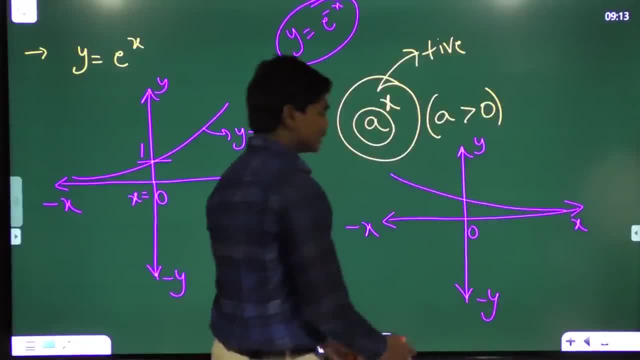 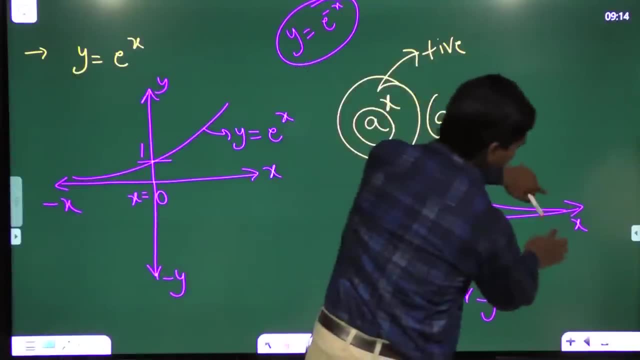 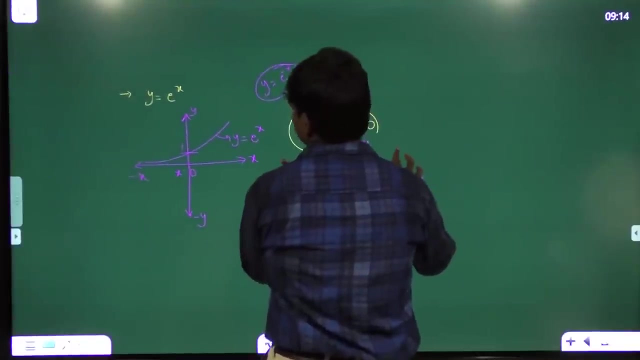 this graph. So graph looks something like this and if you see, clearly I am not touching these lines because we can't put infinity here. If you see, I still maintain some difference here which you could see in broad scale. These two lines didn't meet each other, okay. 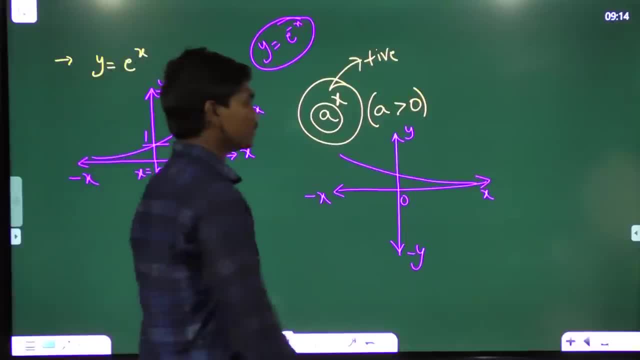 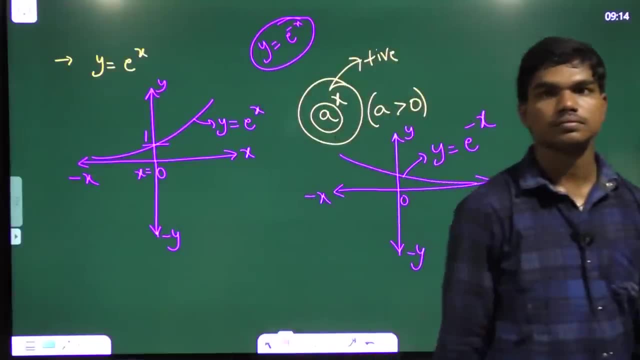 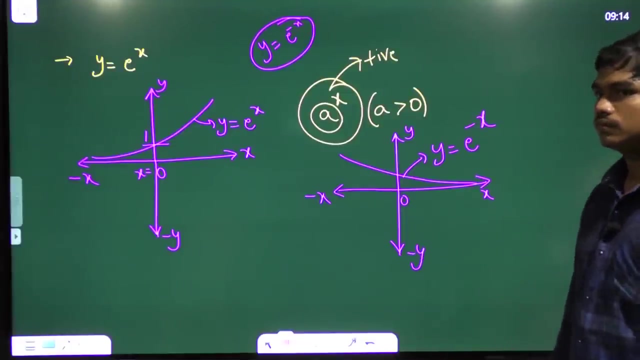 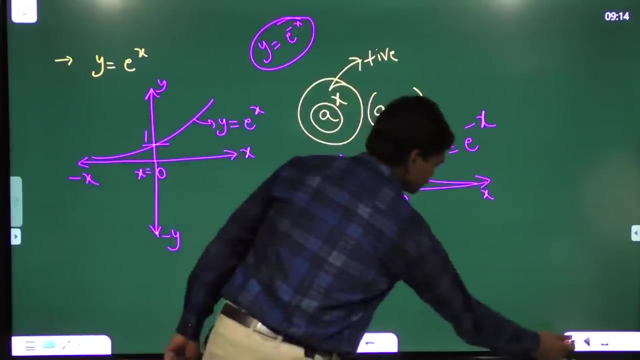 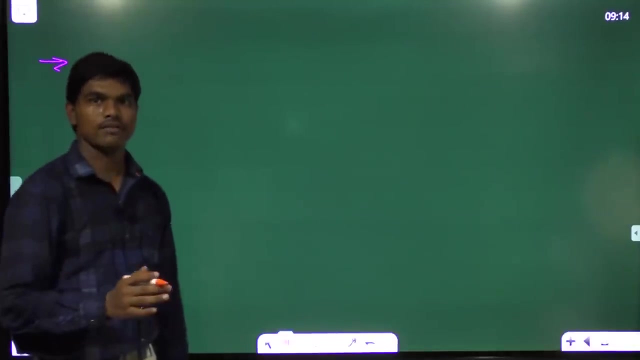 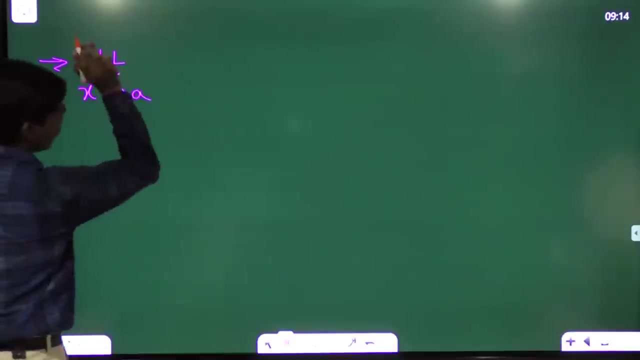 Okay, Take it Okay. So this is: y is equal to e power minus x looks like: Okay, Clear. Now let me ask you one thing. I told you what is an integer part function? Okay, Let me ask us a question which is very often asked in gate limit extends to a limit extends. 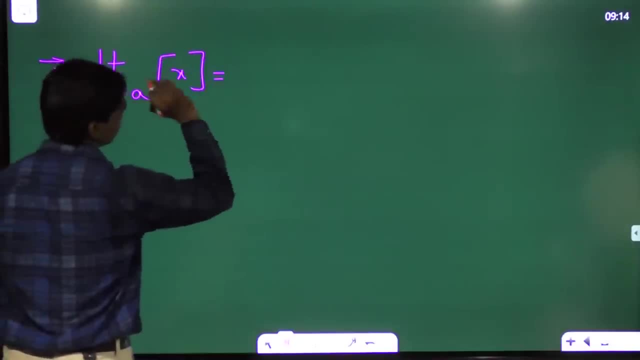 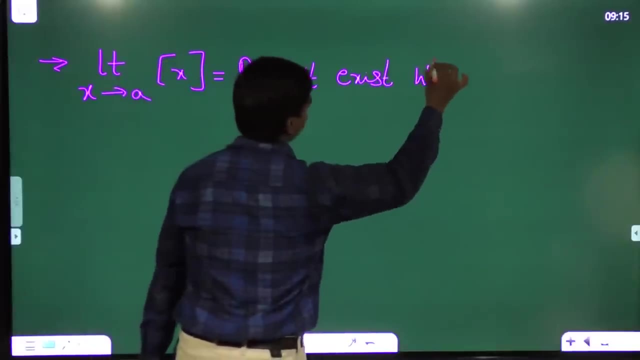 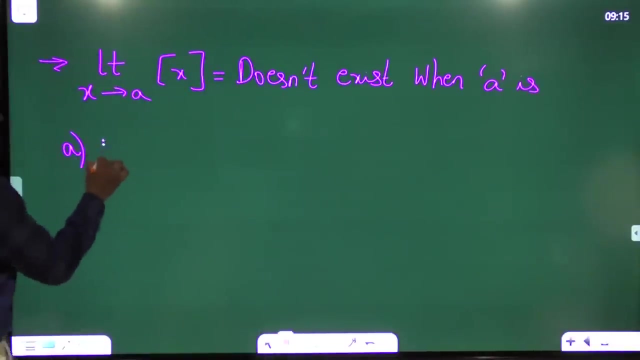 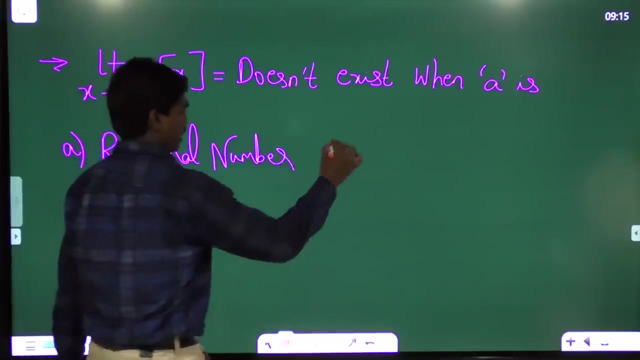 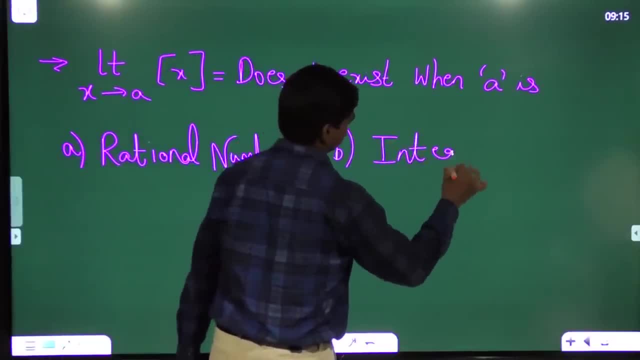 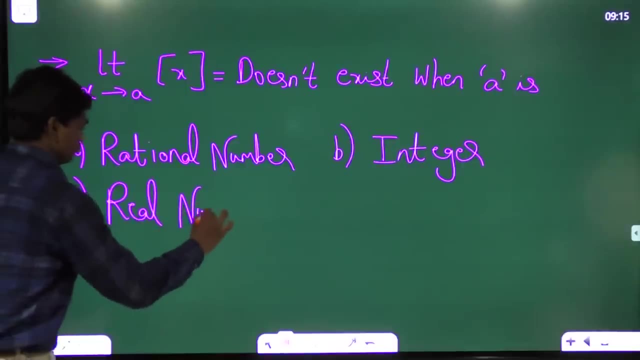 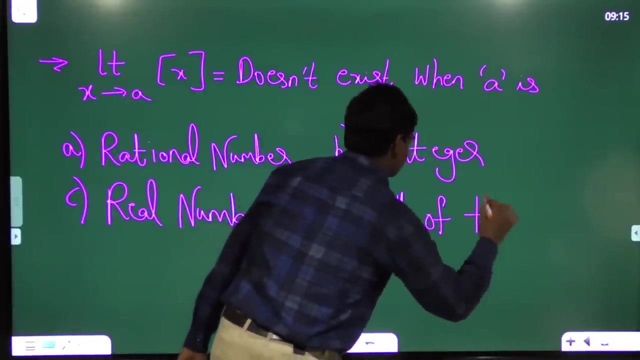 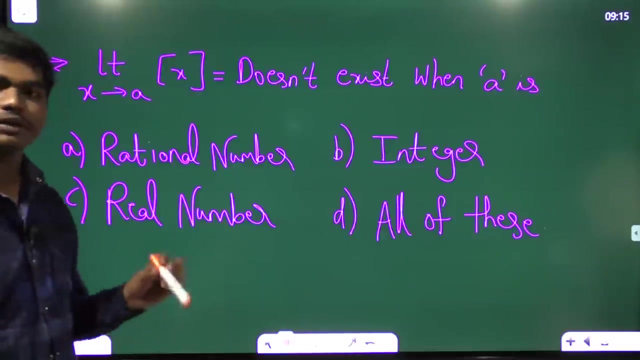 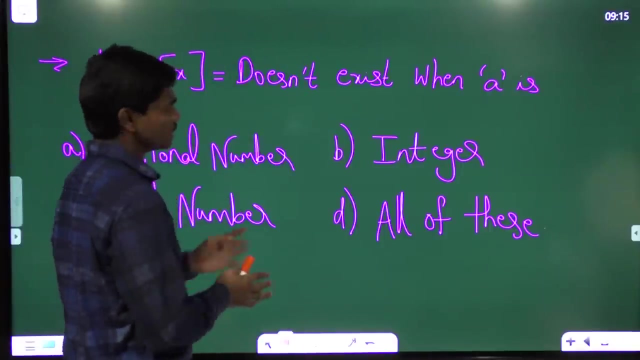 This is the question. You could pause the video for a moment and you could think what is the answer. I am giving you time for a minute. Please do that. I am telling you: limit extends to a integer. part x does not exist when a is. 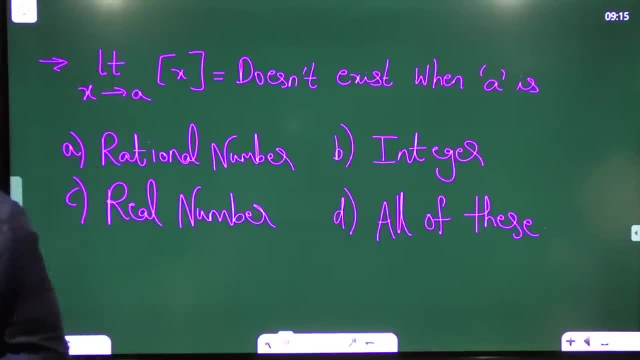 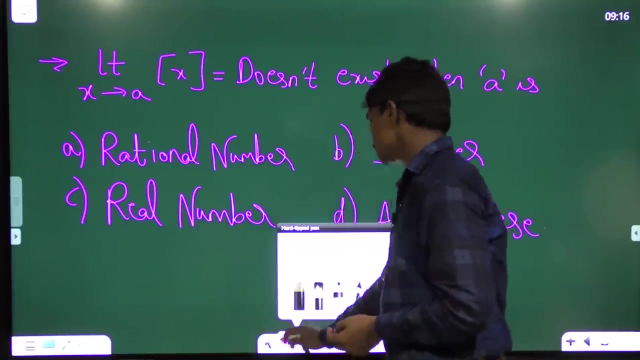 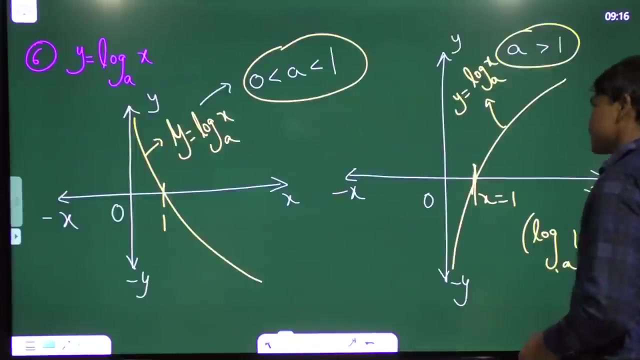 Okay, Please take this and try to answer this. The answer is a. The answer, Well, let me tell you, The correct answer for this is integer, Because if you see the graph of integer, part x that I showed you moments later, 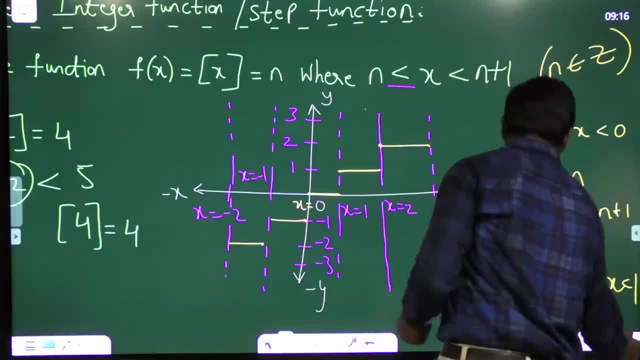 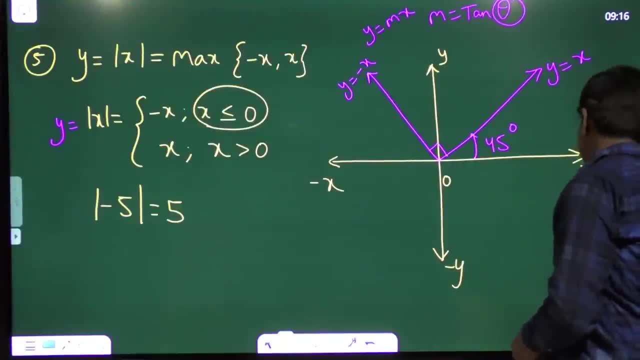 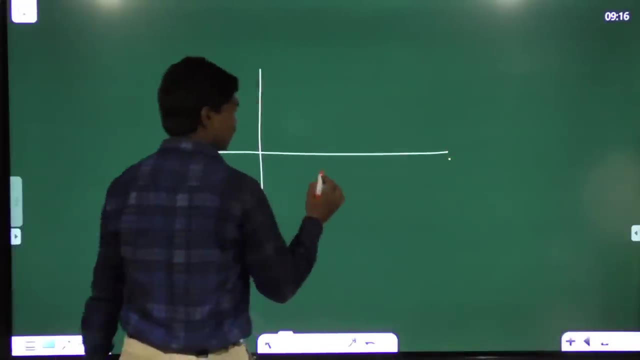 This one. Now, this is the graph that I am showing you for the basic idea, to recount what we have learned. Now why, for integers, this graph does not exist. See here: Let us suppose This is x axis, This is minus x, 0, y and minus y. 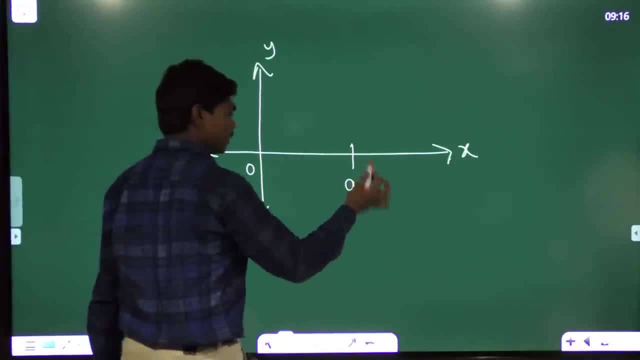 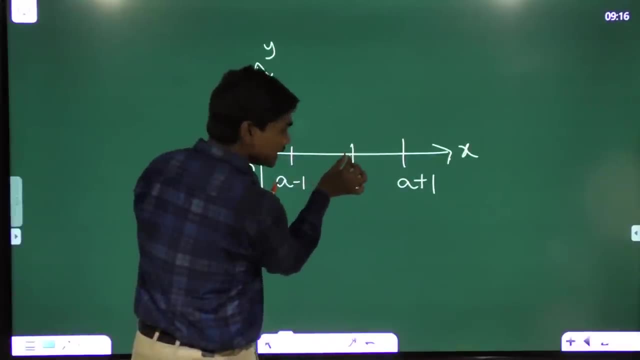 Okay, Now let this value. here is a, Then this is a minus 1 and this is a plus 1.. And, of course, a minus is somewhere near to this here and a plus is also somewhere near to this at that point. 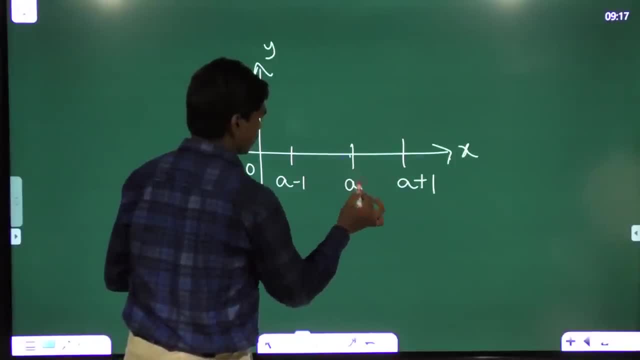 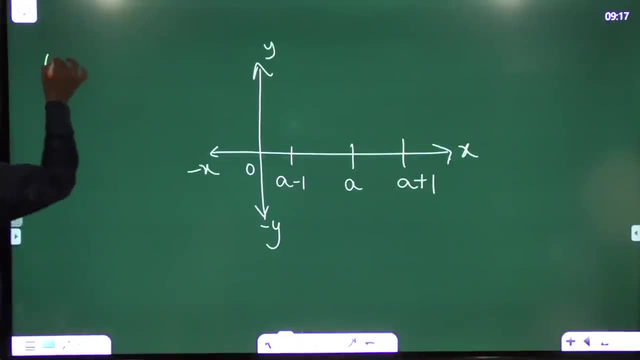 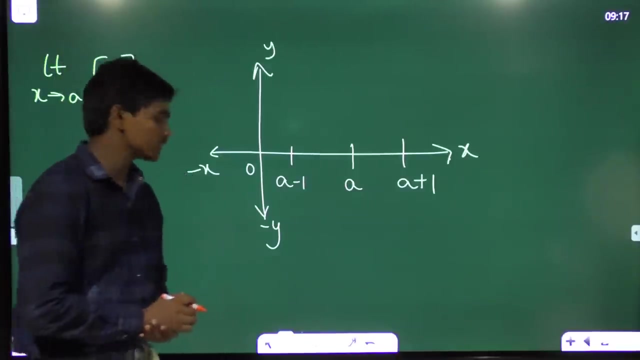 Let me make it clear: Okay, So this is a and this is a plus 1.. Now, if I want to evaluate this limit- x tends to a integer part of x- we should consider both left-hand limit as well as a right-hand limit. 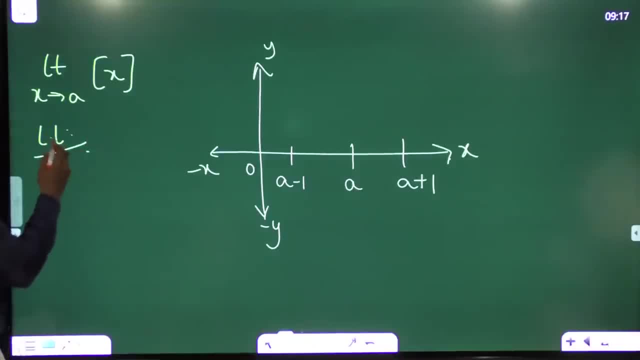 So left-hand limit, if I am considering l stands for left-hand limit, So limit x tends to a minus. integer part x. This is what I need to evaluate. It means, when x is tending to this a minus, what does this integer part x function goes? 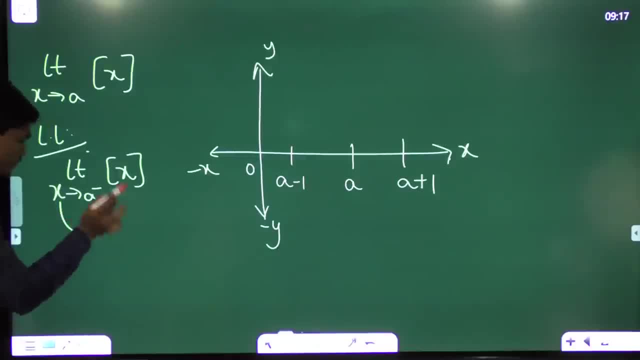 to Now see clearly: When I say x is tending to a minus, this implies x is less than a or more than a. Tell me, I told you this. a minus corresponds to left-neighborhood. So when x is in the left-neighborhood of a, x is less than a or it is more than a. 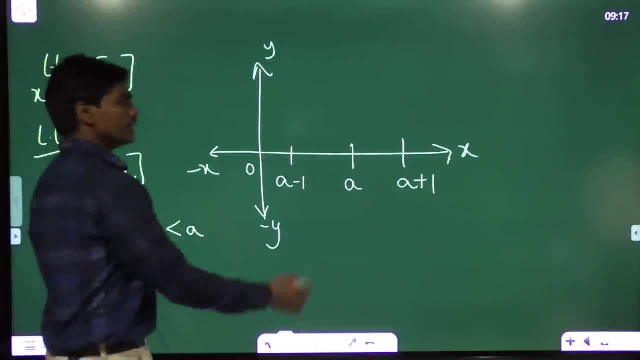 It is less than a. When x is less than a, x is lying somewhere here. Let me use a different color So you could see x is tending somewhere here and now. here, x is lying in between two consecutive integers, which are a minus 1 and a. 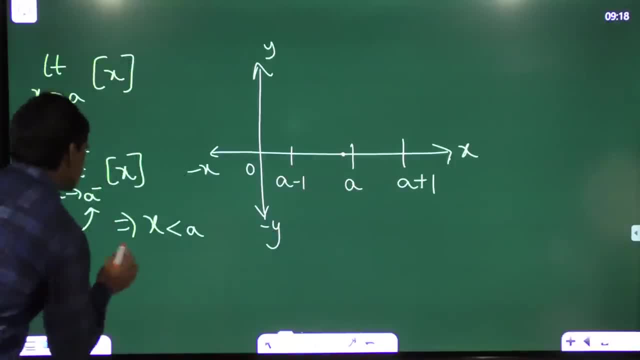 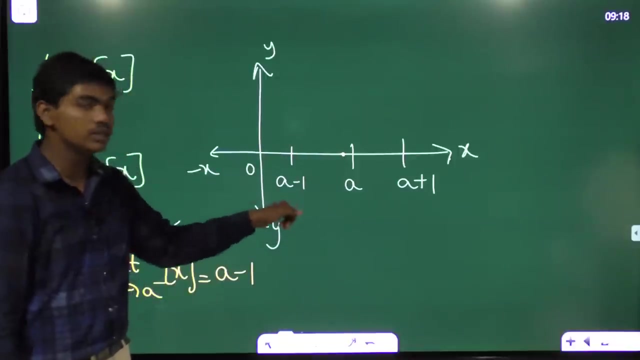 Okay, So, which means this implies limit x tends to a minus. integer part x is equal to a minus 1, since x is lying in between a minus 1 and a. And I told you, when x is lying in between n and n plus 1, integer part x value is n. 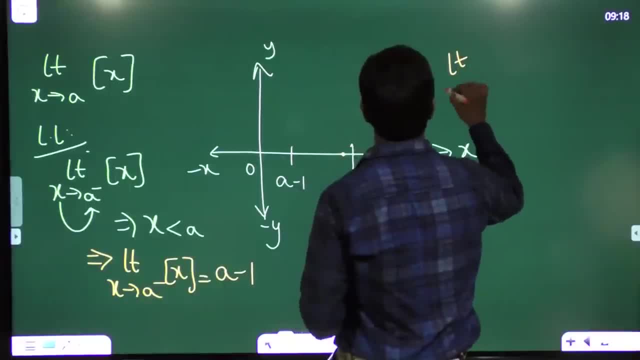 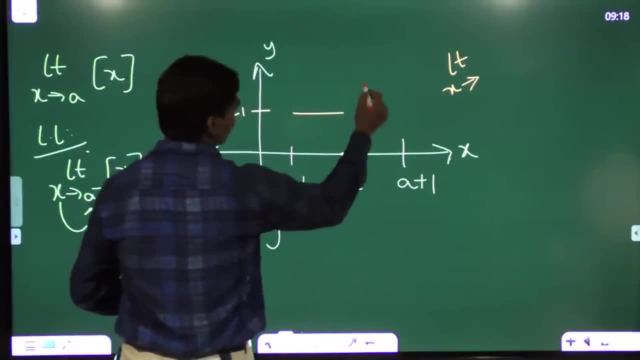 Okay Now, if you talk about right-hand limit, let me draw the graph also for these two. For a plus 1 to a, the value will be a minus 1.. For a plus 1 to a, the value will be somewhere here.